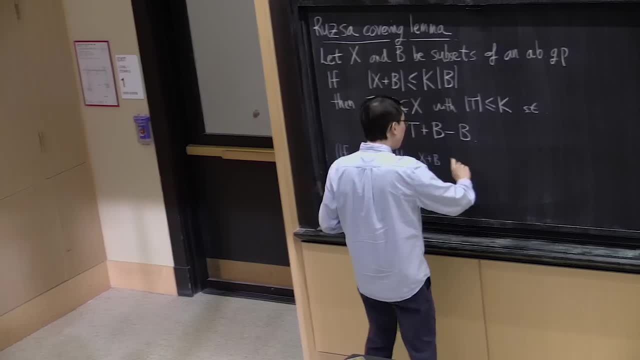 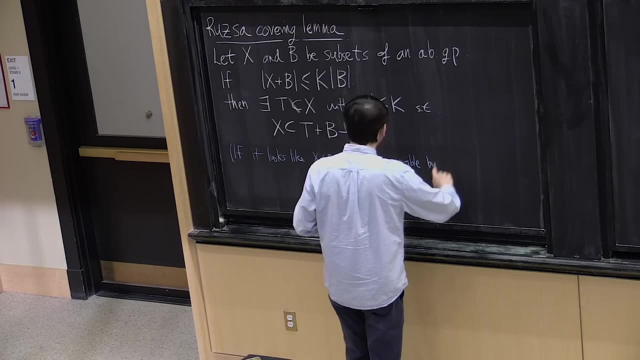 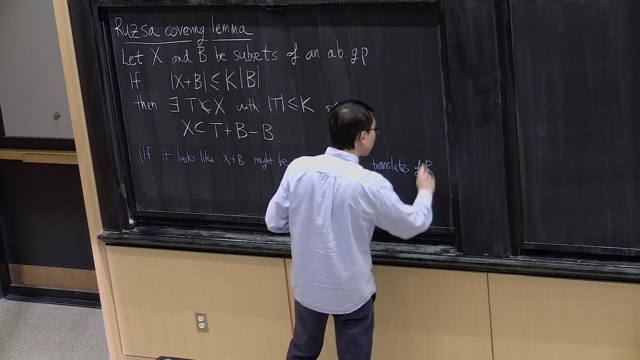 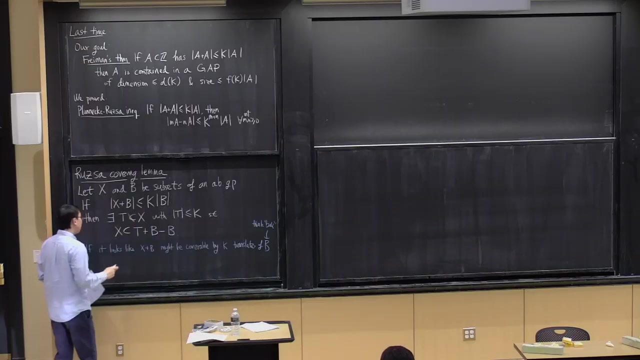 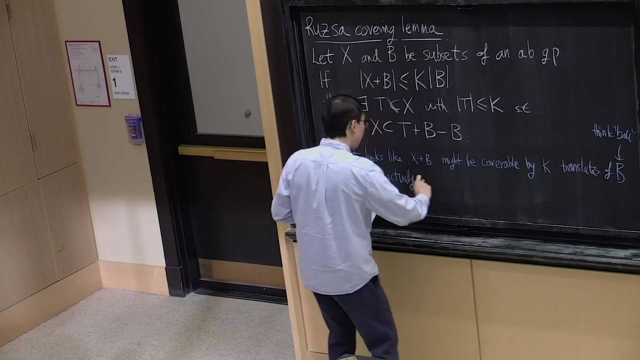 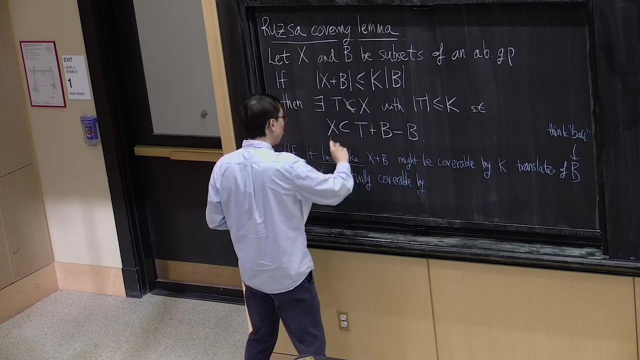 So if it looks like x plus b might be coverable by k translates- So here you're supposed to think of b like a ball in the metric space- Then x is actually coverable. So if it looks like meaning just by size alone, by size info. 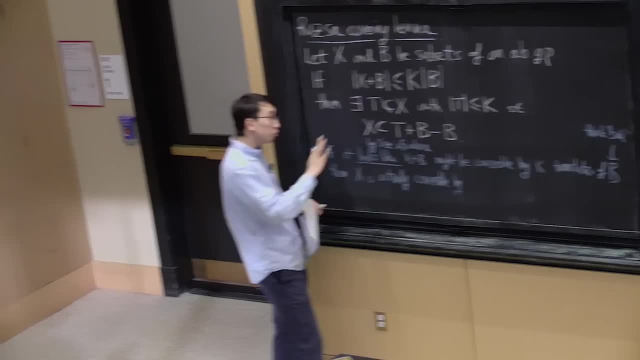 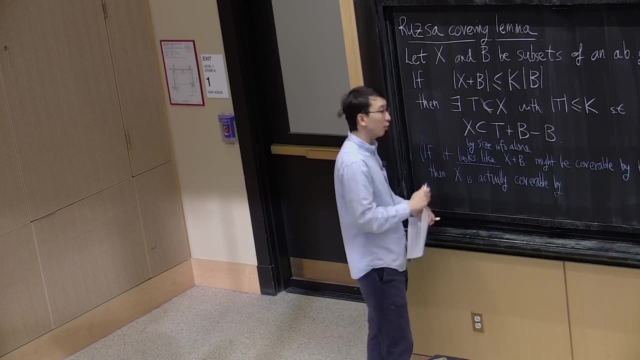 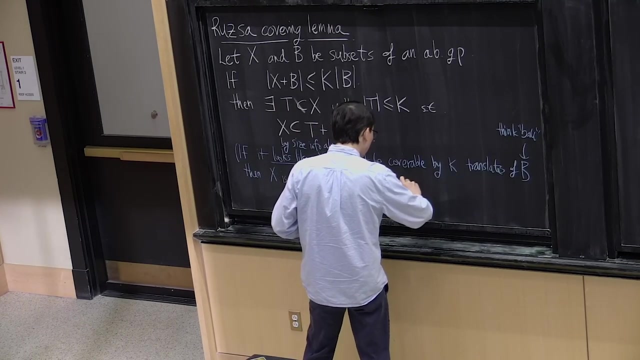 alone, OK. OK, So just based on the size, if it looks like x plus b might be coverable by k different translates of b, then actually x is coverable, But you have to use slightly larger balls by k copies of b minus b. 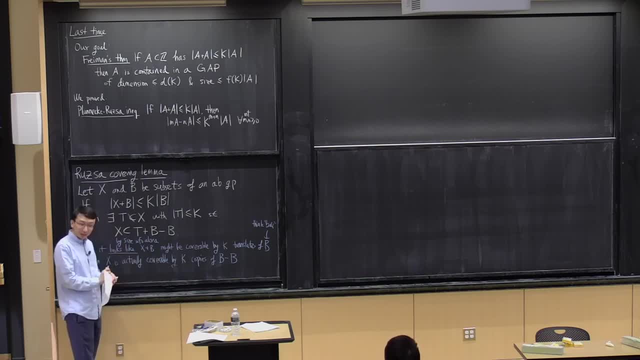 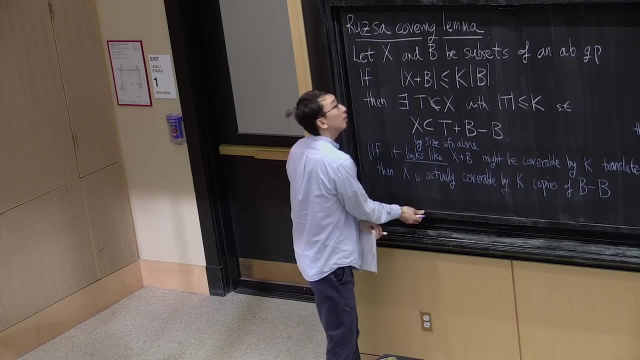 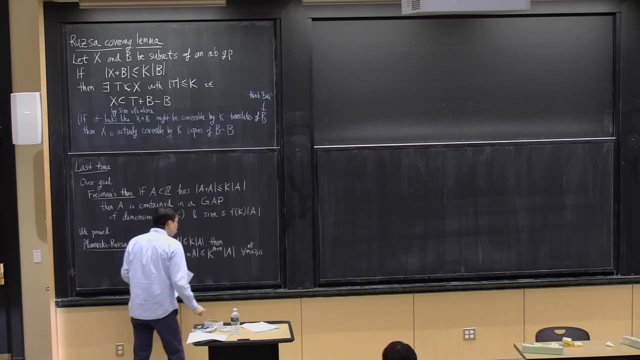 So you should think of b minus b as slightly larger balls than b itself. So if b were an actual ball in Euclidean space, then b minus b is the same ball with twice the radius. So Rousseau covering lemma is a really important tool. 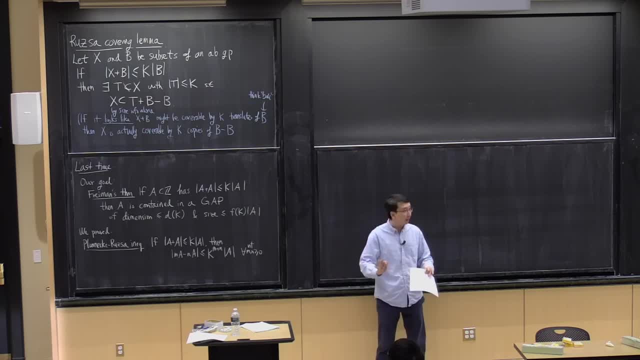 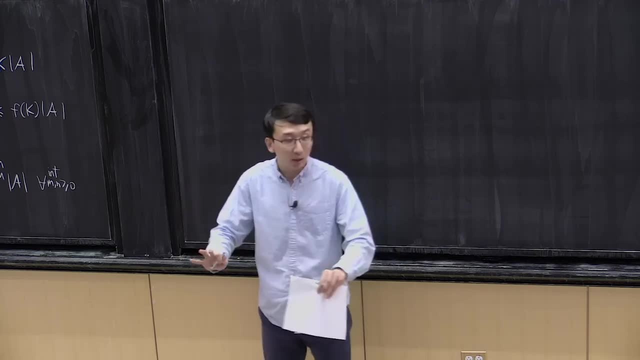 The proof is not very long And it's important to understand the idea of this proof. So this is a proof, not just in additive combinatorics, but something that happens. It's a standard idea in analysis, So it's very important to understand this idea. 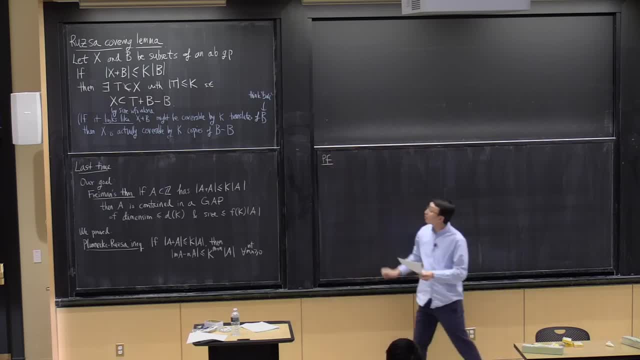 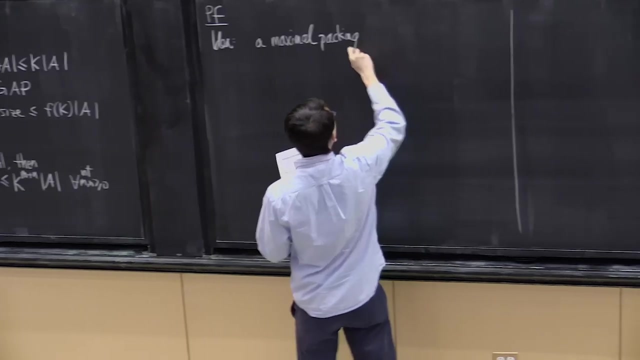 And the key idea, But here I think the proof is more important than the statement up there. The key idea here is that if you want to produce a covering, one way to produce a covering is to take a maximal packing, a maximal packing using with. 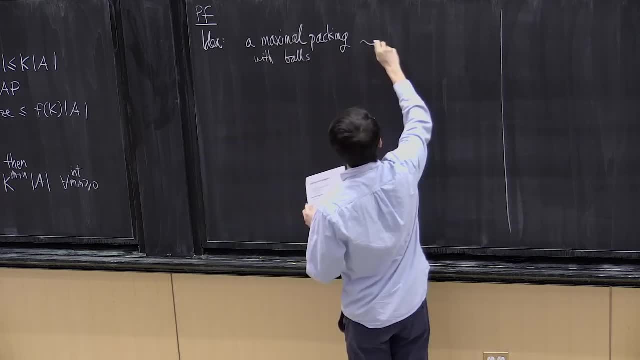 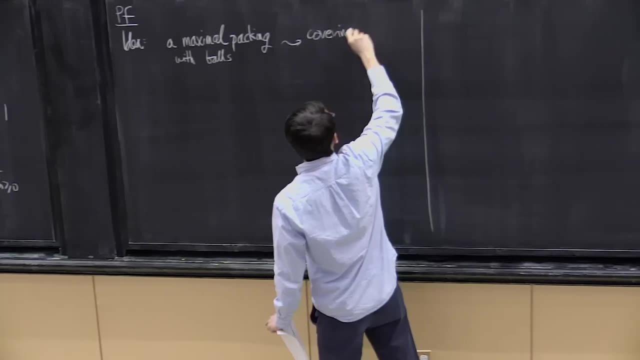 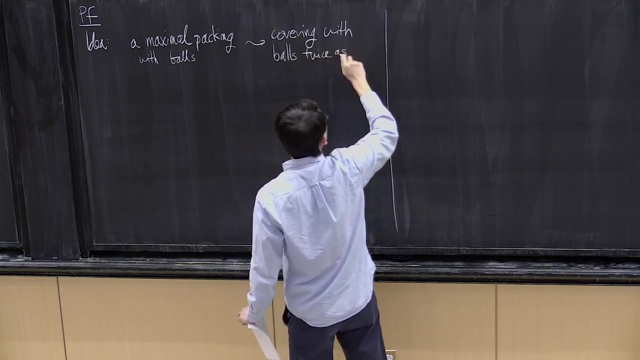 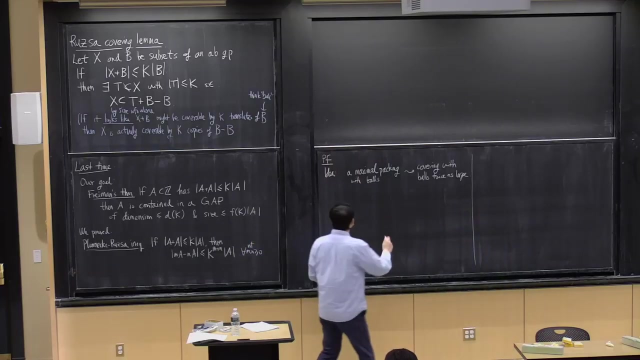 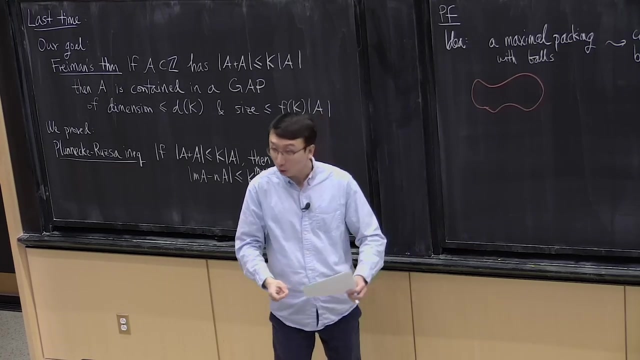 OK, So let's say unit balls, for instance, implies a covering with balls twice as large. So let me illustrate that with the picture. Suppose you have some space that I want to cover, But you get to use, let's say, unit balls. 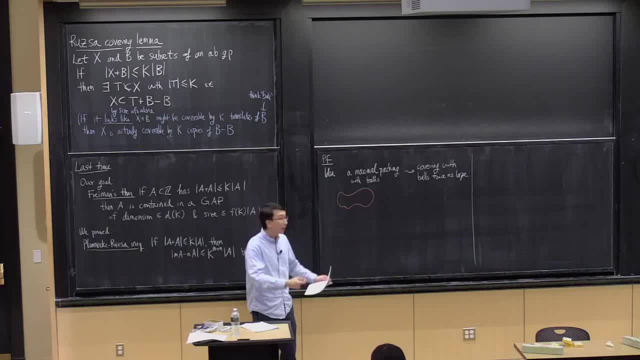 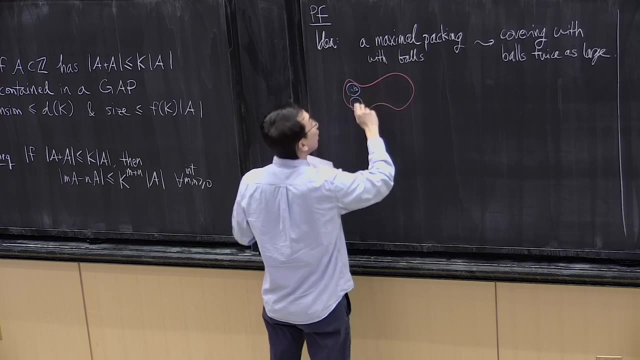 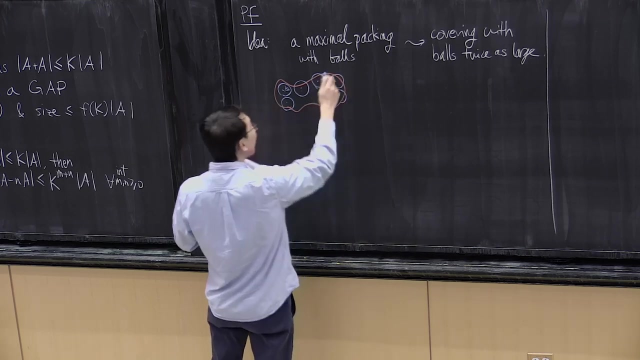 So how can I make sure I can cover the space using unit balls, And I don't want to use too many unit balls. So what you can do is let me start by a maximal set of unit balls, So with centers, so it's now half unit balls. 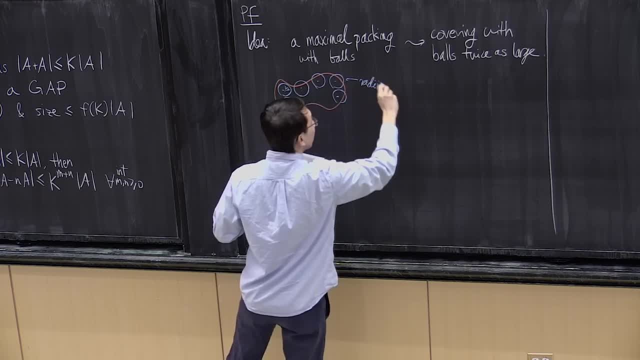 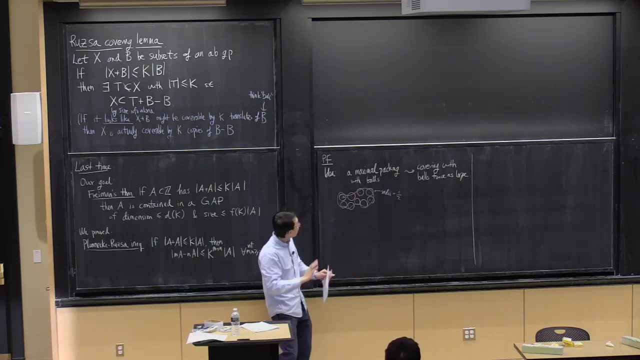 So the radius is 1 half. So I put in as many as I can, so that I cannot put in any more. So that's what maximal means. Mo here doesn't mean the maximum number, although if you put in the maximum number, that's also OK. 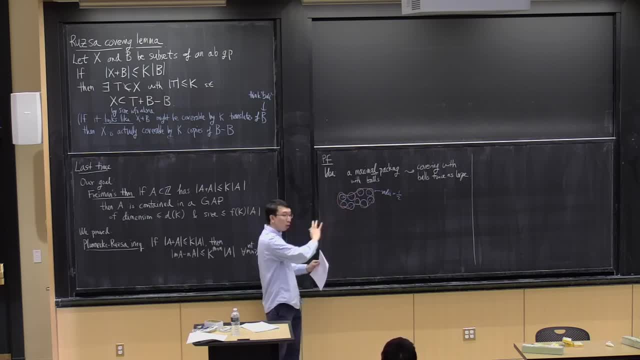 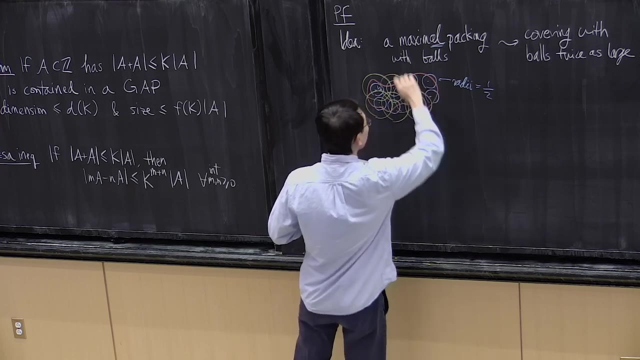 But maximal means that I just cannot put in any more balls that are not overlapping. Then if I have this configuration now, what I do is I double the radii of all the balls. So whoever takes today's notes will have a fun time drawing this picture. 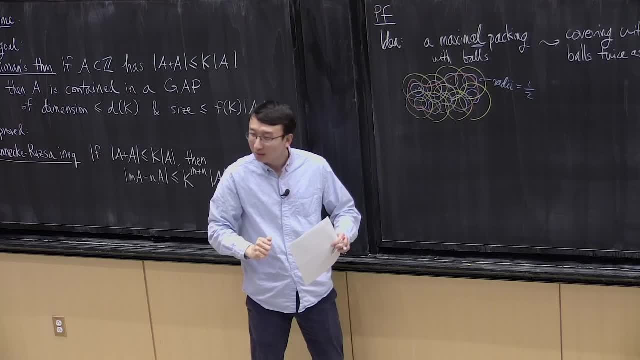 So this has to be a covering of the original space, Because if you had missed some point, I could have put a blue ball in. Yes, What if the space has some like narrow portion? YUFEI ZHAO-. What if the space? 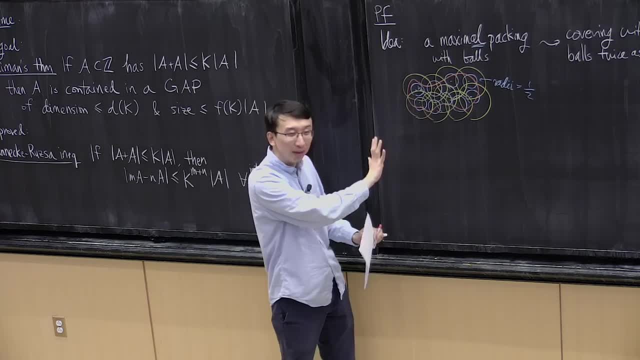 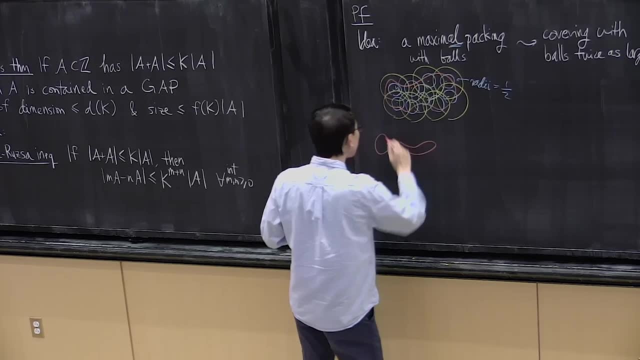 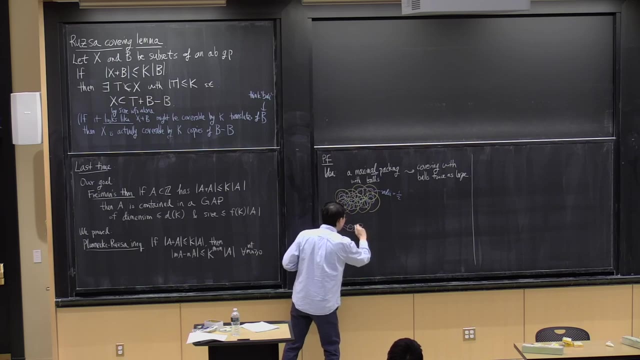 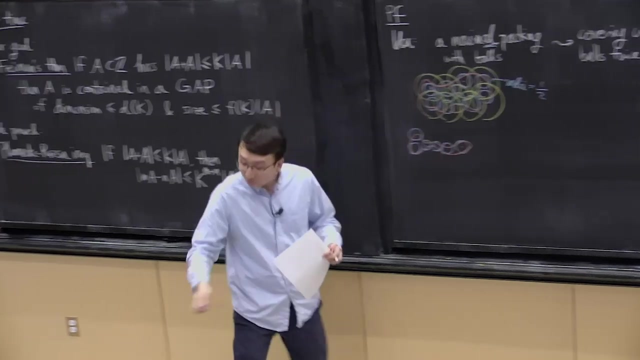 has some narrow portion. It doesn't matter If you formulate this correctly, if you miss some point, So here. so it depends on how you formulate this covering. So the point is that if you take a maximal set of points, when you expand, you have to cover the whole space. 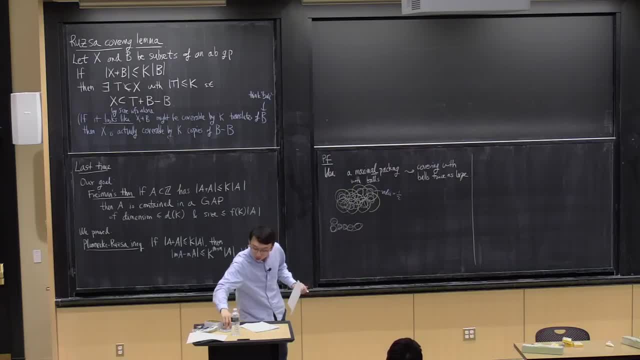 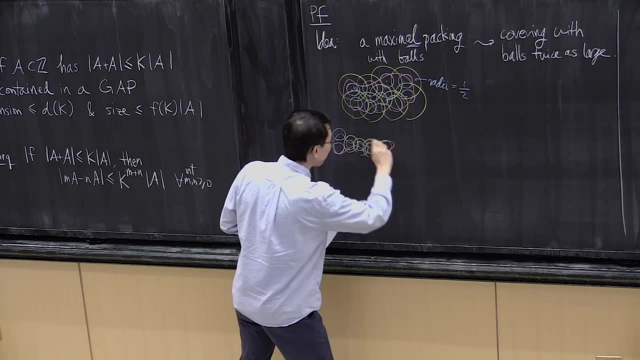 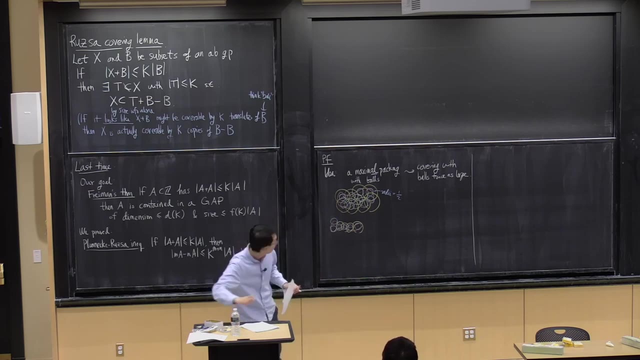 Because if you missed some point, so imagine if you had, for example, if suppose you missed, well, OK, I mean suppose you had missed some point over here, then I could have put an extra ball in. So if you had missed some point over here, 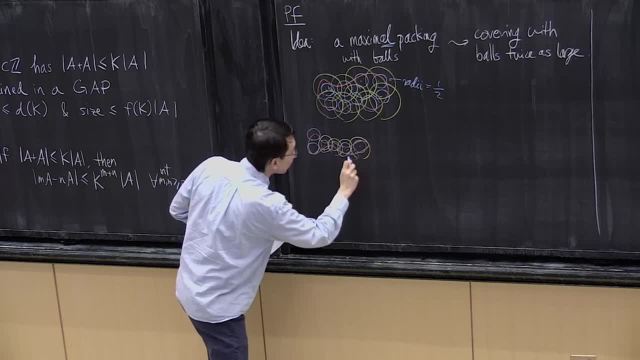 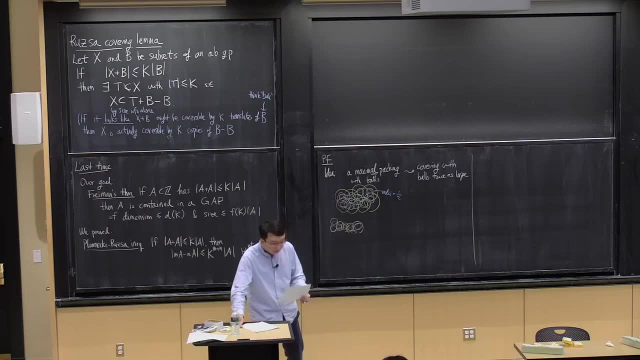 then it means that I should have been able to put in that ball there initially. So this is a very simple idea but a very powerful idea, And it comes up all the time in analysis and geometry and it also comes up here. So let's do the actual proof. 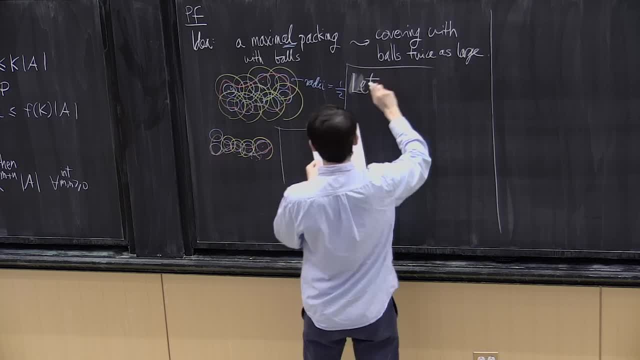 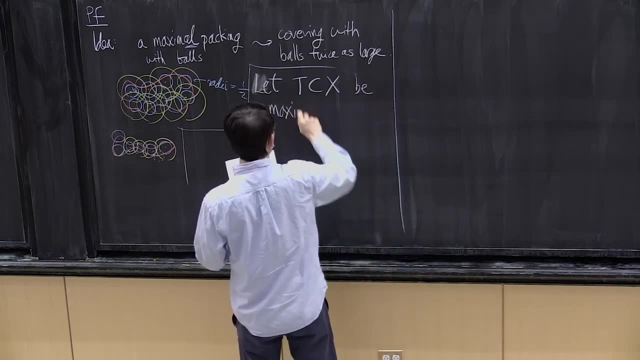 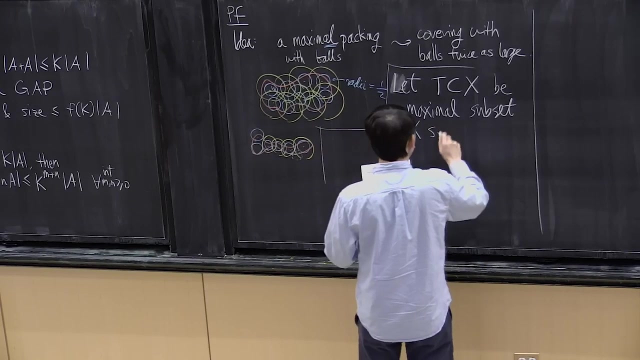 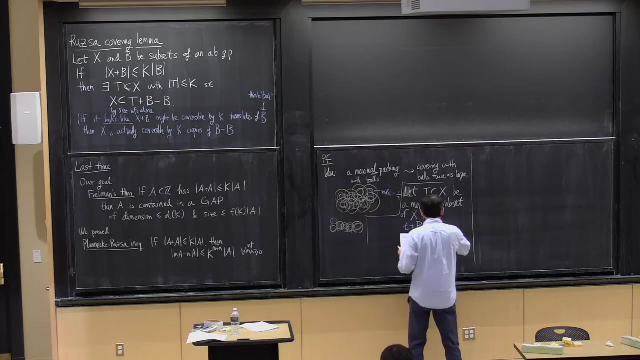 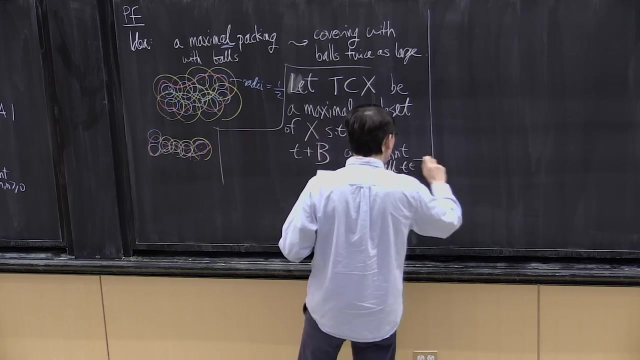 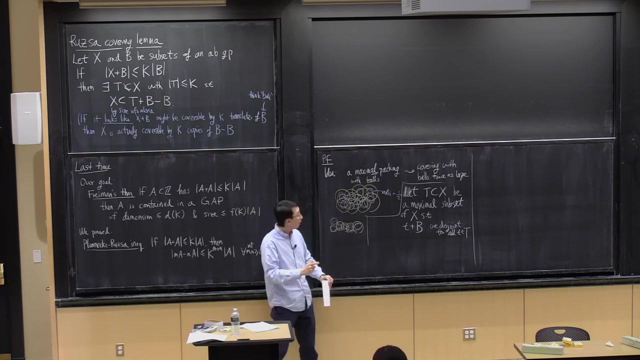 So let me let T be a subset of X, be a maximal subset of X, such that the sets little t plus b are disjoint for all elements: little t of the set, big T. So it's like this picture: I pick a subset of X so that if I center balls around these T's 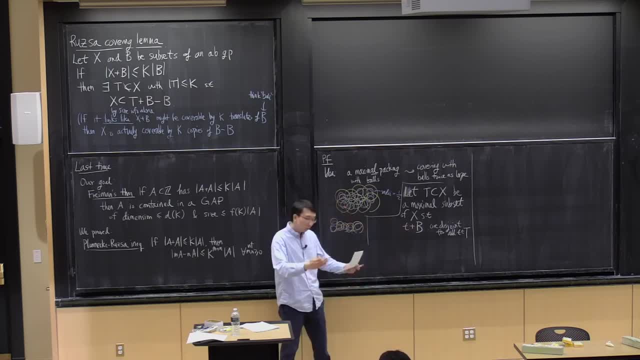 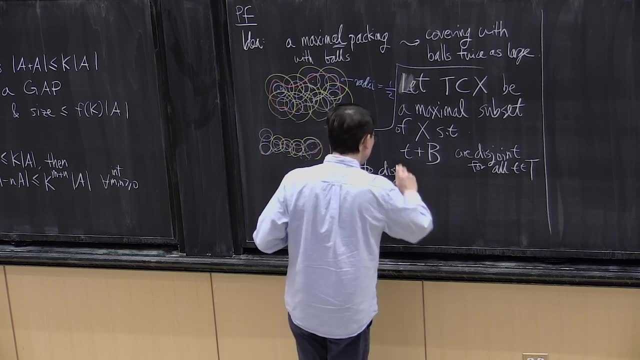 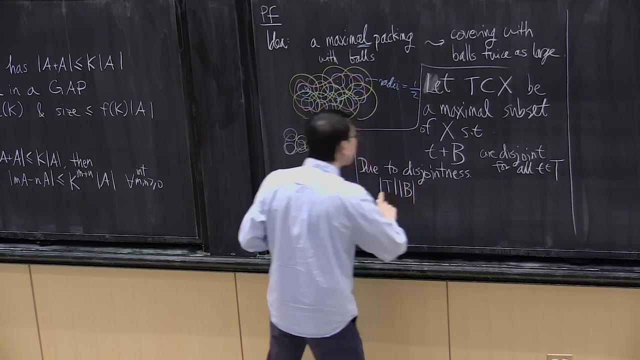 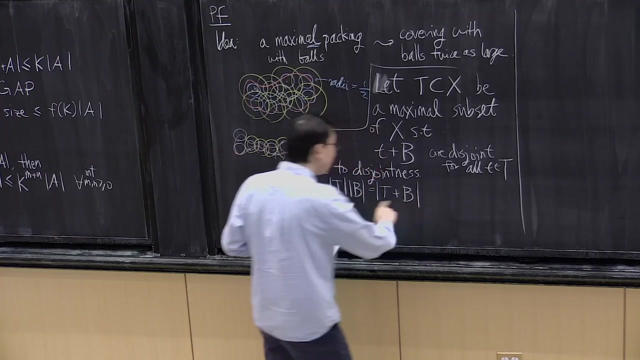 then these translates of b's are disjoint. Then you're putting a maximal set. There's no such set. So due to the disjointness, we find that the product of the sizes of T and b equals to the size of the sum, because there's no overlaps. 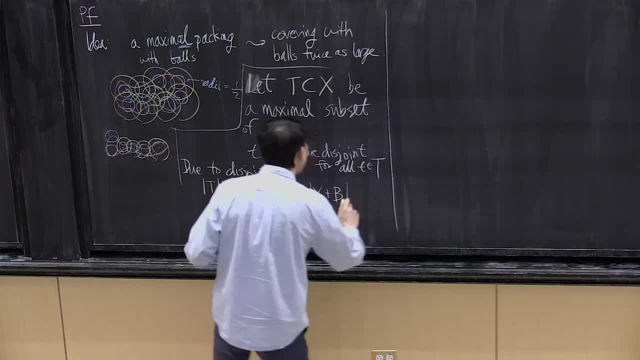 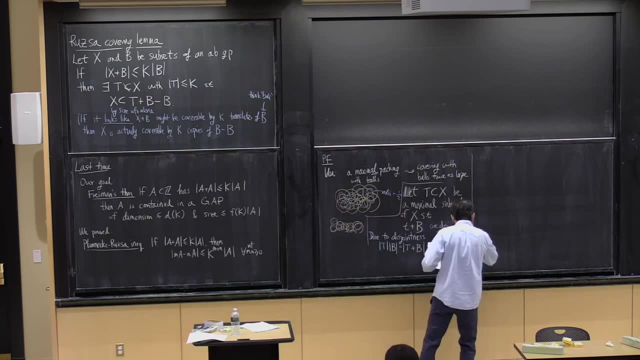 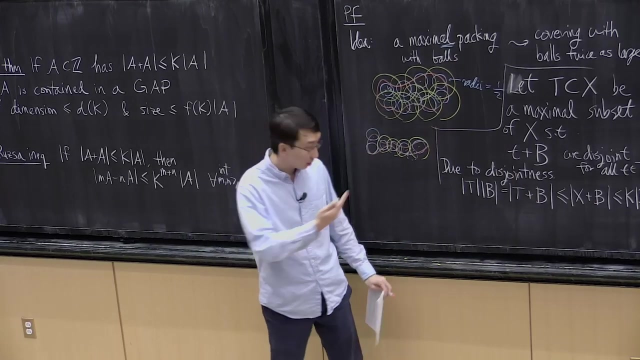 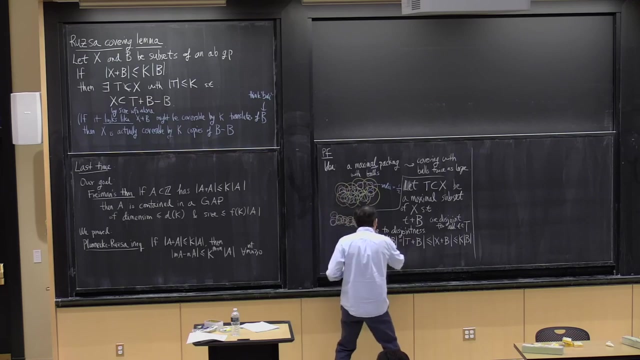 But T plus b has size at most X plus b Because T is a subset of X. But I also, from the assumption we knew, that X is size of X plus b is upper bounded by the size of b times K. So in particular we get that the size of T is at most K. 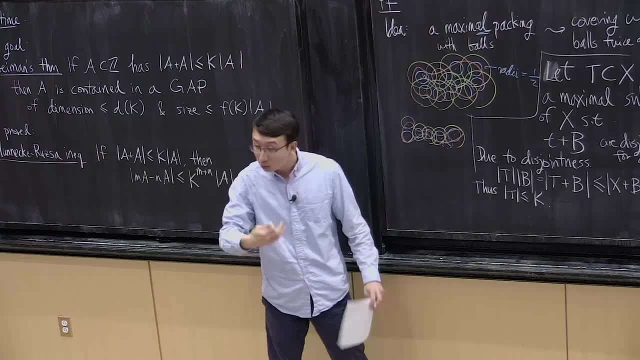 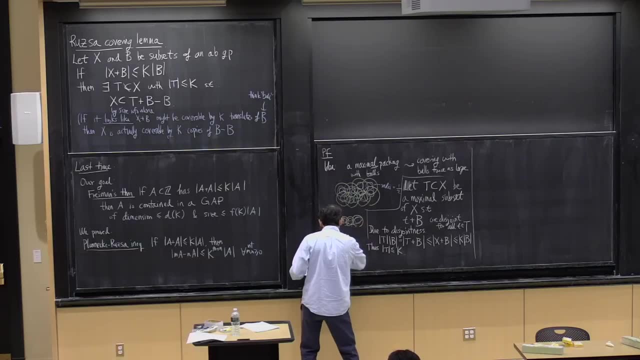 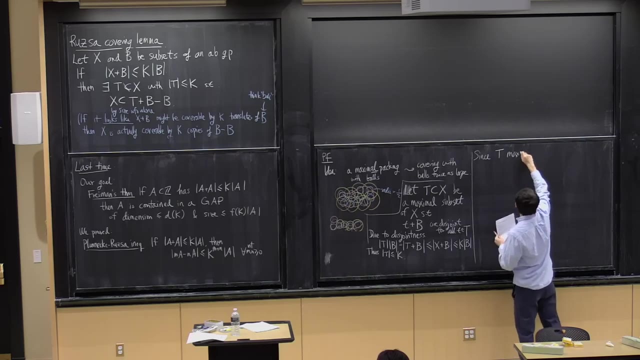 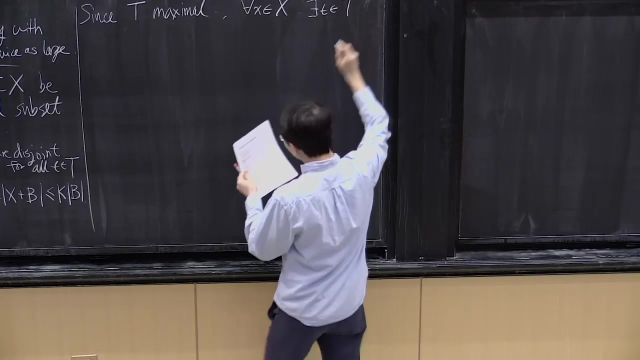 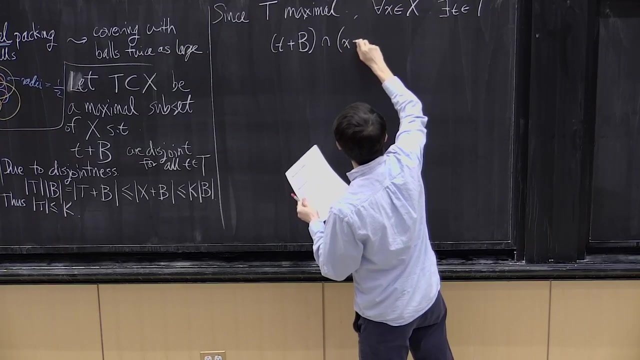 So in other words, over here, the number of blue balls you can control by simply the volume. OK, so since T is maximal, we have that for every little x there exists some little t, Such that the translate of b given by x intersects. 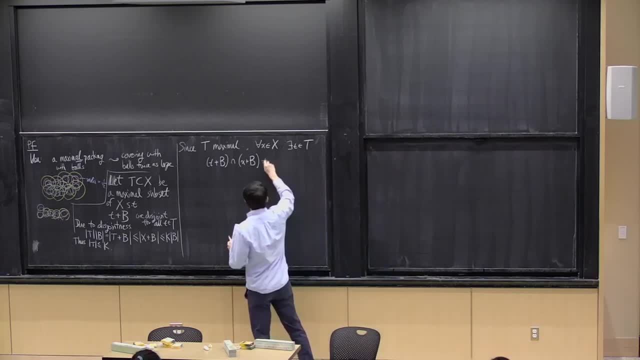 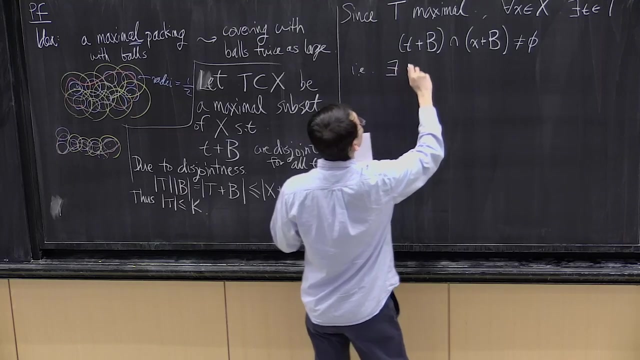 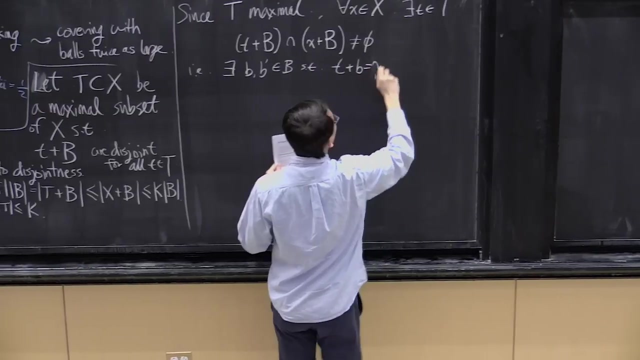 one of my children translates. If this were not true, then I could have put in an extra translate of b. So in other words, there exists two elements, b and b prime, Such that T plus b equals to X plus b prime. 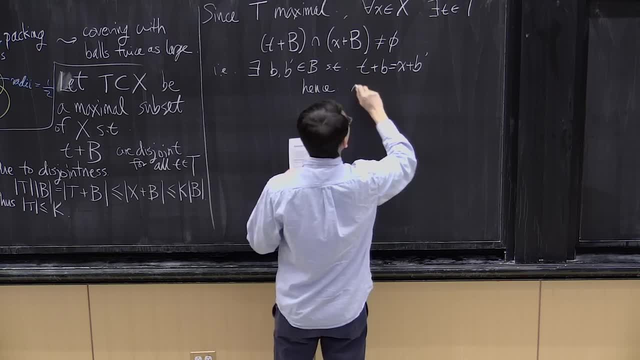 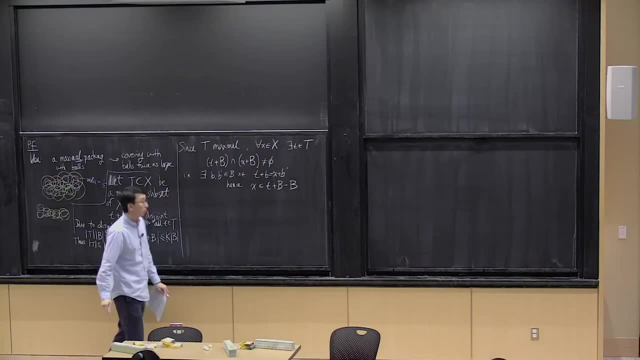 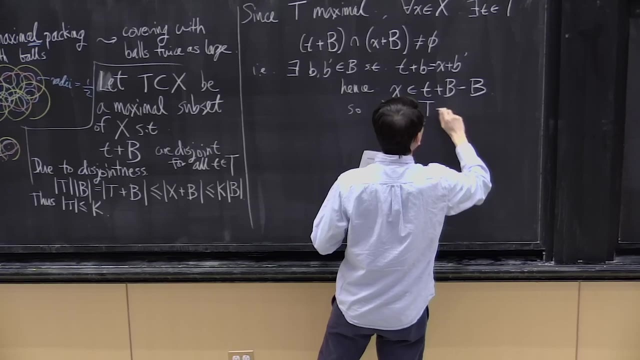 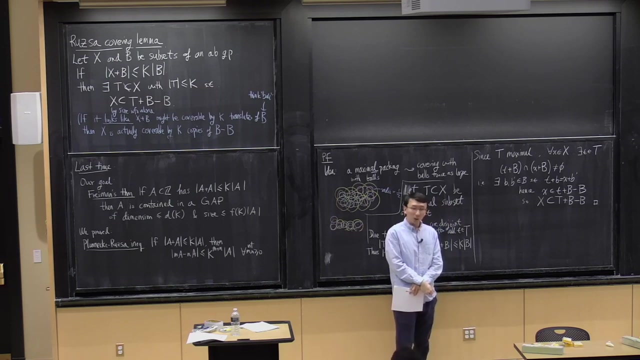 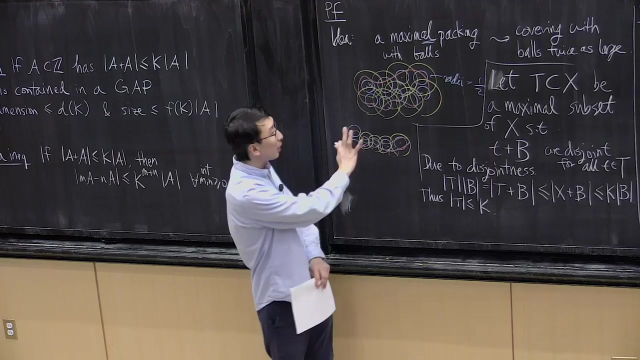 And hence X lies in little t plus b minus plus b minus b, which implies that the set X lies in T plus b minus b. OK, so that's the Ruzsa covering lemma. So it's an execution of this idea I mentioned earlier. 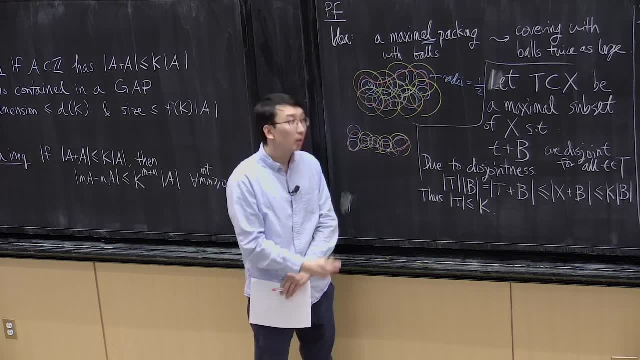 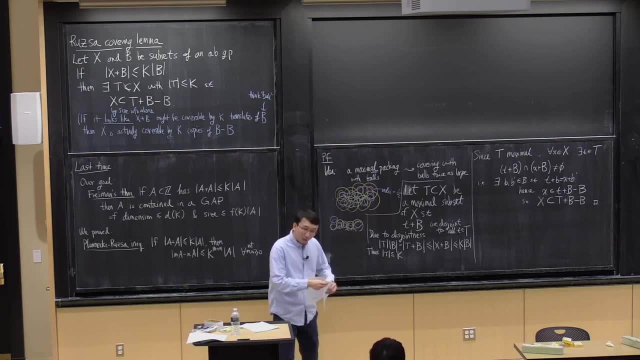 that a maximal packing implies a good covering Any questions. So now we have this tool, We can prove an easier version of Freiman's theorem where, instead of working the integers, we're going to work in the finite field model. OK, 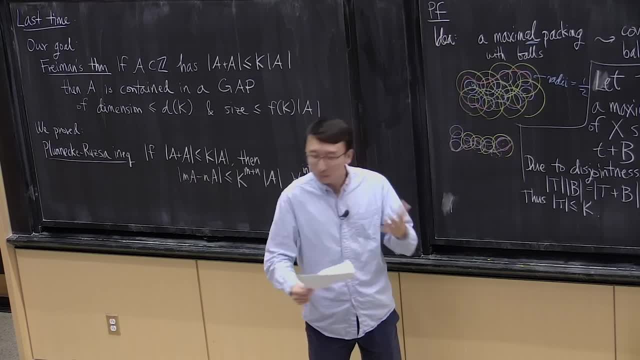 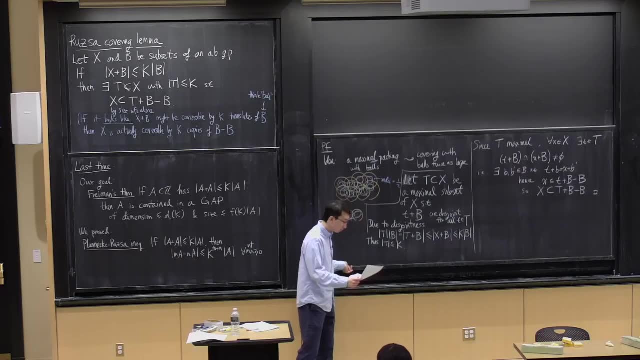 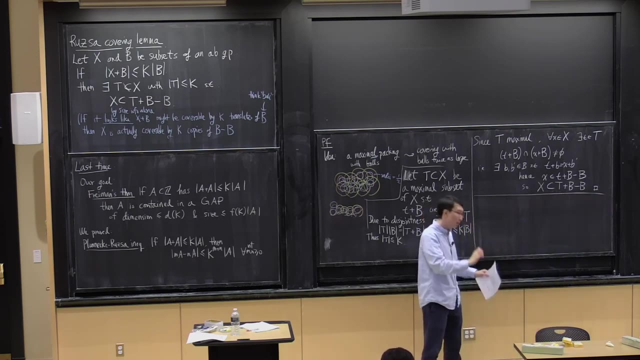 Usually it's good to start with finite field models. Things are a bit cleaner In this case. it actually only requires a subset of the tools that we'll need for the full theorem. So instead of working finite field model, we're going to work in something just slightly more general. 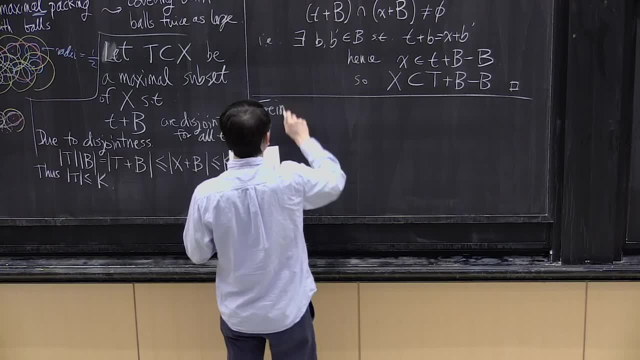 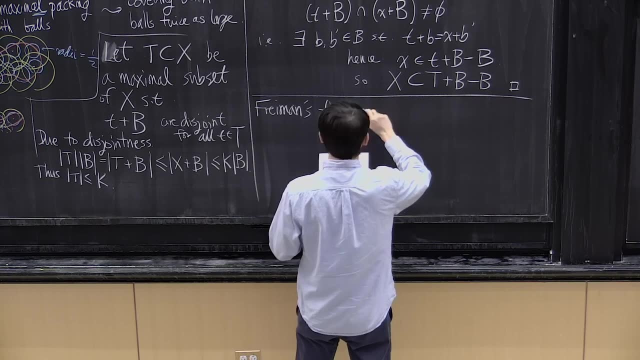 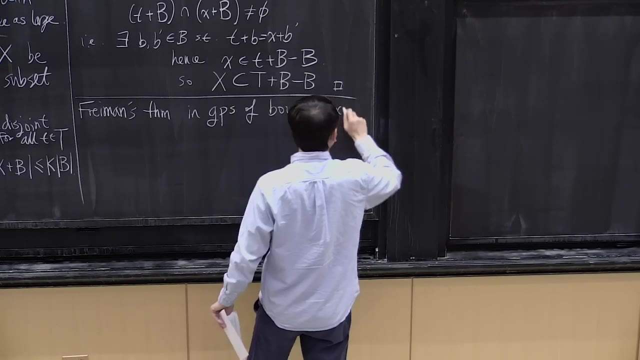 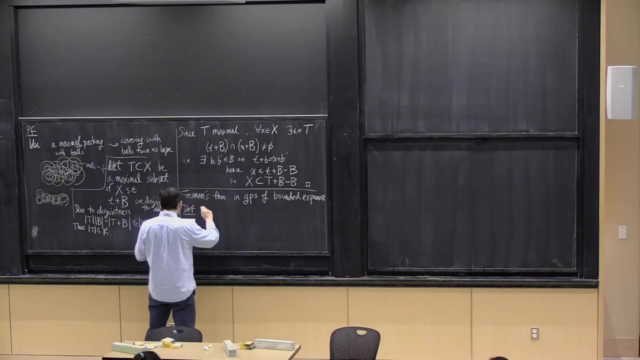 but it's the same proof. So we're going to be working in a group of bounded exponent- Freiman's theorem in general. So we are going to work in groups of bounded exponent. And the word exponent in group theory means the following: 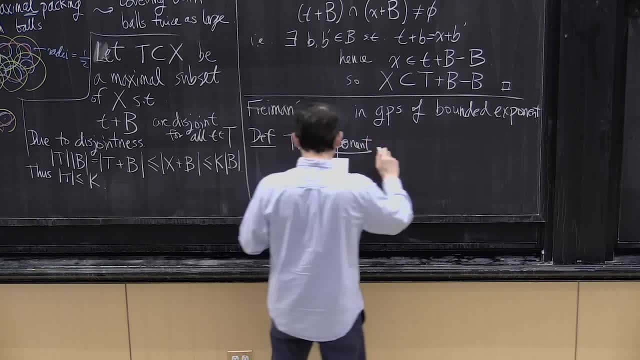 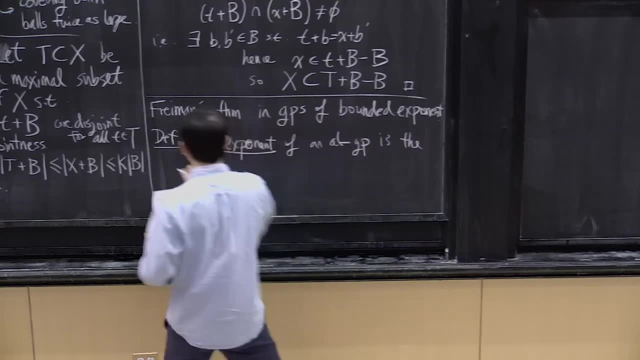 So the exponent of an abelian group is the smallest positive in the polar grains And this is going to be the lowest positive in the group, And what we're going to do is we're going to work this out. It's going to be a little bit confusing. 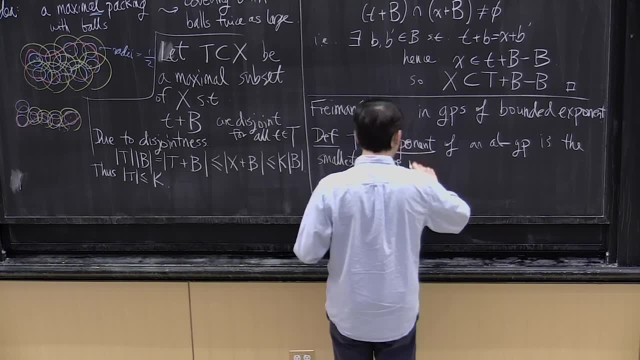 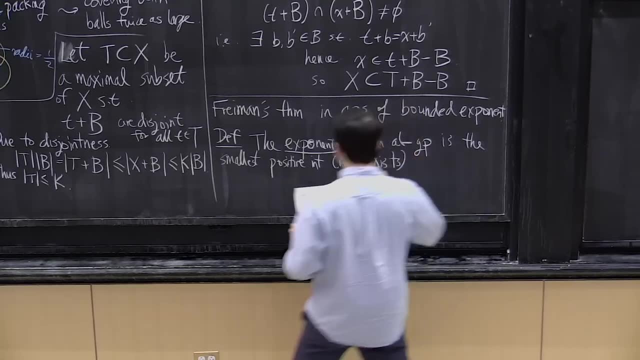 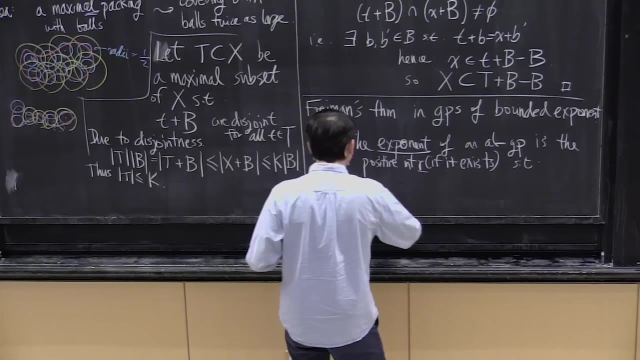 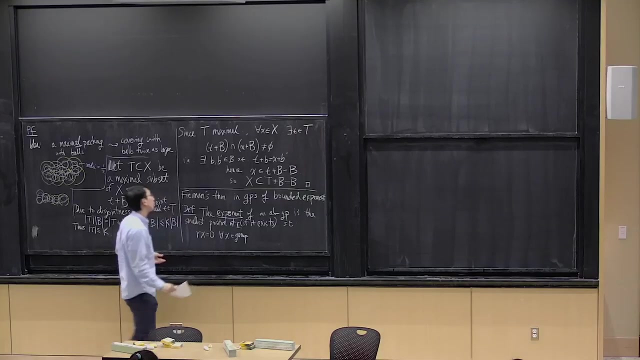 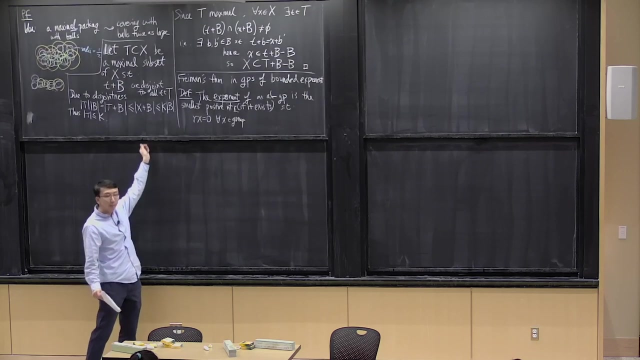 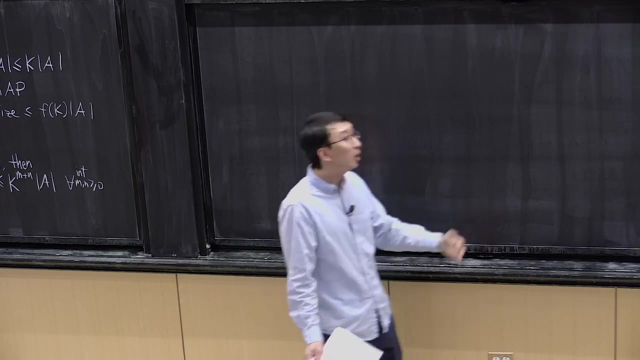 of integer, if it exists, so the smallest positive integer, r, so that rx equals to 0 for all x in the group. So, for example, if you are working fp to the n, then the exponent is p, So every element has, if you add to itself r, times. 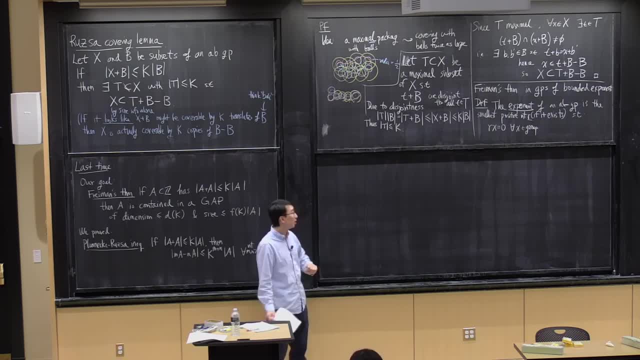 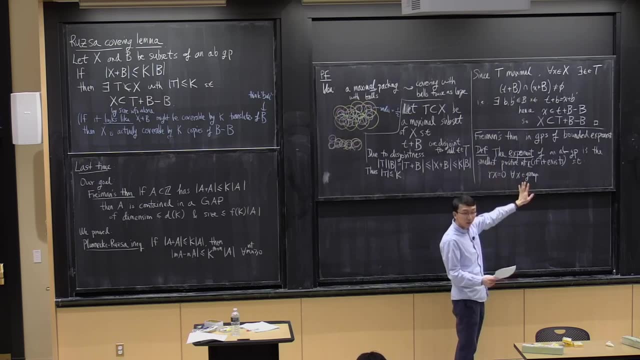 then it vanishes the element The name of the word exponent comes from. I mean you can define the same thing for non-obelient groups, in which case you should write this expression using the exponent instead. Instead of addition, you have multiplication. 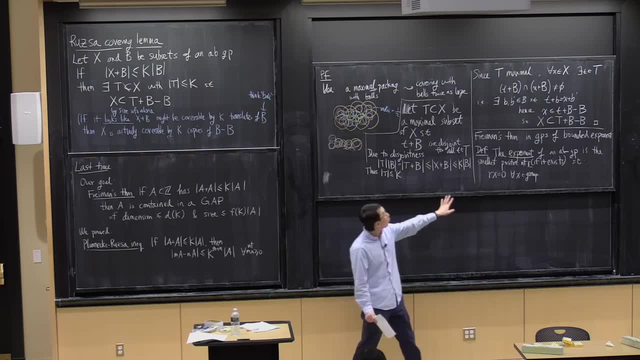 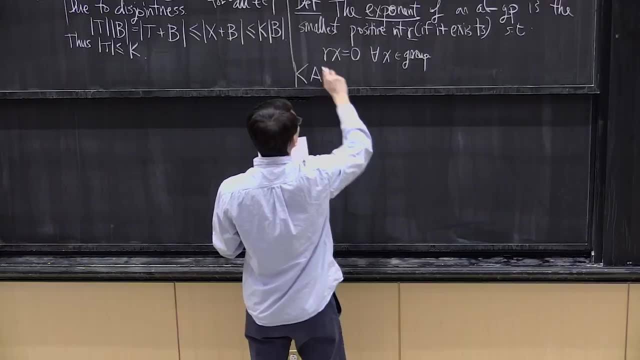 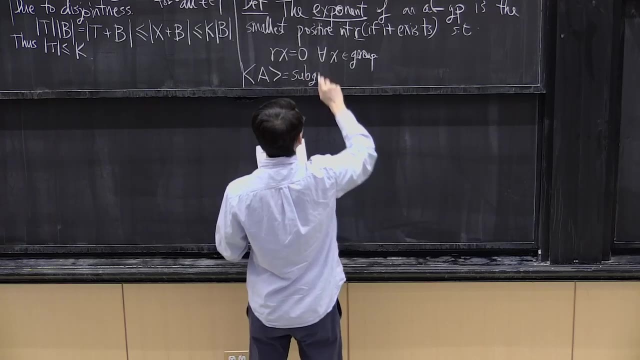 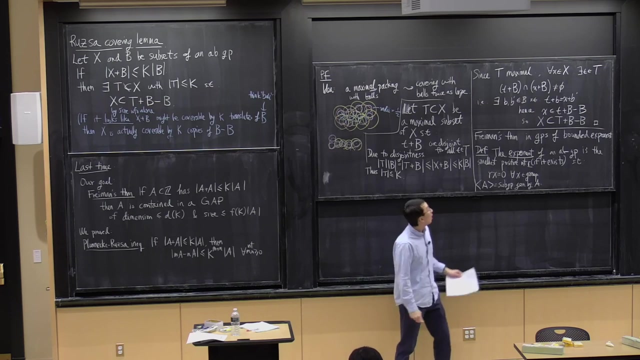 So that's why it's called exponent, so the name is stuck, even though we're still working in the additive setting. We're going to write this. so the angle brackets to mean the subgroup generated by the subset A. A is a subset of the group elements. 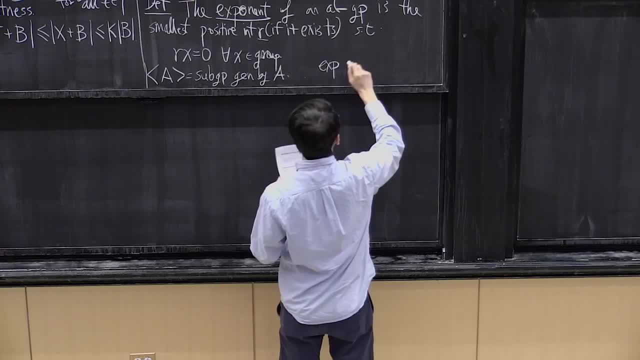 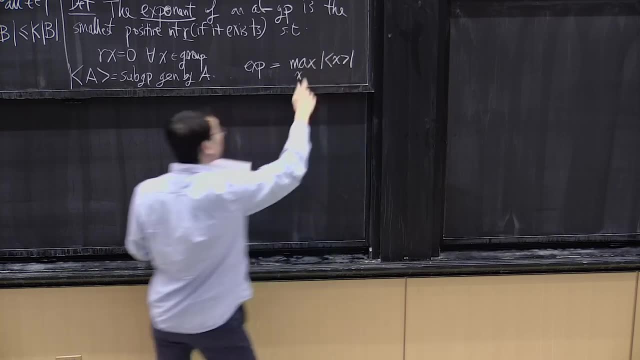 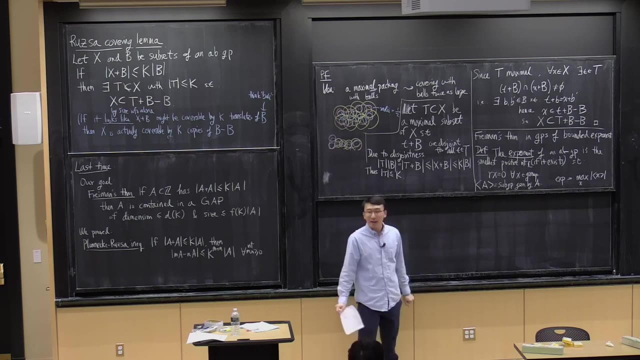 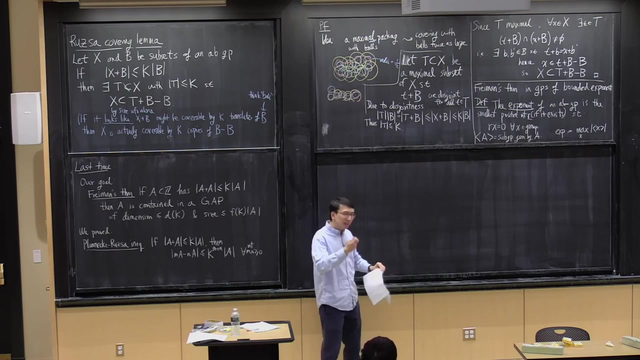 And so the exponent A is a subset of a group then- is equal to the maximum number of. so if you pick a group element, look at how many group elements does it generate. So it's equal to the max. All right, so the example you can have in mind. 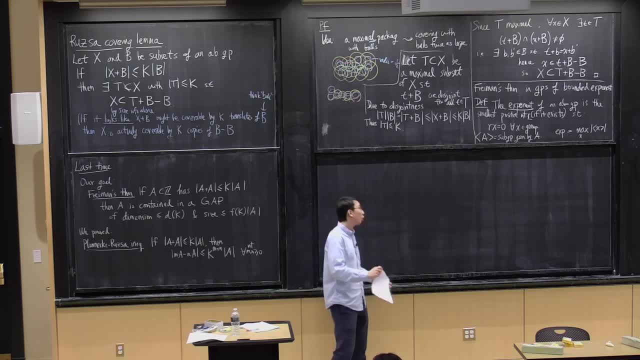 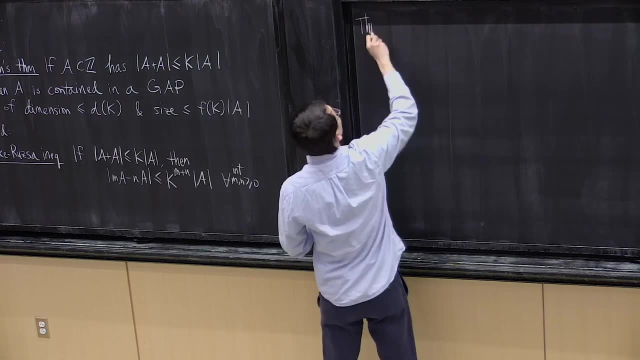 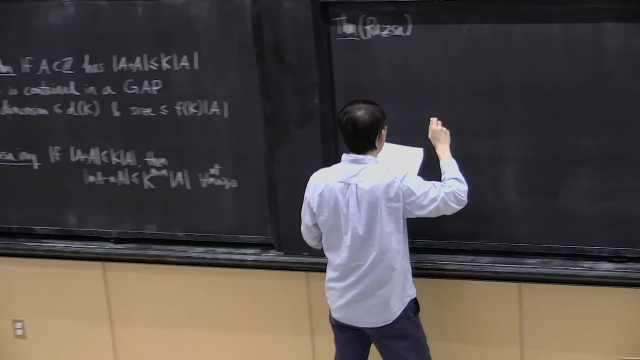 is f2 to the n which has exponent 2.. So in general we're going to be looking at a spectrum, but a special case in a group with bounded exponent, And Freiman's theorem in this case is due to Grusha, who showed that if you 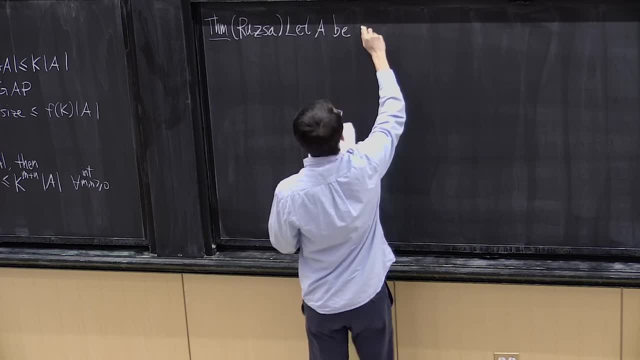 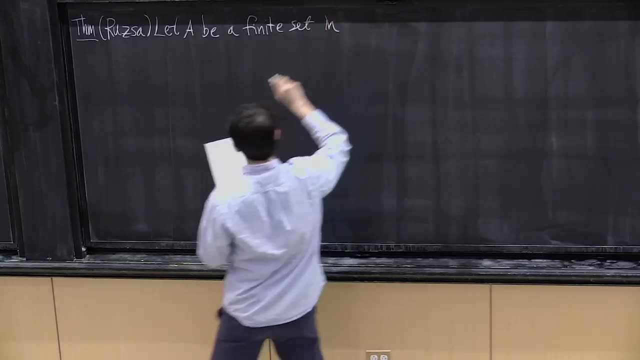 have a finite subset in an abelian group, then you have a finite subset. So if you have a finite subset in an abelian group, then you have a finite subset. So if you have a finite subset in an abelian group, then you 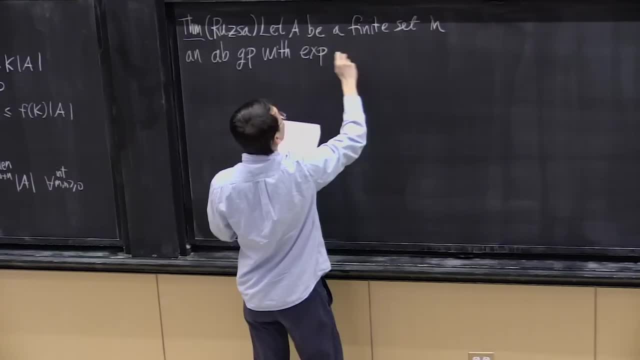 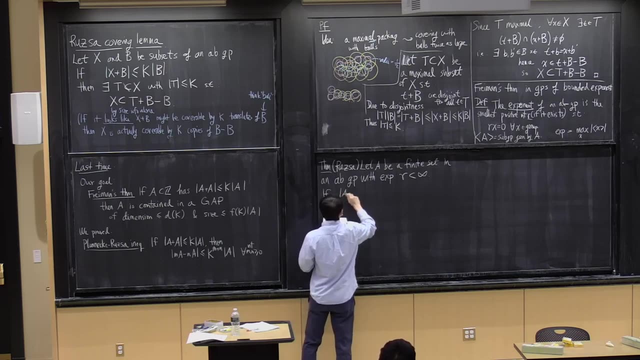 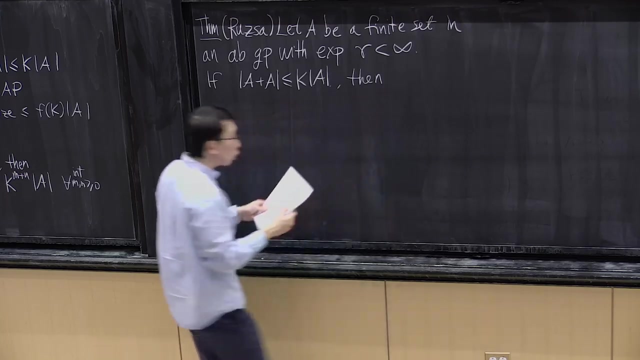 have a finite subset. And so if you have a finite subset in a group with exponent r, so a finite exponent, if A has doubling constant, at most k, then what do we want to say? We want to say, just like in Freiman's theorem: 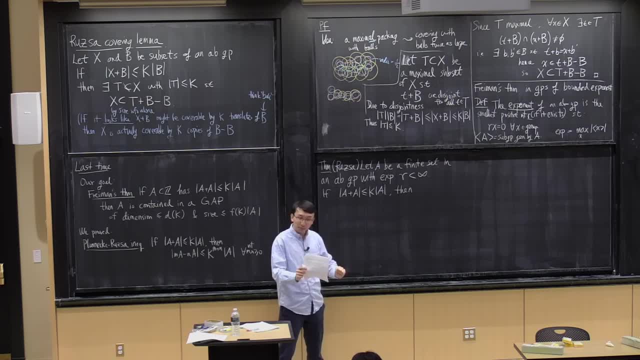 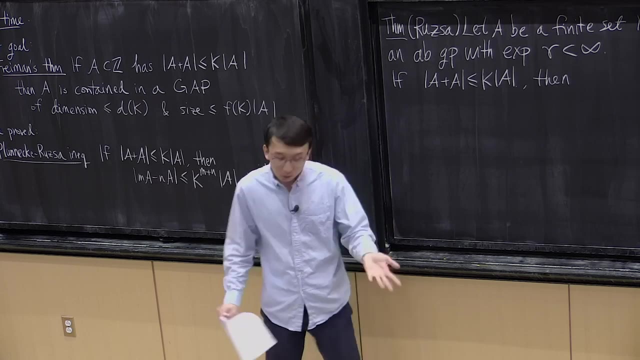 that if A has bounded doubling, then it is a large portion of some structured set, And here structured set means subgroup. OK, Well, if you're going to be looking at subgroups that contain A, you might as well look at the subgroup generated by A. 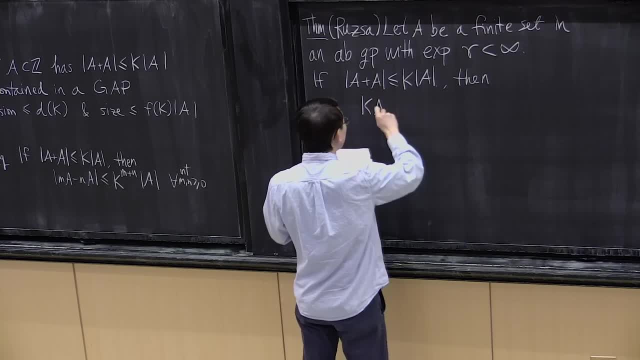 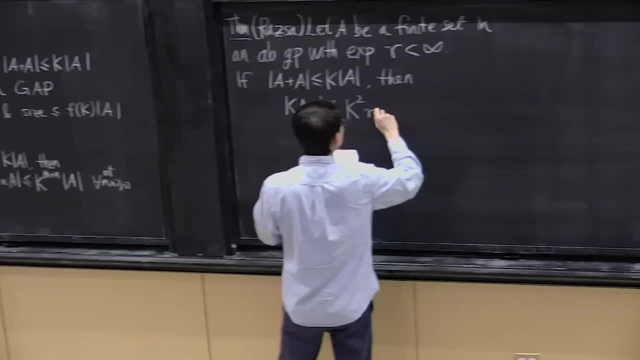 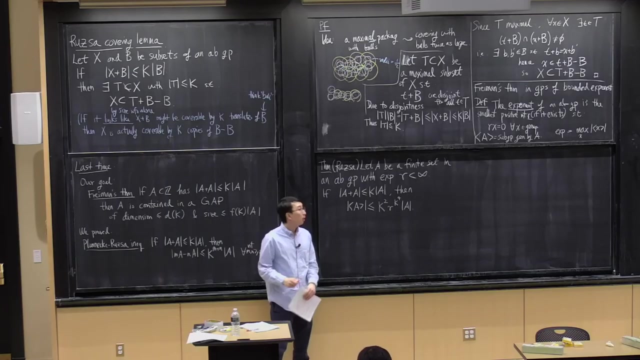 So the claim then is that the subgroup generated by A is only a constant factor bigger than A itself. So let me say it again: If you have a set A in a group, then you have a bounded exponent and A has bounded doubling. 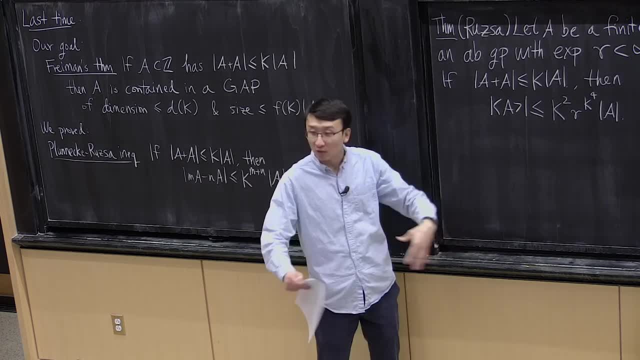 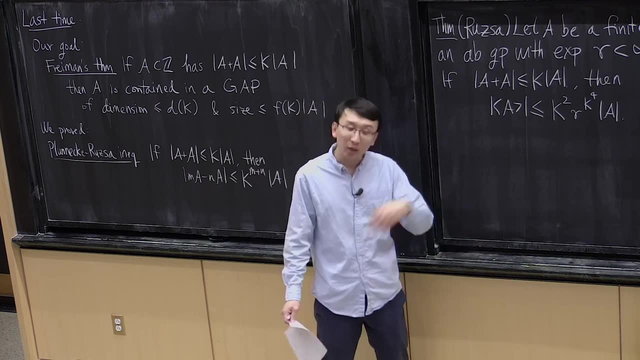 then conclusion is that A is a large proportion of some subgroup. Conversely, we saw last time, if you take a subgroup, it has doubling constant 1. So if you take a positive proportion, a constant proportion of the subgroup, it also has bounded doubling. 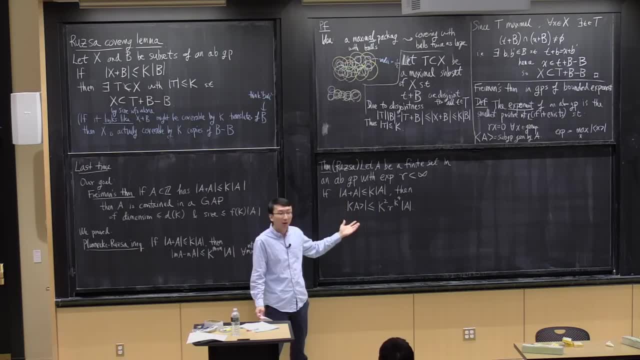 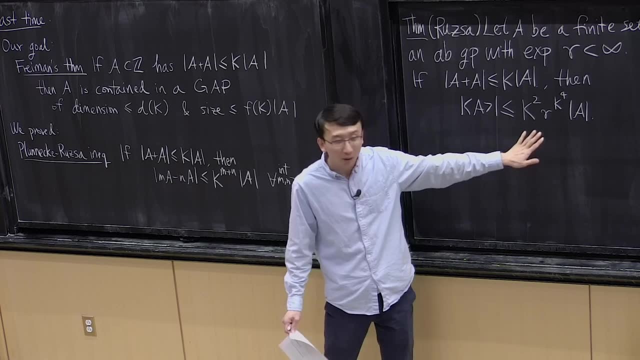 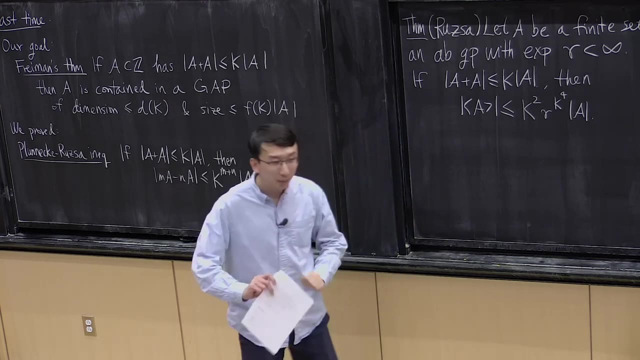 And this statement is in some sense a converse of that observation. OK, This bound here is not optimal. I'll make some comments about what do we know about these bounds, But for now just view this number as a constant. Any questions about the statement? 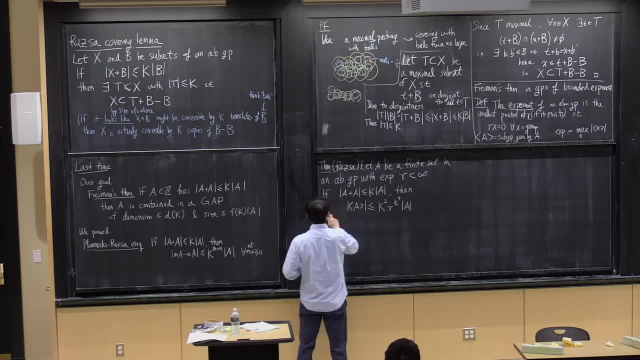 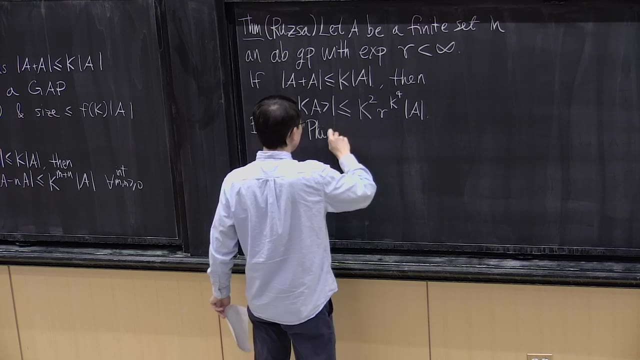 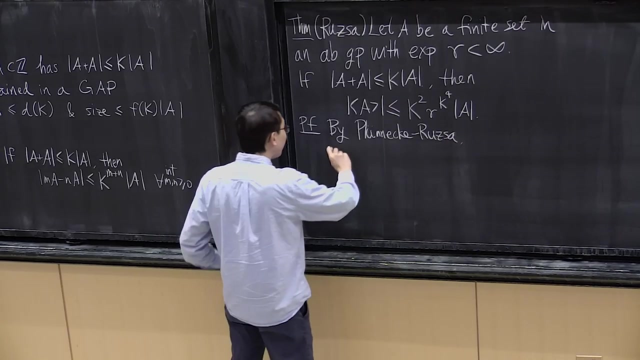 All right. So let's prove this Ruzsa's theorem, giving you Freiman's theorem in groups with bounded exponent. So we're going to be applying the tools we've seen so far, starting with Plinic-Ruzsa, So by Plinic-Ruzsa, inequality. we find that OK. so I'm 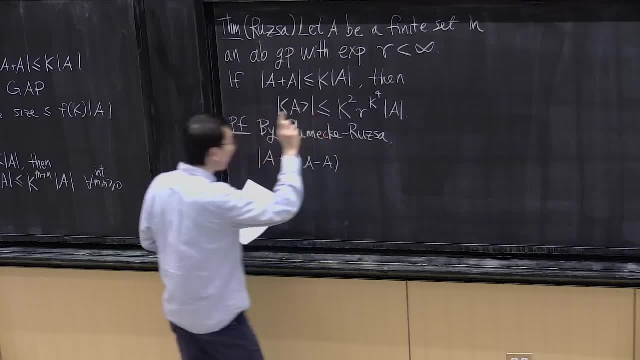 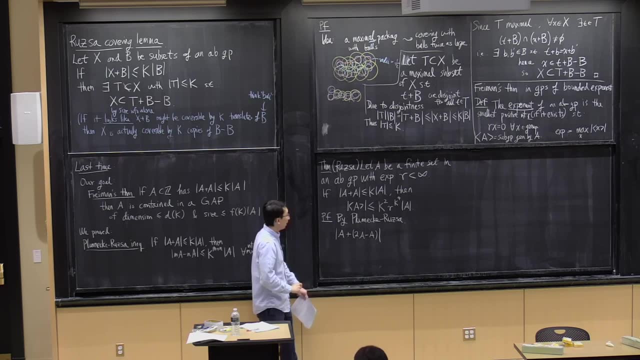 going to write down some expression. You might wonder why this expression? Because we're going to apply covering lemma in a second. So this set by Plinic-Ruzsa, its size is bounded because the set can also be written as 3A minus A. 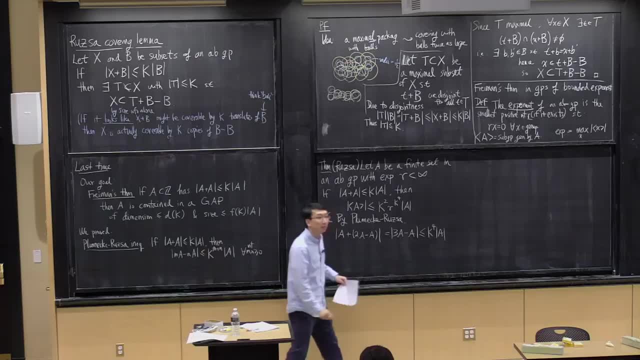 So its size is bounded. It's bounded by K to the fourth times size of A. So Plinic-Ruzsa is a very nice tool to have. It basically tells you if you have bounded doubling, then all the other iterated sums are essentially controlled. 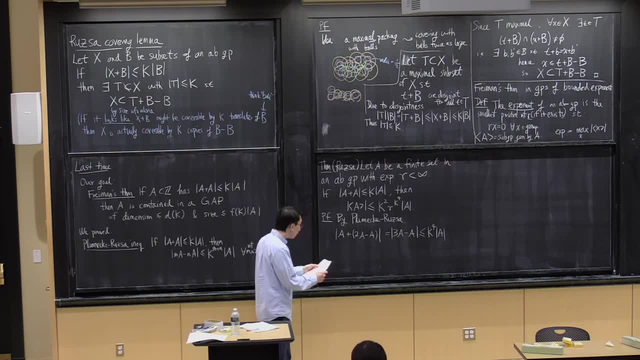 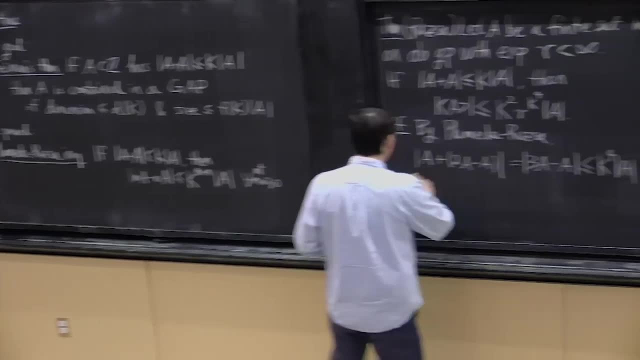 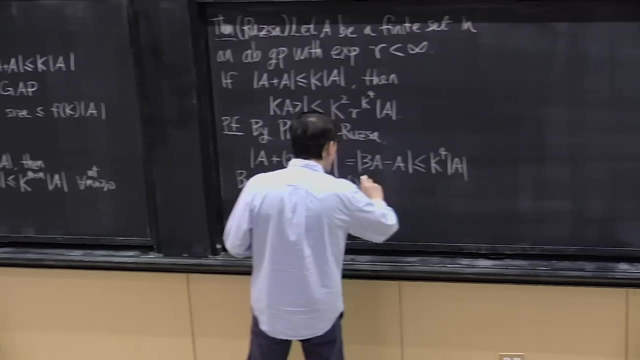 in size And now we're using that here. OK, So now we're in the setting where we can apply the Ruzsa covering lemma. So by covering lemma, OK. OK, We're going to apply the covering lemma, so using 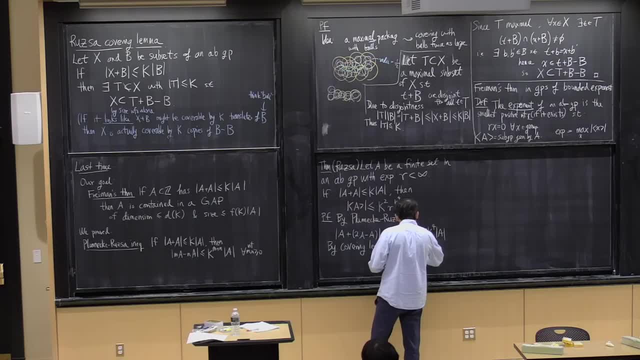 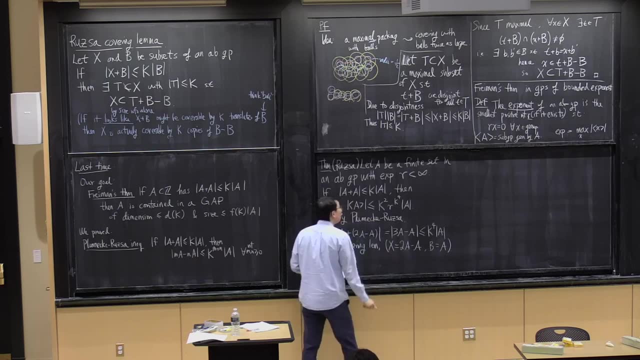 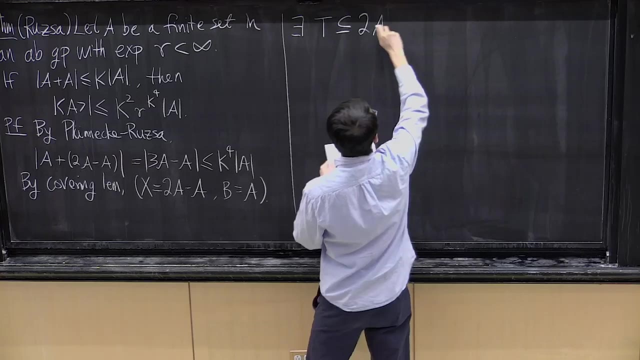 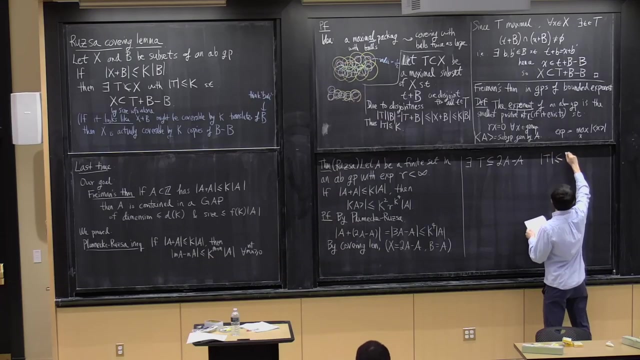 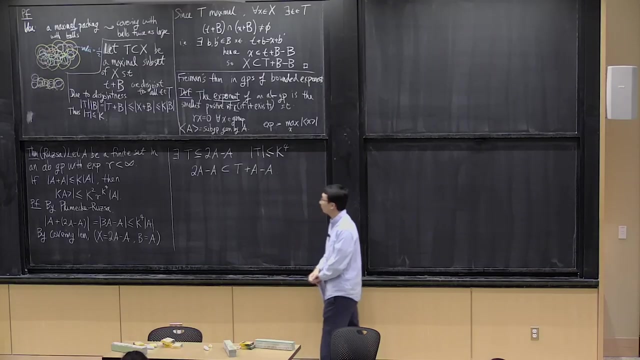 the notation earlier, with x equal to 2A minus A and B equal to A. By covering lemma, there exists some T being a subset of 2A minus A, with T not too large because of our earlier estimate And such that 2A minus A is contained in T plus A minus A. 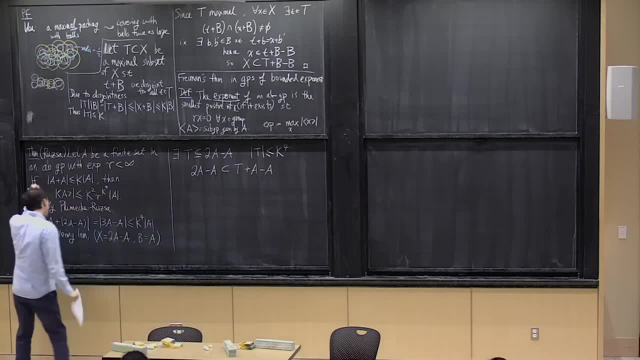 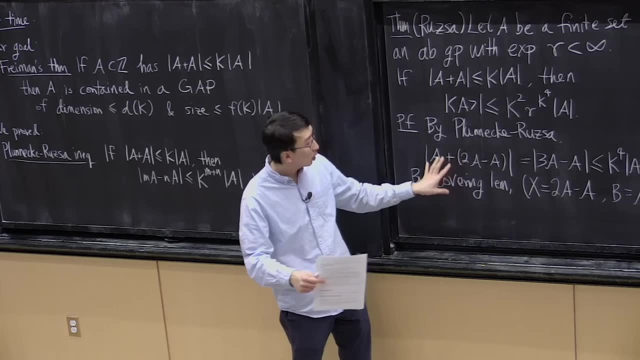 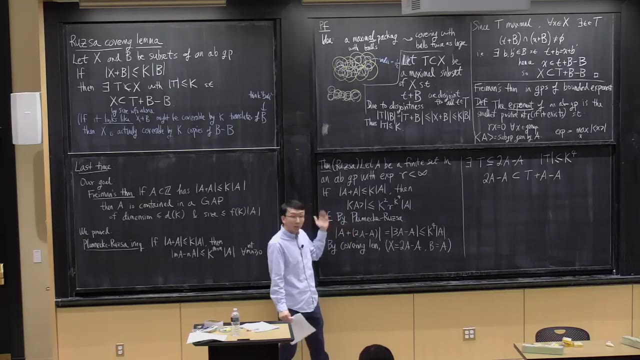 So it's easy to get lost in the details. But what's happening here is that I start with A and I'm looking at how big these iterated growing sumsets can be Right, And if I keep on doing this operation, like if I just apply Plunnecker-Ruzsa- 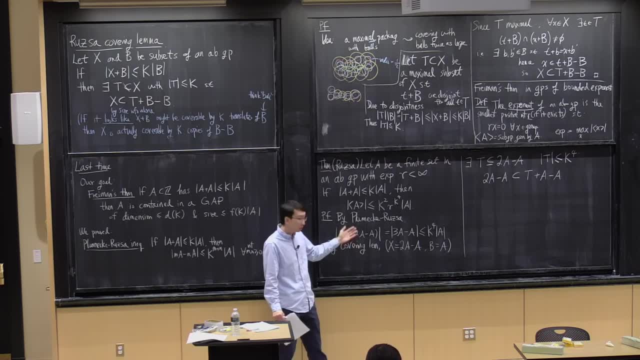 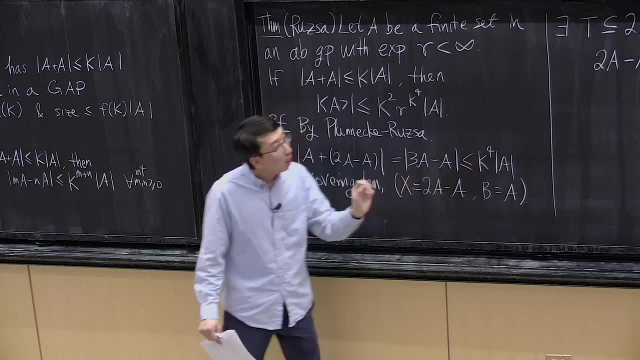 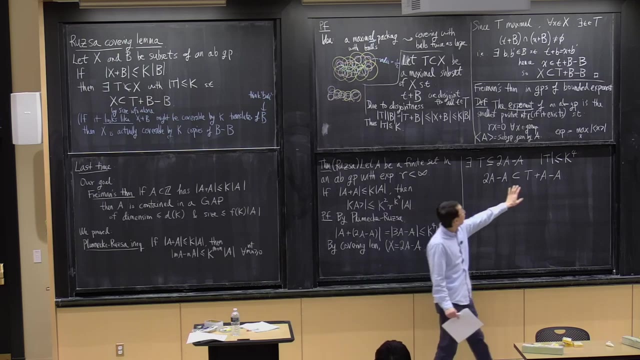 I can't really control the iterated sums by an absolute bound. This bound will keep growing if I take bigger iterations. But Ruzsa covering lemma gives me another way to control the bounded iterations. It says there is some bounded set T such that this iterated. 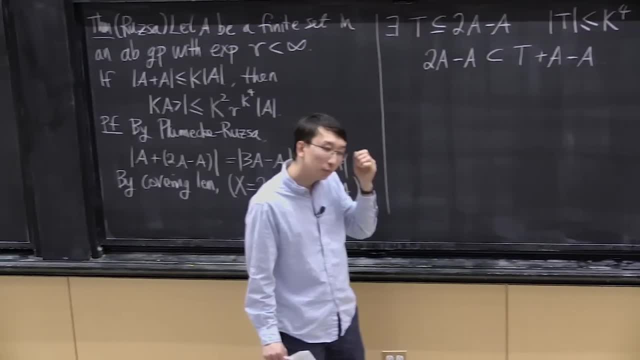 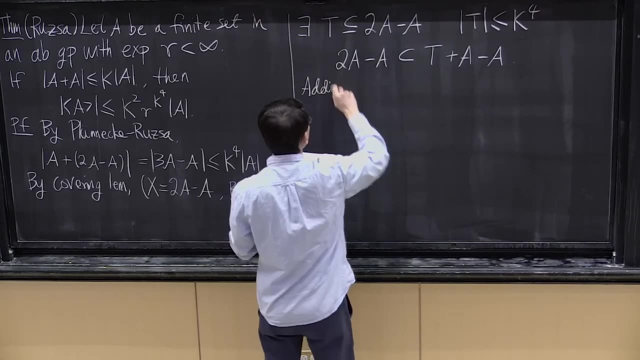 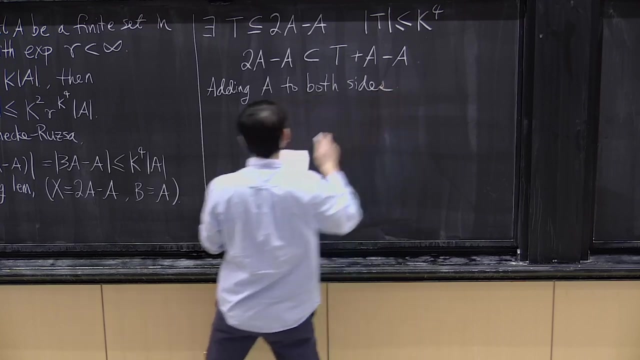 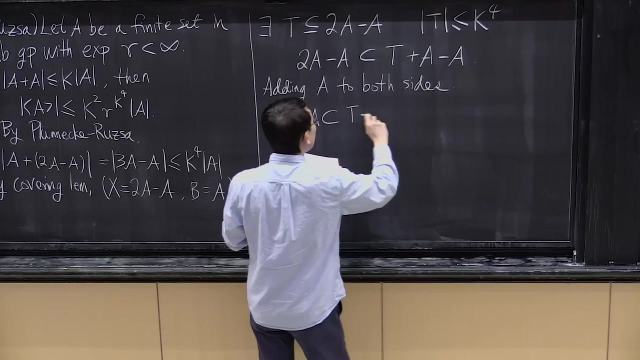 sum is nicely controlled, So let me iterate this bound even further. We're going to iterate the containment by adding A to both sides, A to both sides, And we obtain that 3A minus A is contained in T plus 2A minus. 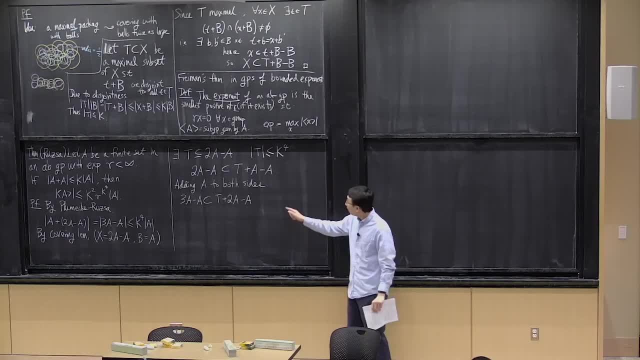 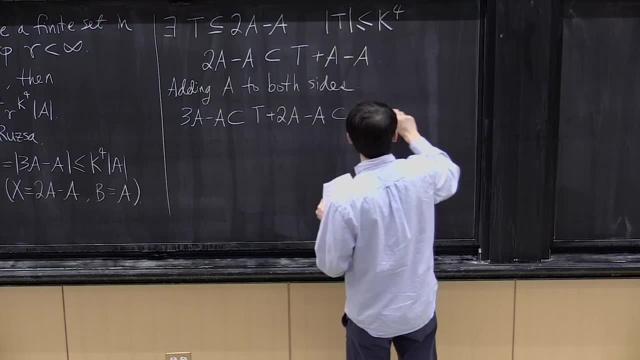 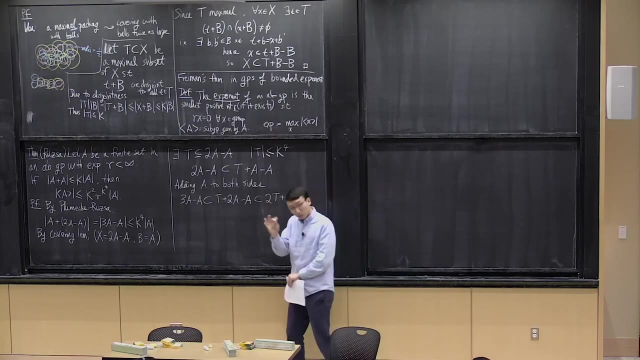 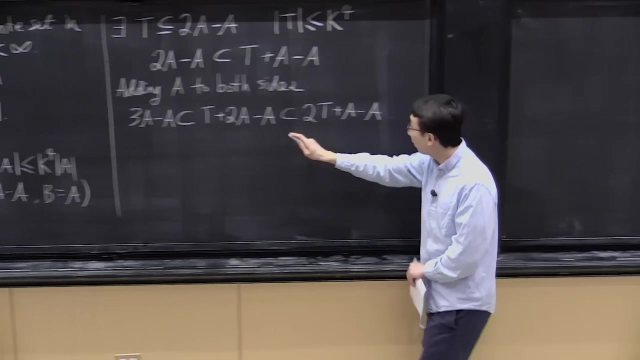 A. But now 2A minus A was containing T plus A minus A, So you get 2T plus A minus A. So now we've gained quite a bit because we can make this iteration go up, but not at the cost of iterating A, but at the cost of iterating T. 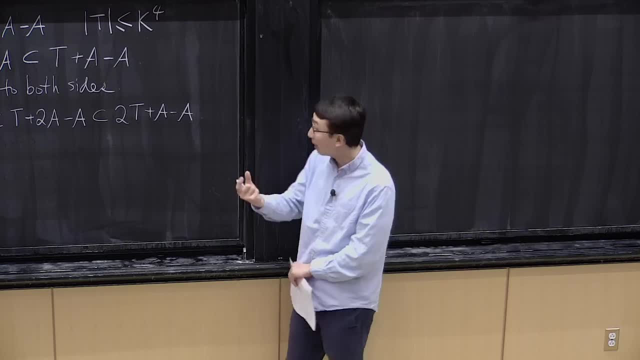 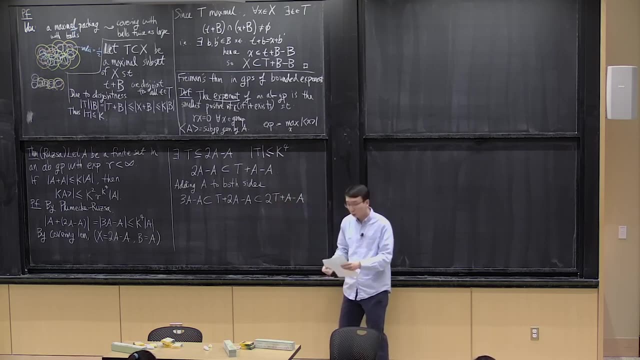 But T is a bounded size. T is bounded size, So T is bounded Right, OK OK. So T will have very nice control. We'll be able to very nicely control the iterations of T. So if we keep going so, we find that for all integer n. 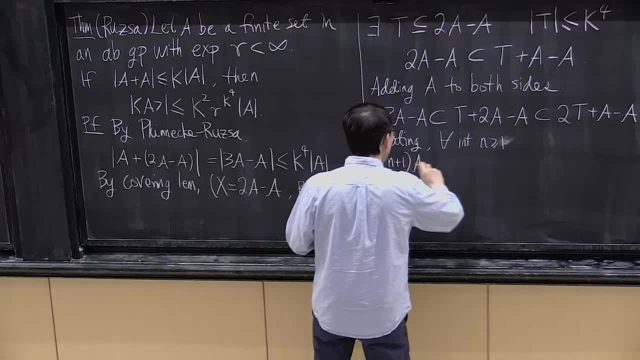 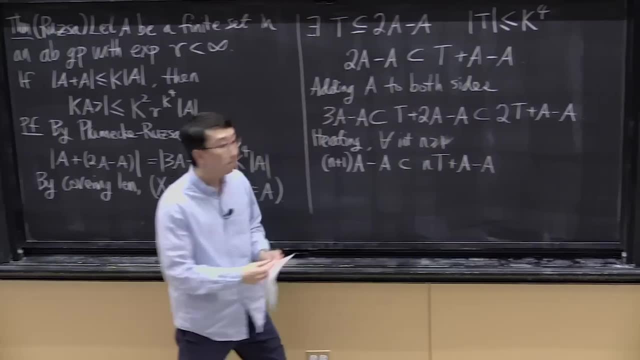 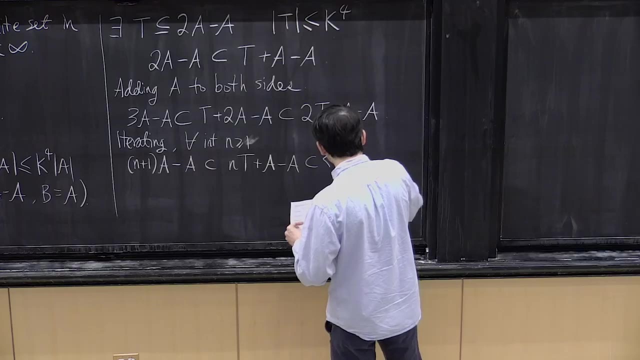 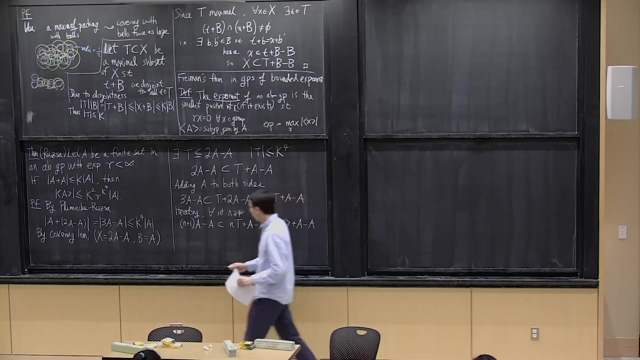 positive integer n, n plus 1A minus A, is contained in nT plus A minus A. But for every integer n, the iterated sum, the sums of T, are contained in the subgroup generated by T. So therefore, if we take n to be as large as you want, 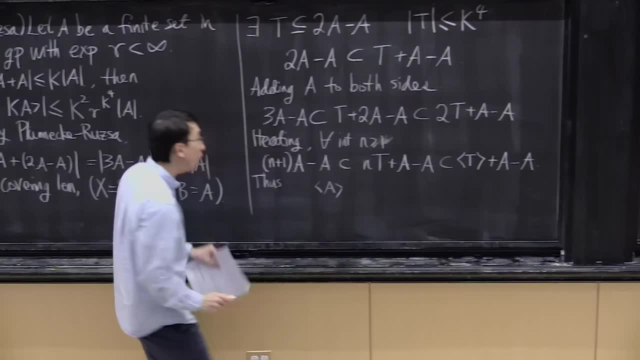 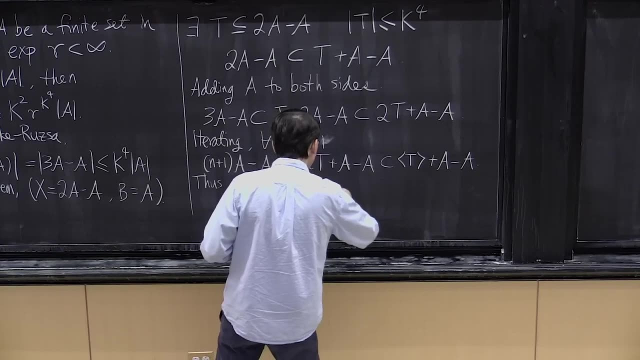 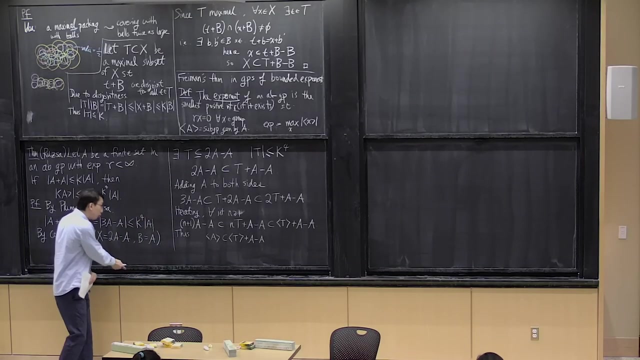 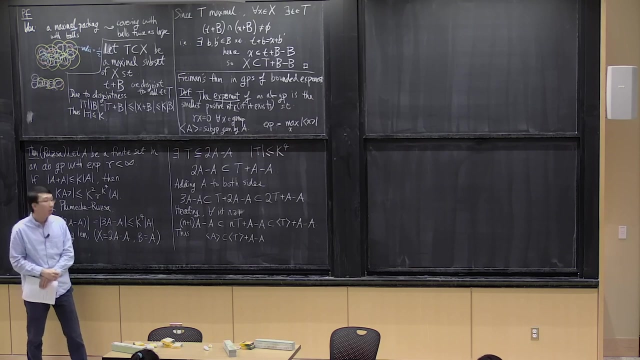 see that the left-hand side eventually becomes the subgroup generated by A And the right-hand side does not depend on n. So you have this containment over here. We would like to estimate how large the subgroup generated by A is. So you look at that formula and we 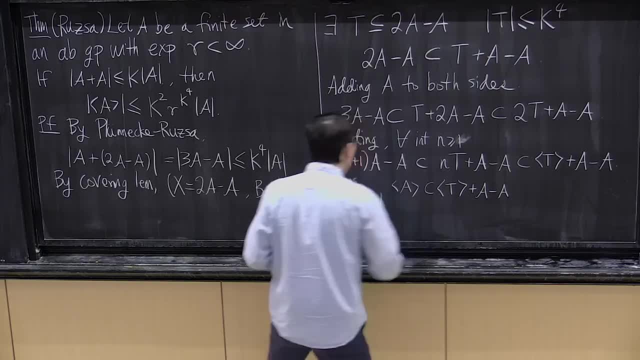 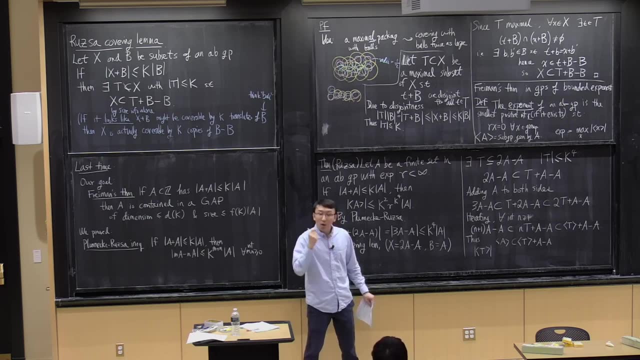 see that the size of the subgroup generated by T, And here is where we're going to use the fact that the assumption that the group has bounded exponent, Or so think, F2 to the n, if you will, F2 to the n. if I give you a set T, what's? 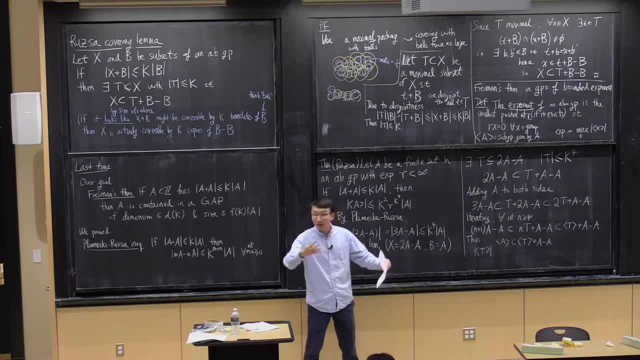 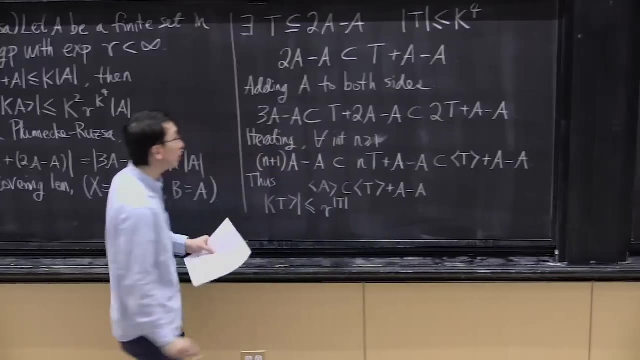 the subspace spanned by T. What's the maximum possible size? So at most 2 raised to the number. So in general you also have that the subgroup generated by T has size at most r raised to the size of T in a group of exponent r which we can control. 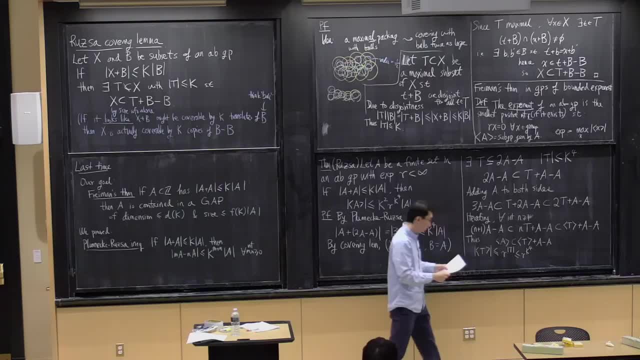 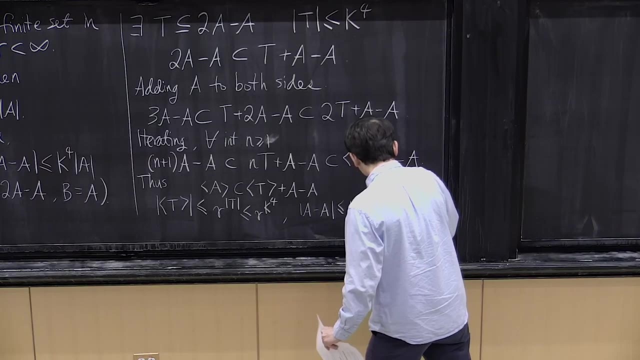 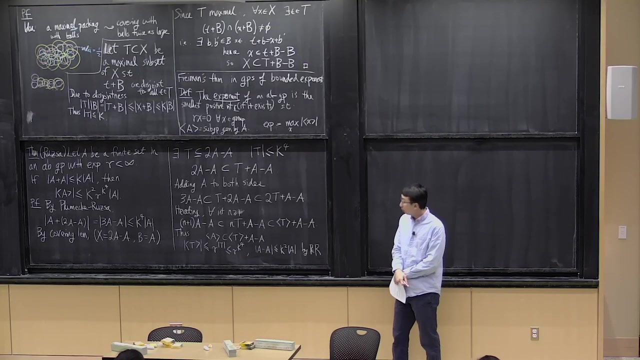 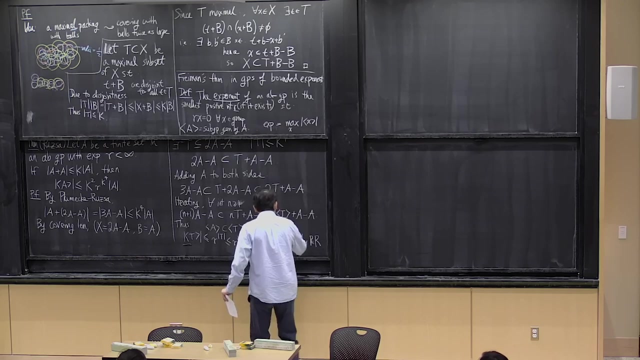 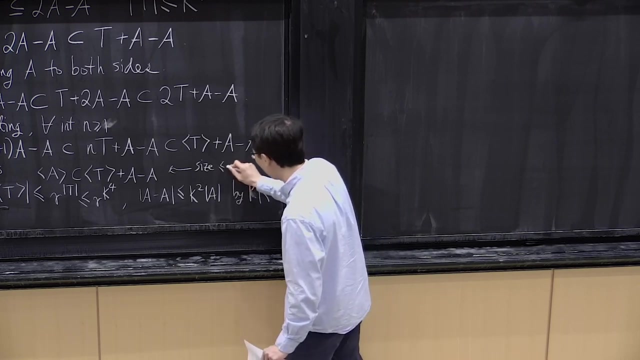 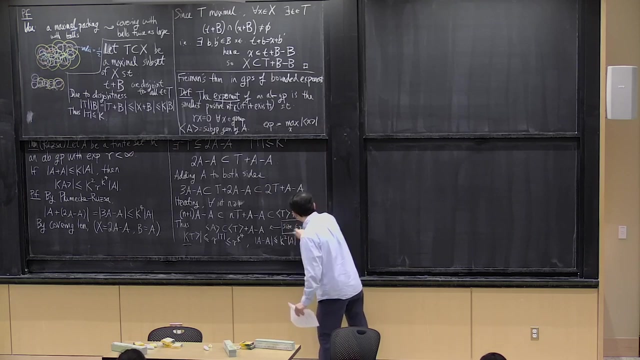 because T has bounded size And the second term A minus A. we also know how to control that by Plunica-Ruzsa, Therefore. so putting these two together, we see that the size up here is F. It is at most r to the k to the 4 times k squared size of A. 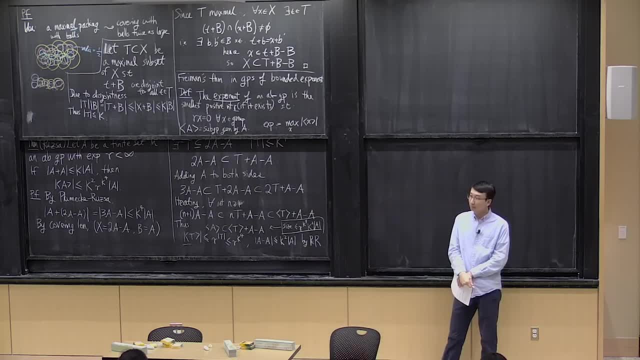 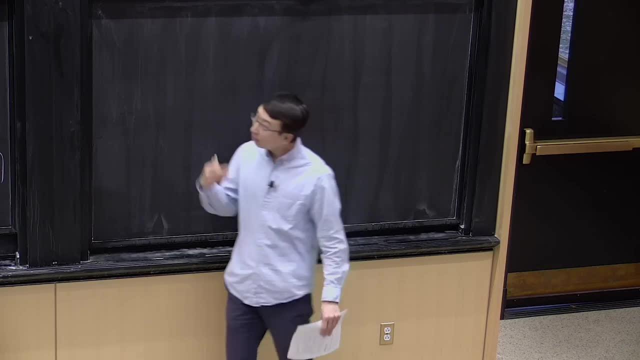 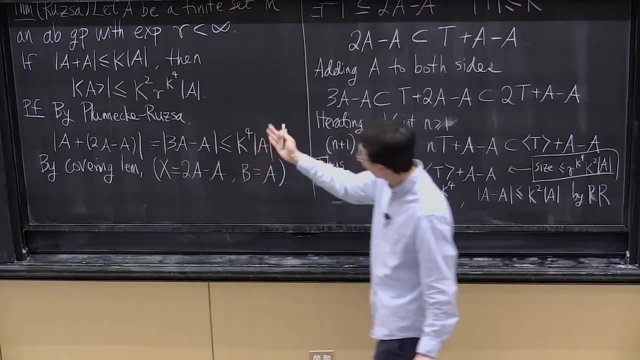 which is the bound that we claimed. Any questions? All right. so the trick here is to only use Plunica-Ruzsa somehow a bounded number of times. If you use it too many times, you can't. I mean this bound. 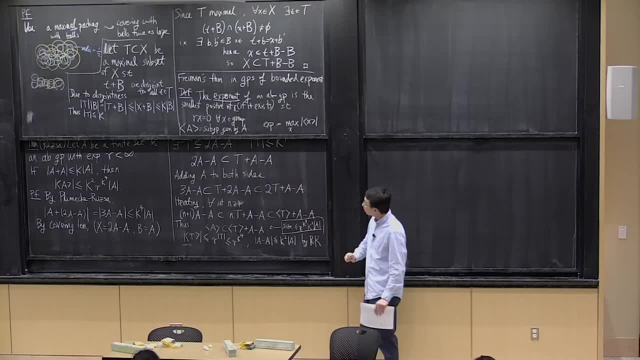 This bound blows up, But you use it only a small number of times And then you use the Ruzsa covering lemma so that you get this bounded set T that I can iterate. Let me make some comments about the bounds that come out of this proof. 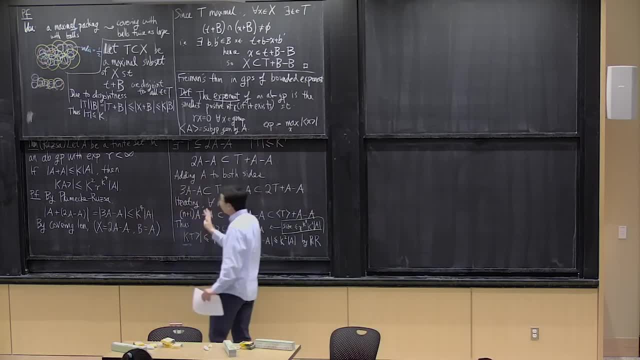 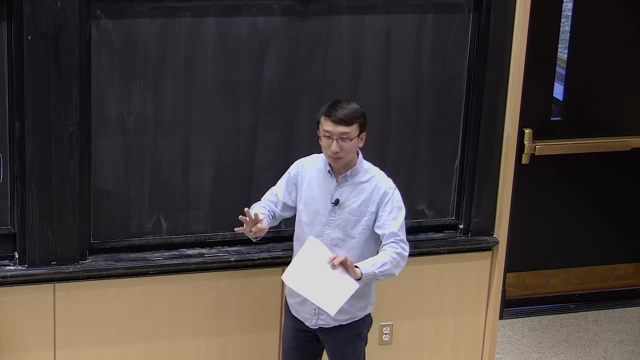 So you get this very clean bound just following this proof. But what about examples? So what kinds of examples can you think of where you have, say, a set of bounded doubling, but the set generated, the group generated by that set, is potentially large? 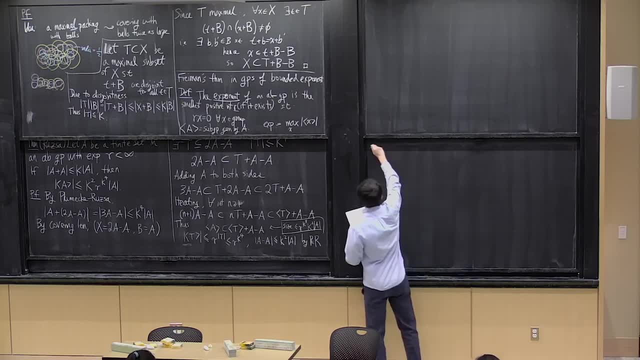 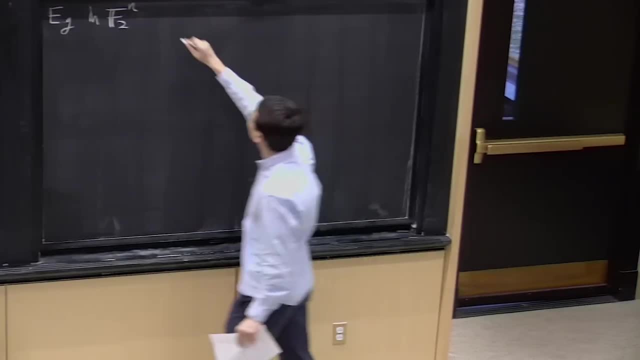 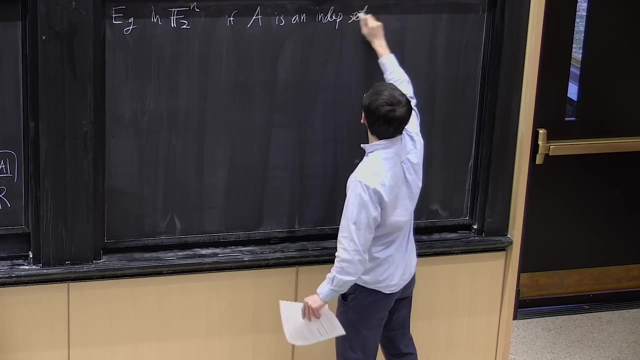 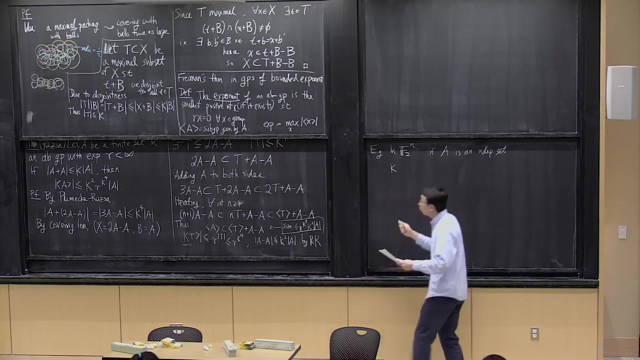 So even in F2, in F2 to the m. so if A is an independent set, so a basis or a subset of a basis, for instance, then K, so A is independent set. so all the pairwise sums are distinct. 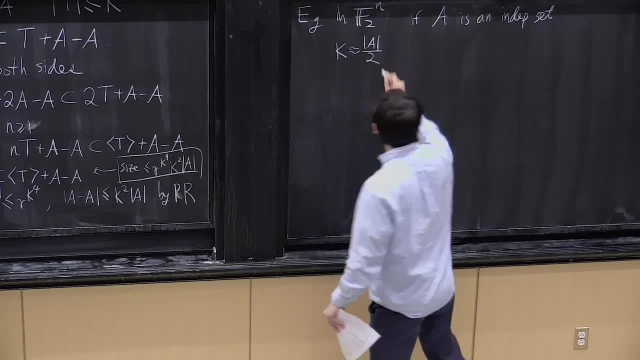 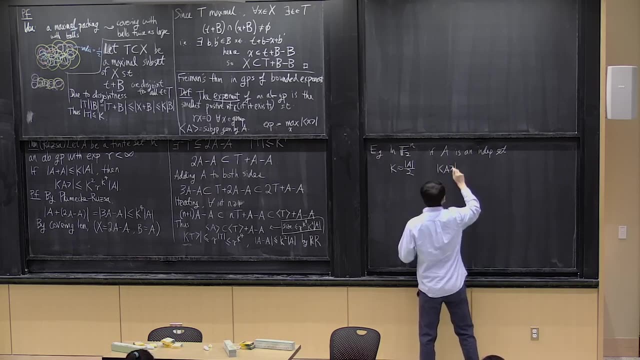 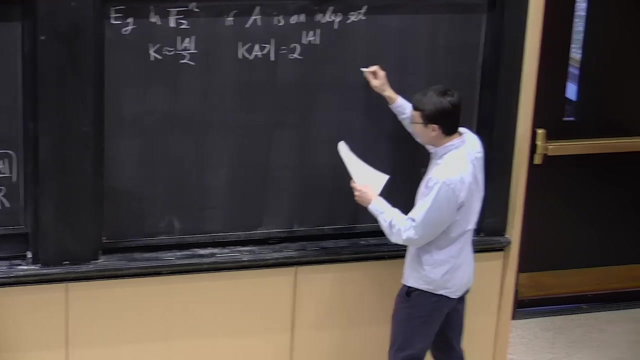 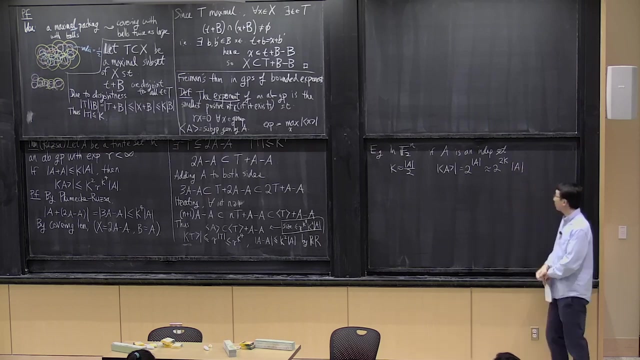 So K is about the size of A over 2.. That's the doubling constant, Whereas the group generated by A has size 2 to the size of A, which is around 2 to the 2K, And that's the size of A. 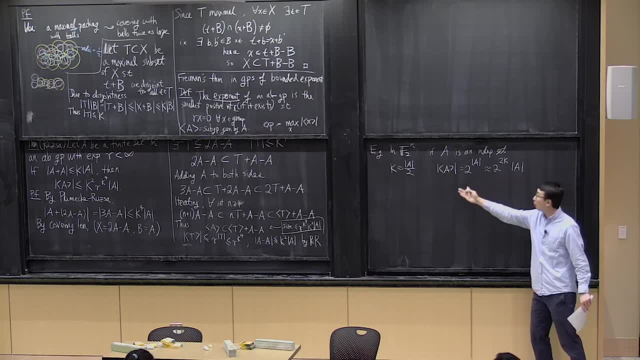 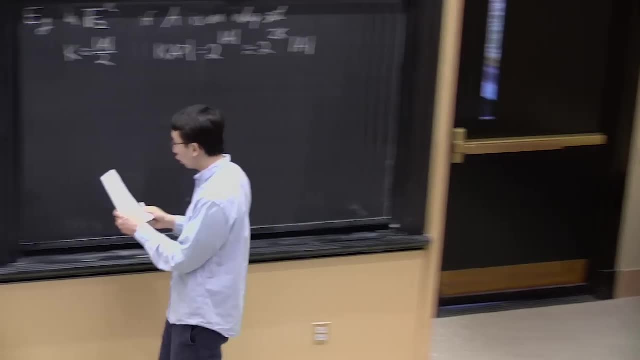 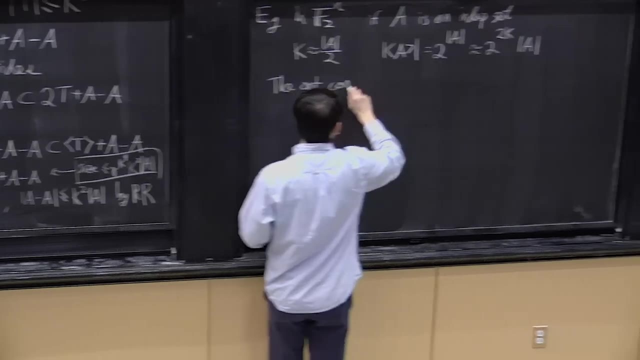 So you see that you do need some exponential blow-up from K to this constant over here, And it turns out that's more or less correct. So the optimal constant for F2 to the m? OK, so that's the optimal constant for F2 to the m. 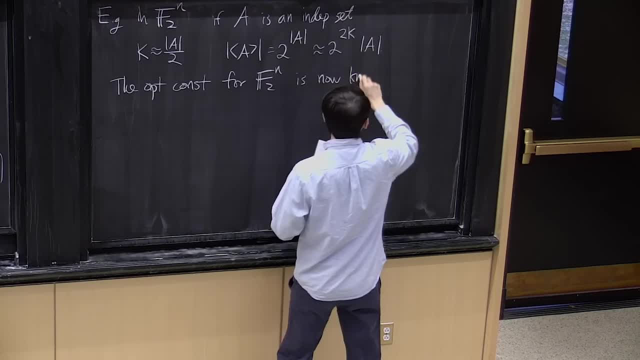 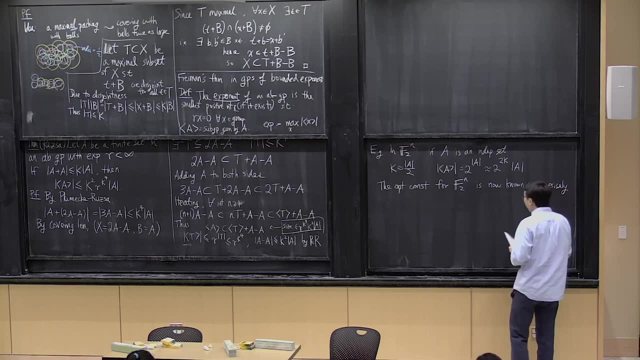 And it's now known very precisely. I said if you give me a real value of K, then I can tell you. there are some recent results that tells you exactly what is the optimal constant you can put in front of the A. So very precisely, 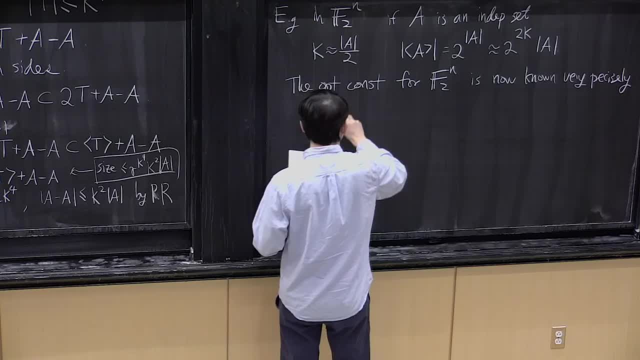 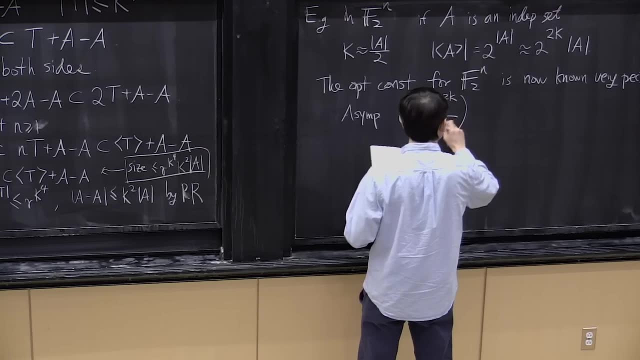 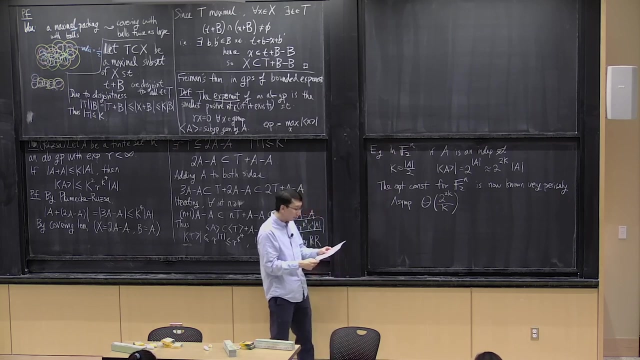 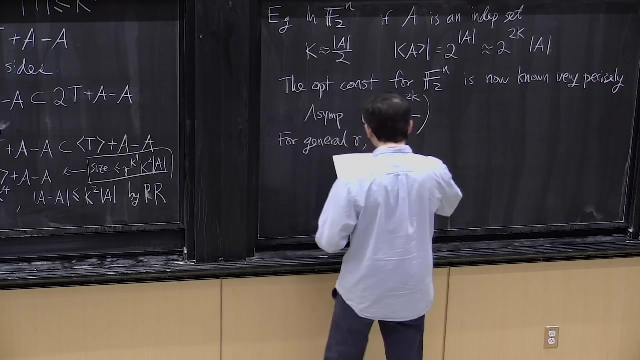 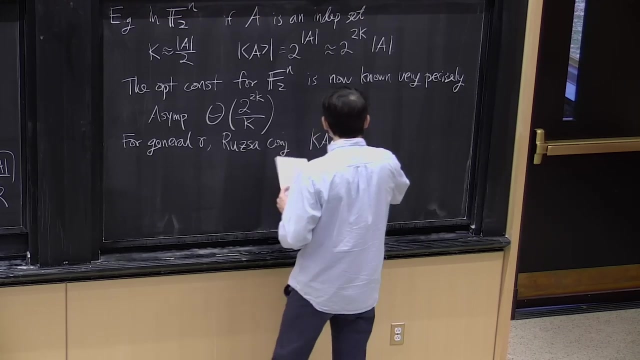 Asymptotically. it looks like 2 to the 2K divided by K. So that's what it looks like. So this example is basically correct. For general R we expect a similar phenomenon, So Ruzsa conjectured that in the hypothesis of the theorem. 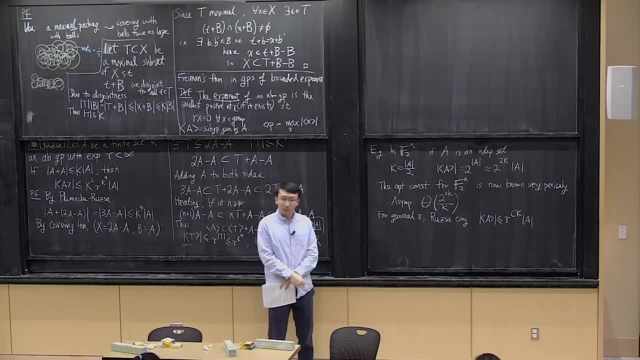 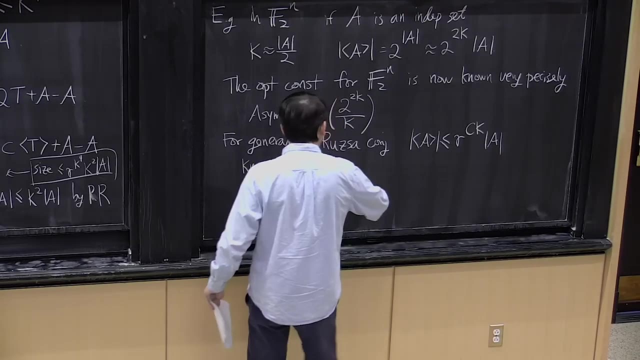 the constant you can take is only exponential in K, so R to the sum, The sum constant C times K. And it has been verified for some values of R but not in general, so known for some R, for example primes. 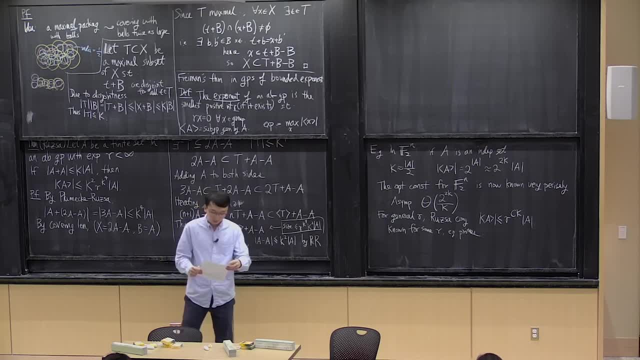 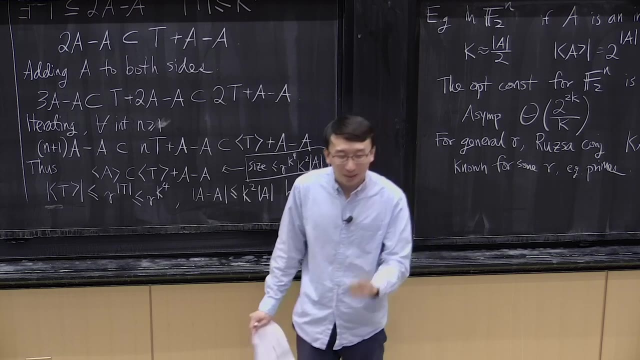 OK, any questions? All right, So this is a good milestone. So we've developed some tools and we were able to prove a easier version of Freiman's theorem in a group of bounded exponent. And you can ask yourself: does this proof work in the integers? 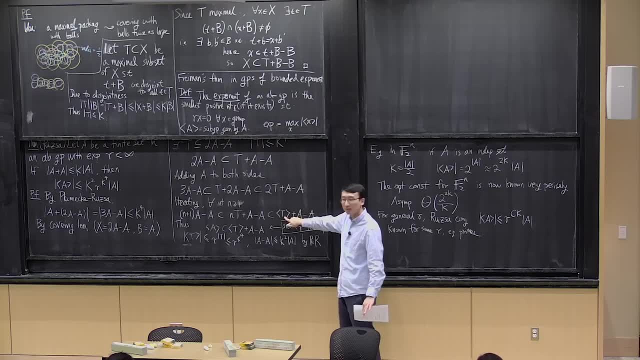 And literally no, because if you look at this proof, this set here is infinite, Unlike in a finite field setting in integers. well, that's not very good. So the strategy of Freiman's theorem, the proof of Freiman's theorem, is, to start with: 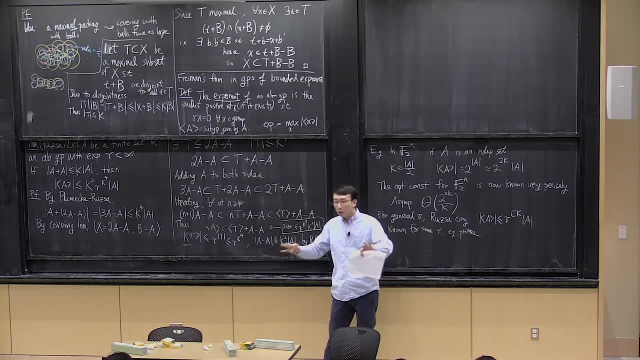 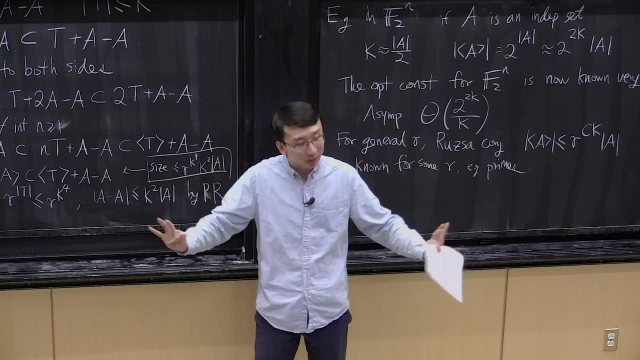 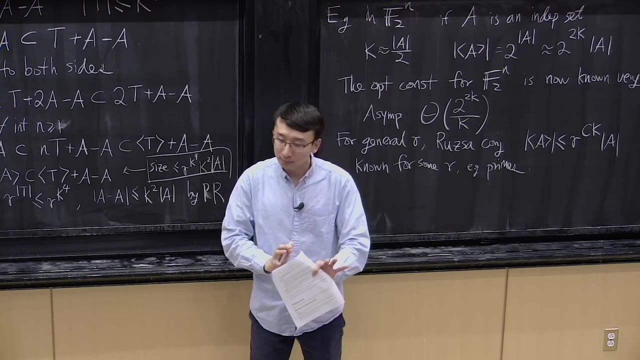 the integers and then try to not work in the integers but try to work in a smaller group. Even though you start in a maybe very spread out set of integers, I want to work in a much smaller group so that I can control things within that group. 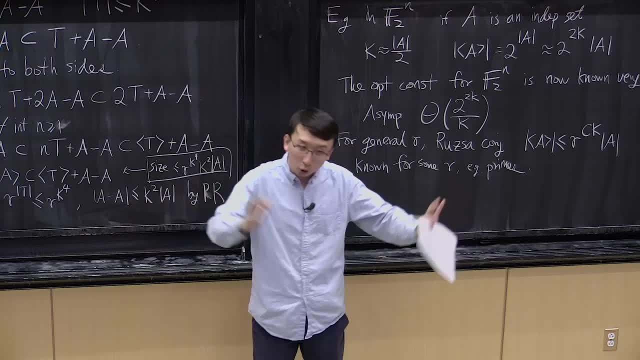 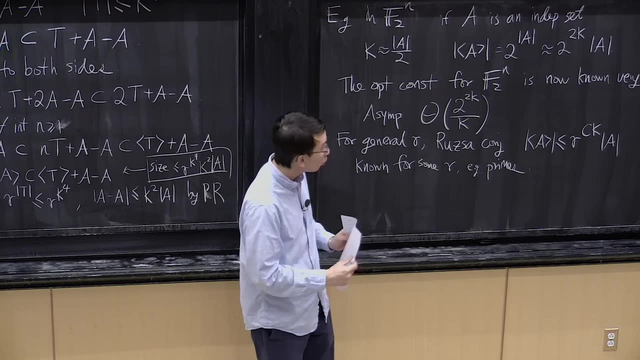 And this is an idea called modeling. So I have a big set and want to model it by something in a small group. So we're going to see this idea. But to understand, what does it mean to have a good model for a set in the sense of additive? 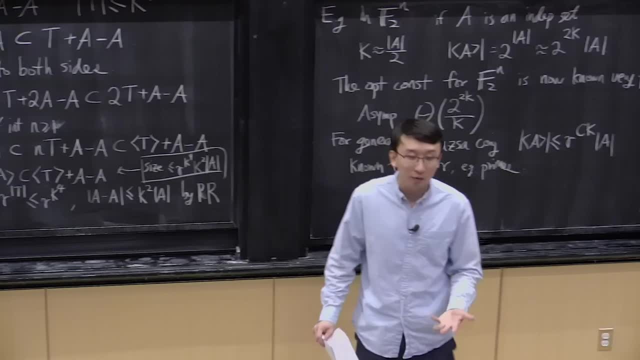 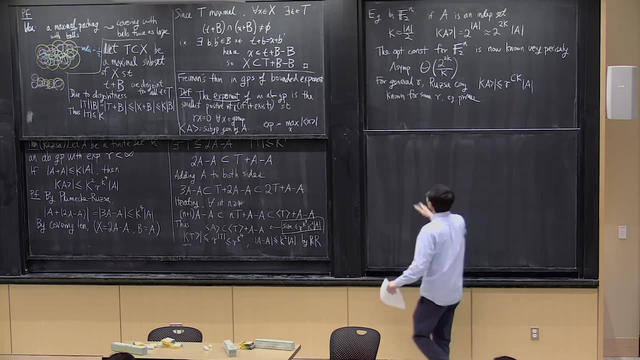 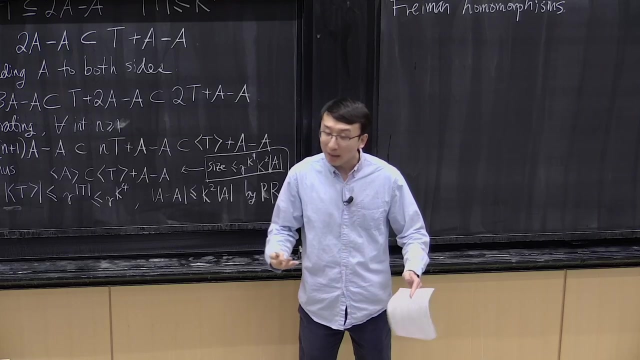 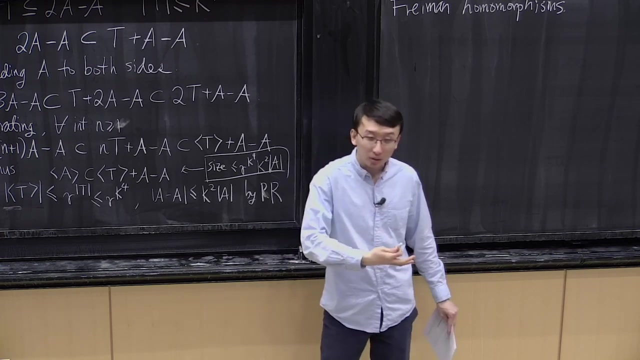 combinatorics, I need to introduce the notion of Freiman homomorphisms. So one of the central philosophies across mathematics is that if you want to study objects, you should try to understand maps between objects and understand properties that are preserved under those maps. 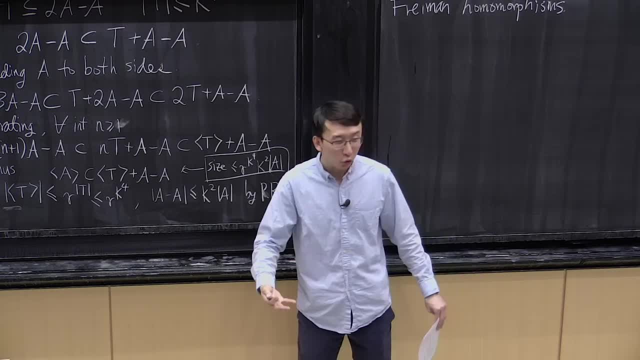 So if you want to study groups, I don't really care how you label your group elements by 1,, 2,, 3, or A, B, C. What I care about is the relationships, And those are the data That I care about. 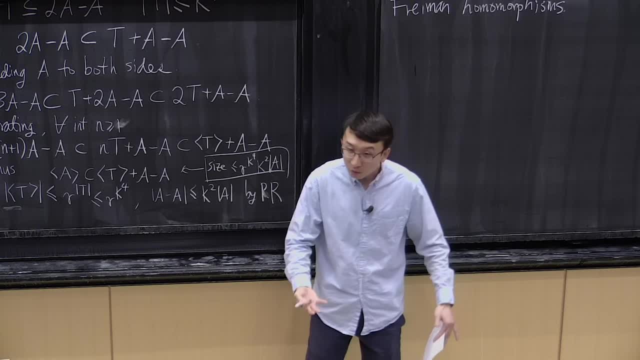 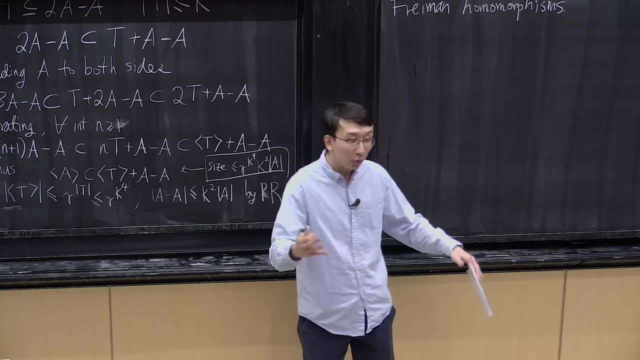 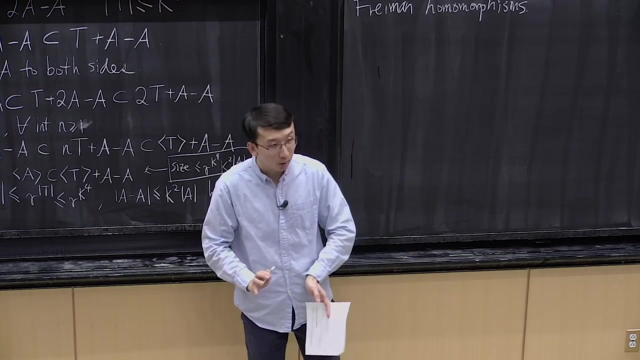 And then, of course, then you have concepts like group homomorphisms, group isomorphisms, that preserve all the relevant data. Similarly in any other area in geometry, you have manifolds. You understand not specifically how they embed into space, but what are the intrinsic properties? 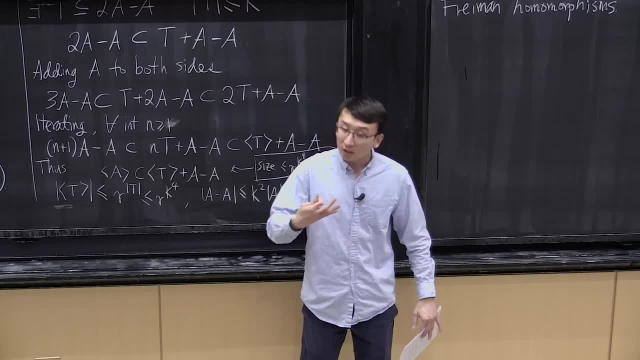 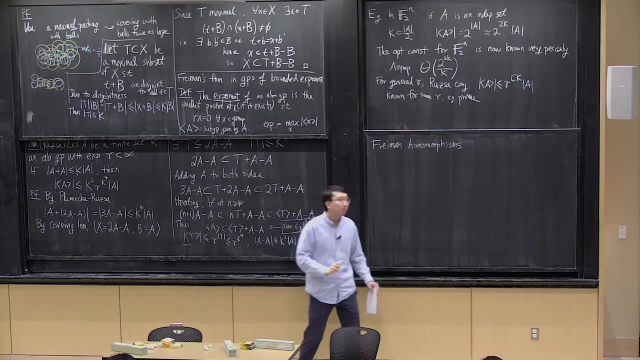 So we would like to understand what are the intrinsic properties of a subset of an abelian group that we care about for the purpose of additive combinatorics and specifically for Freiman's theorem. And what we care about is what kinds of additive relationships are preserved. 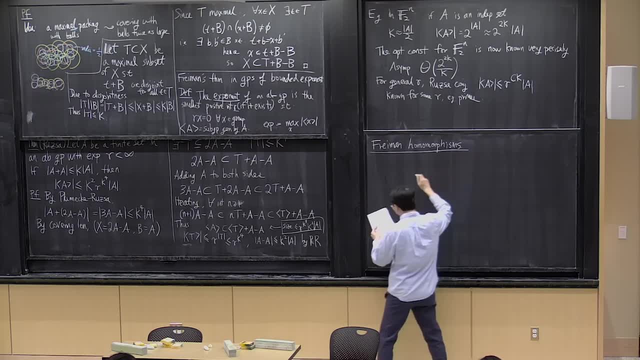 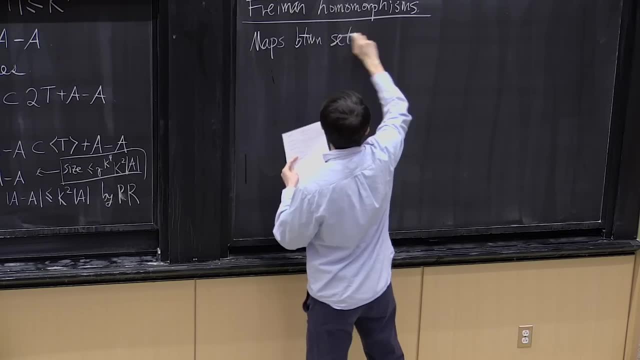 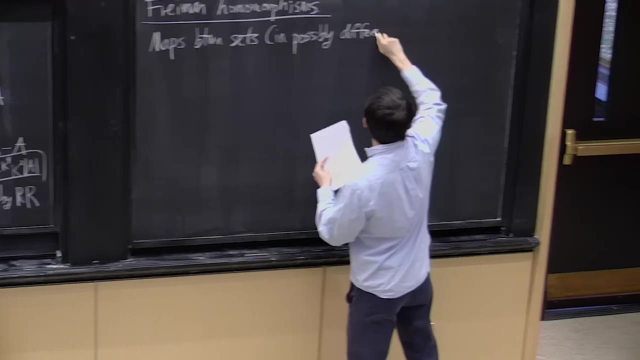 And Freiman's homomorphisms capture that notion. So, roughly speaking, we would like to understand maps between sets in possibly different groups, in possibly different abelian groups that preserve these sets. So, roughly speaking, we would like to understand maps between sets in possibly different abelian. 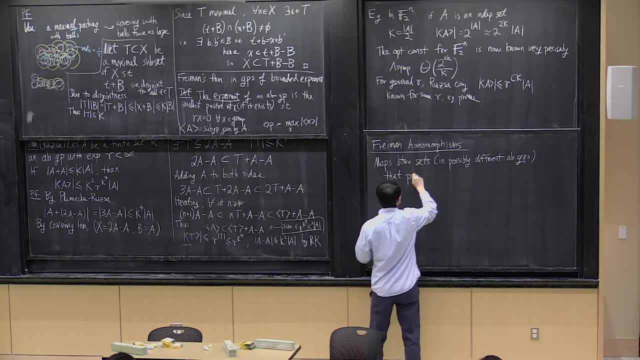 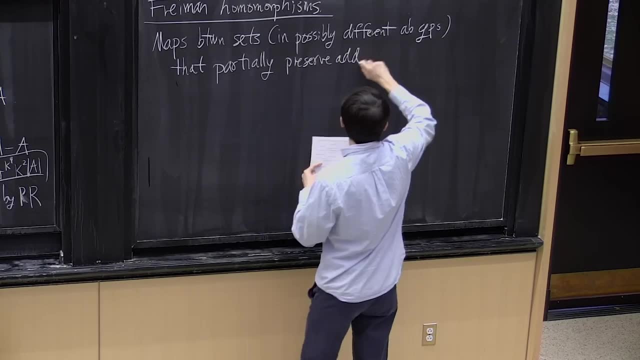 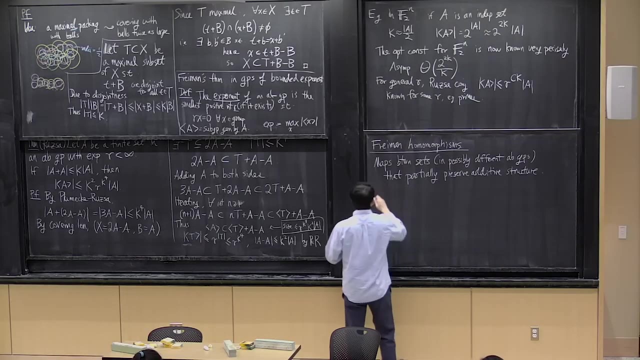 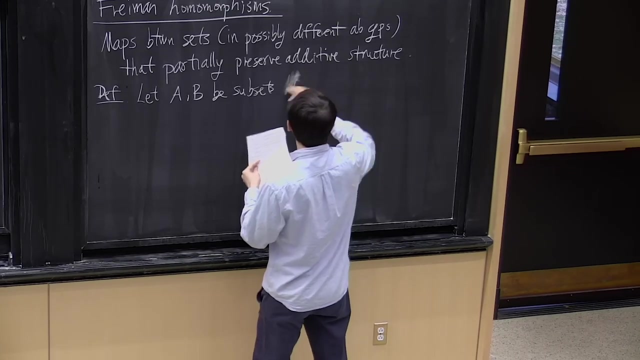 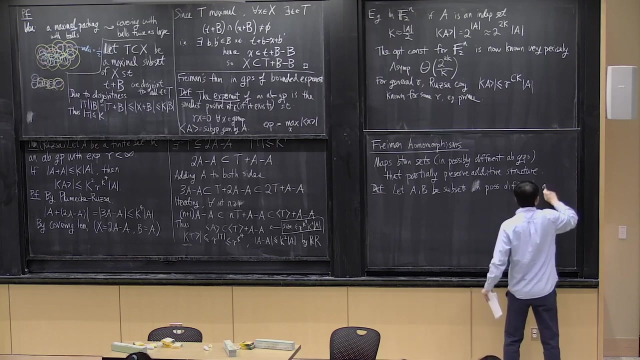 groups that preserve these sets That are preserved in a set. preserve but only partially preserve additive structure. So here's a definition. Suppose we have A and B and their subsets between subsets in possibly different abelian groups Could be the same but possibly different. 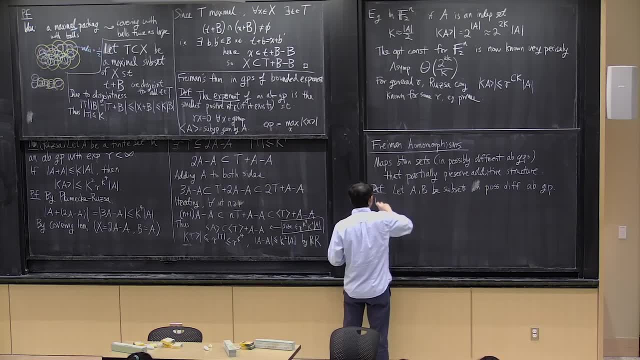 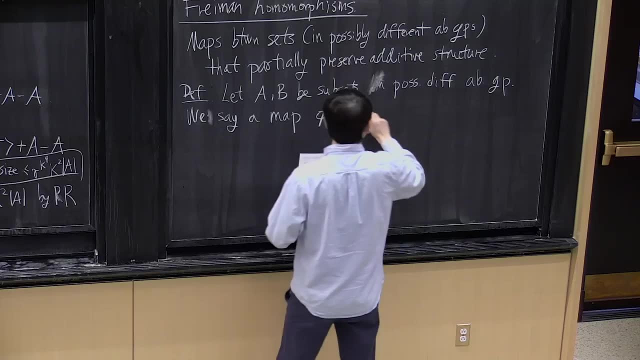 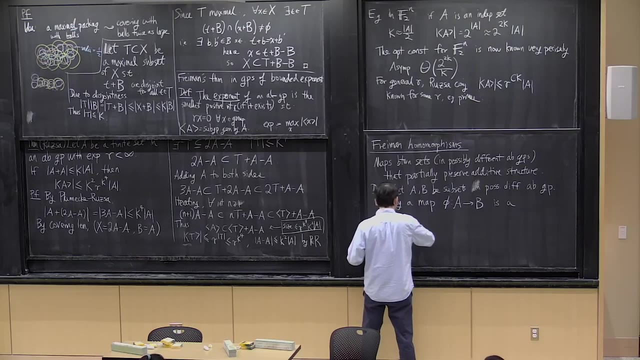 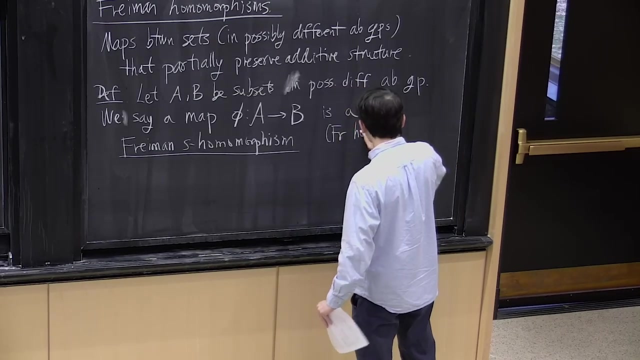 And everything's written under addition as usual. So we say that a map phi from A to B is a Freiman S-homomorphism. So that's the term: Freiman S-homomorphism, Sometimes also Freiman homomorphism of order S. 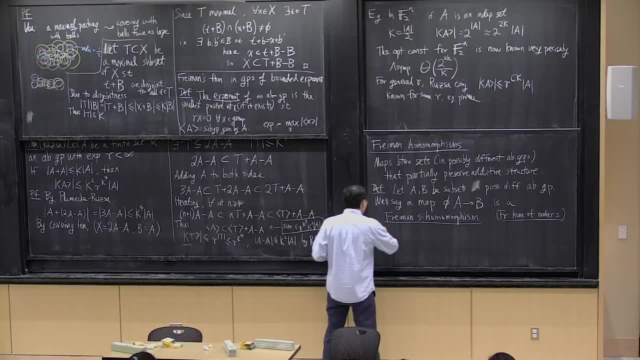 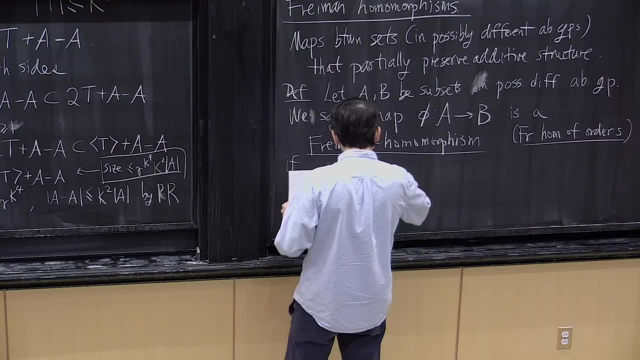 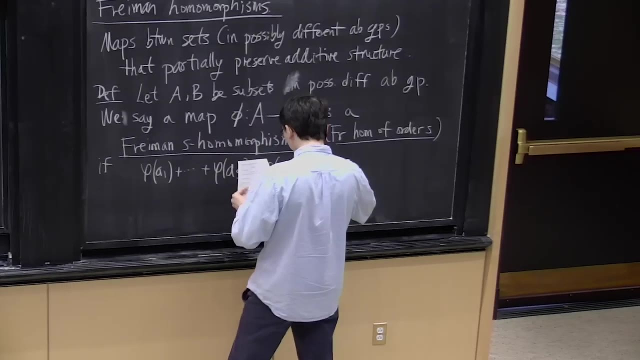 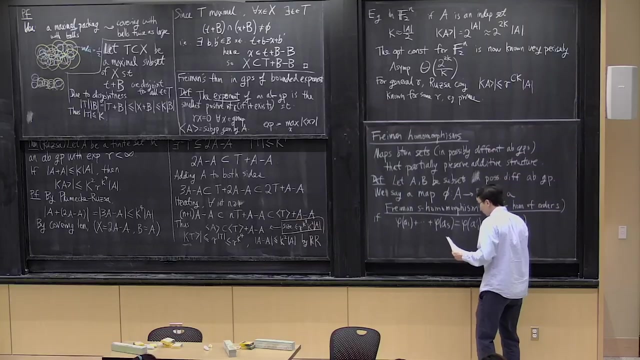 So that's equivalently- I can call it that as well- If the following holds: if we have the equation phi of A plus B- OK, plus da-da-da plus phi of a sub s equal to phi of a prime 1 plus da-da-da plus phi of a prime s. 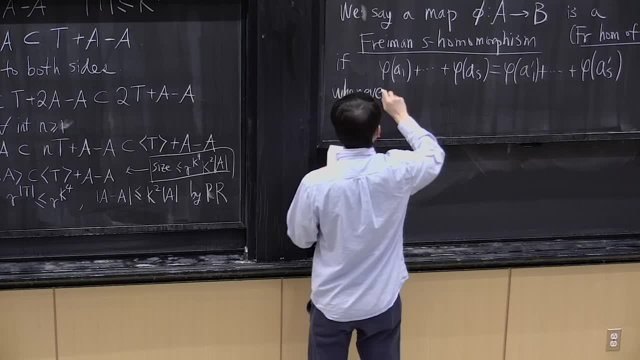 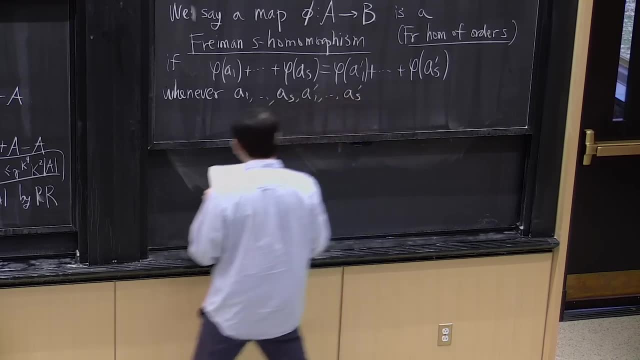 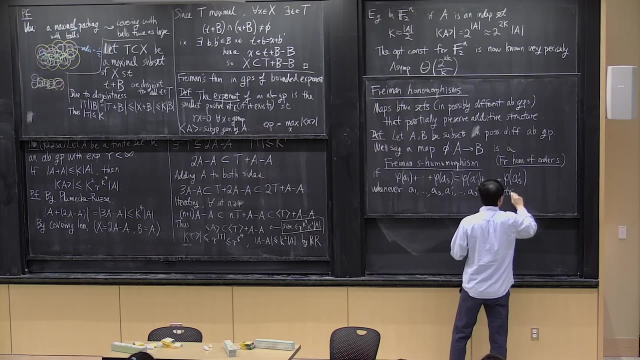 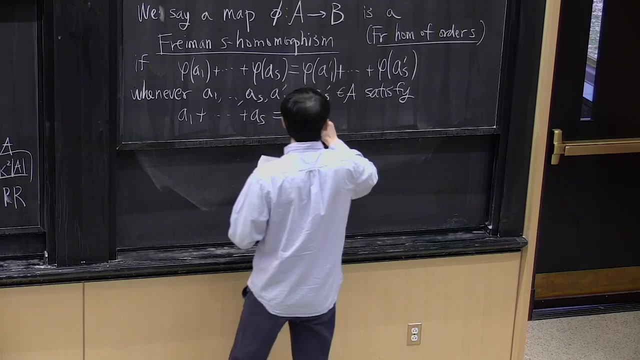 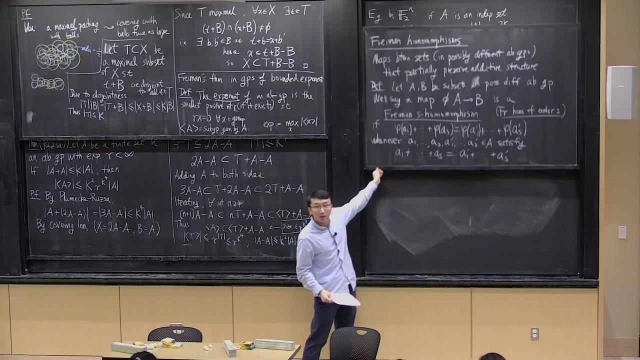 Whenever a through a s, a prime through a s prime, so a1 prime through a s prime satisfy the equation a1 plus da-da-da plus a s equal to a1 prime plus da-da-da plus a s prime. So that's the definition of a Freiman-S homomorphism. 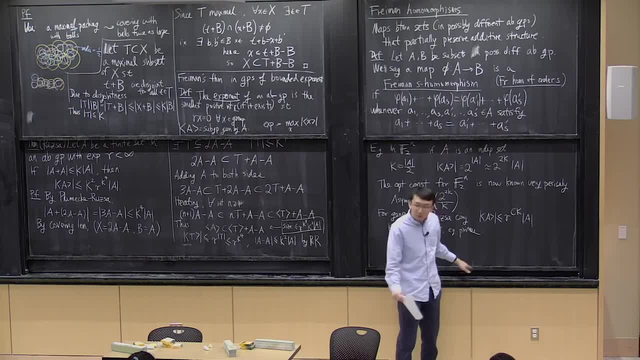 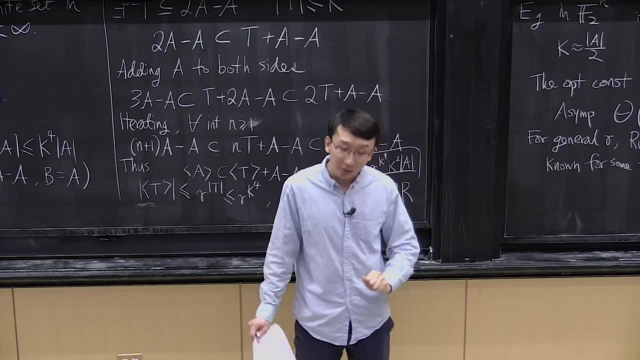 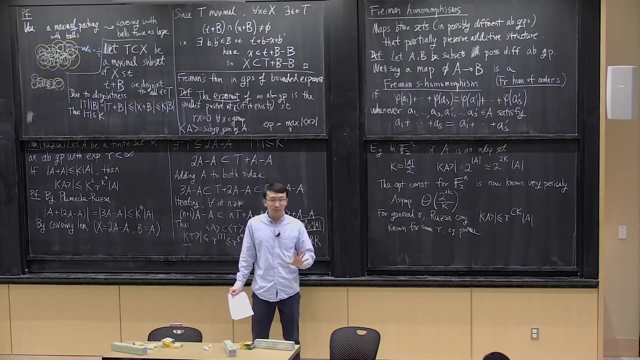 It should remind you Of the definition of a group homomorphism which completely preserves additive structure, let's say, between abelian groups And for Freiman homomorphisms, I'm only asking it to partially preserve additive structure. So the point here is that if I only care about, let's say, 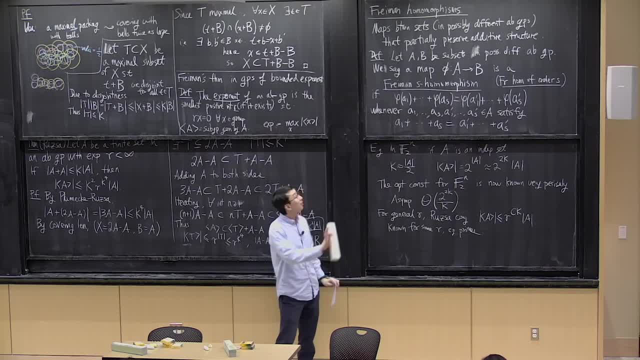 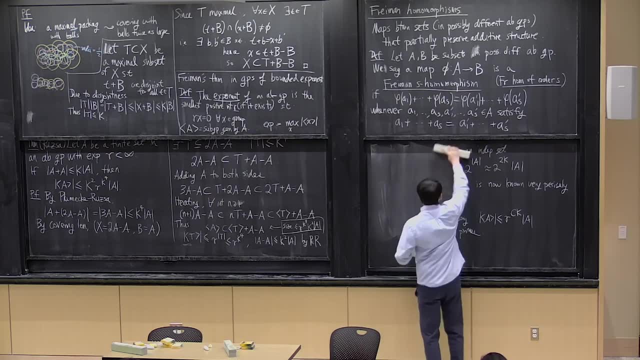 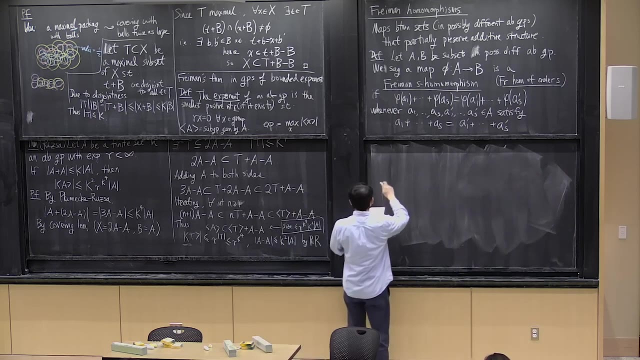 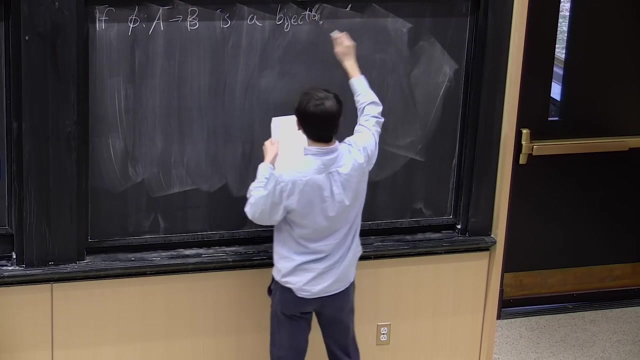 pairwise sums. if that's the only data I care about, then Freiman-S homomorphisms preserve that data. OK, To give you some. OK. so one more thing: if a, so if phi from a to b is furthermore a bijection. 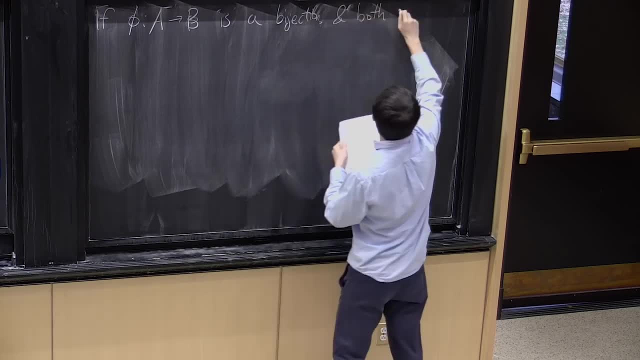 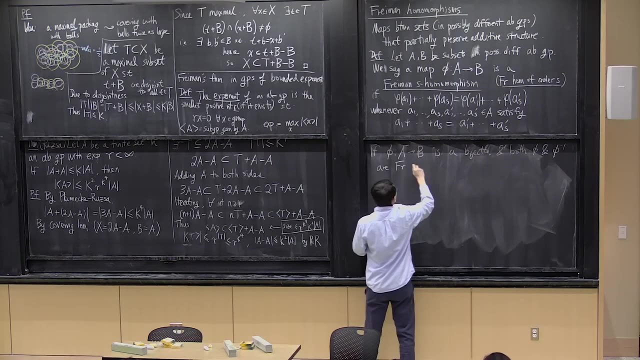 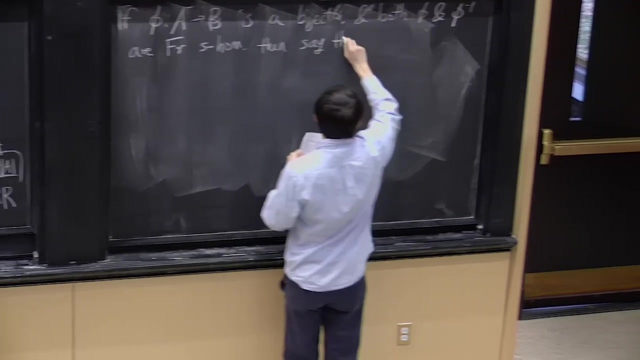 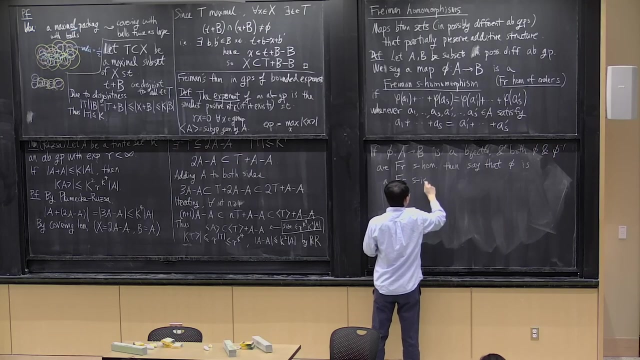 and both phi and phi inverse. If phi and phi inverse are Freiman-S homomorphisms, then we say that phi is a Freiman-S isomorphism. OK, So it's not enough just to be a bijection, but it's a bijection. 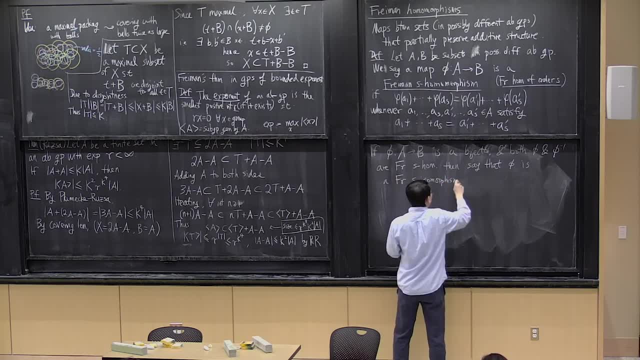 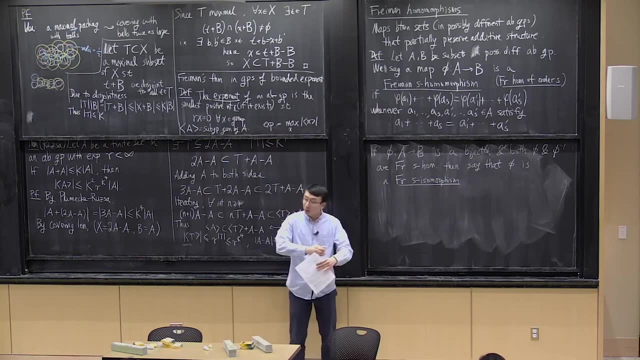 And both the forward and the inward are a bijection. So it's not enough just to be a bijection, but it's a bijection, And both the forward and the inward are a bijection. OK, So the inverse maps are Freiman-S Freiman homomorphisms. 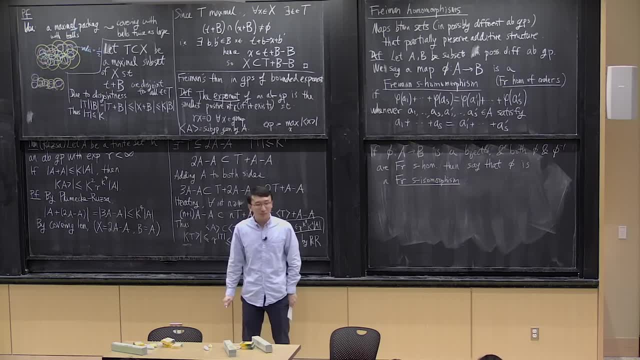 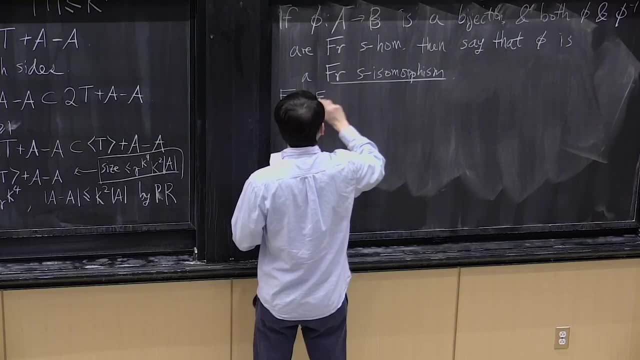 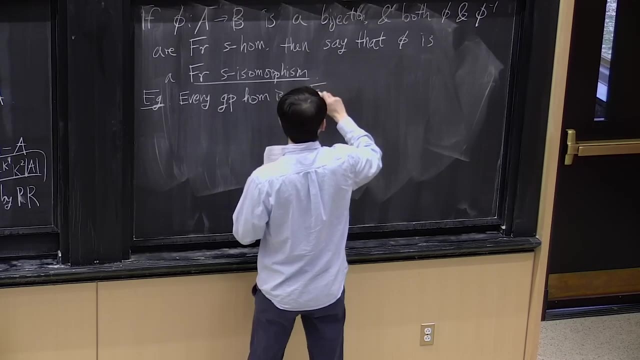 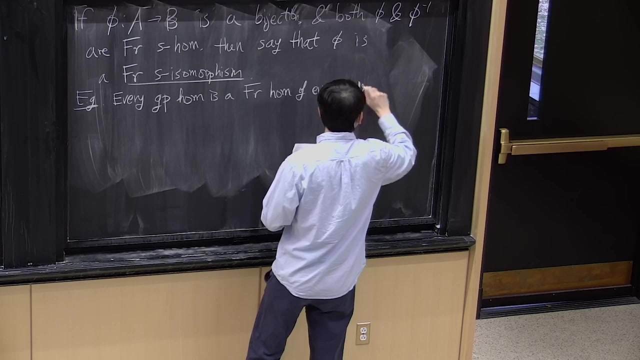 So these are the definitions we're going to use. Let me give you some examples. So every group homomorphism is a Freiman homomorphism of every order. So group homomorphisms preserve all additive structure And Freiman homomorphisms only partially. 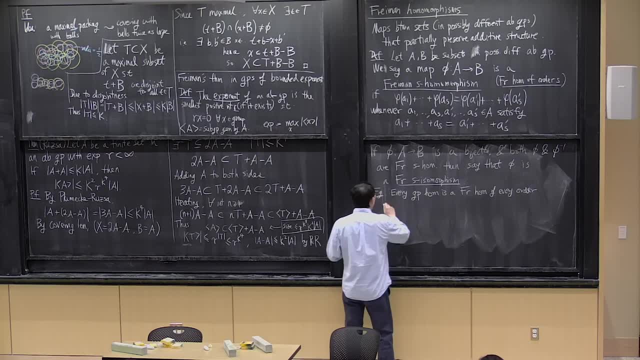 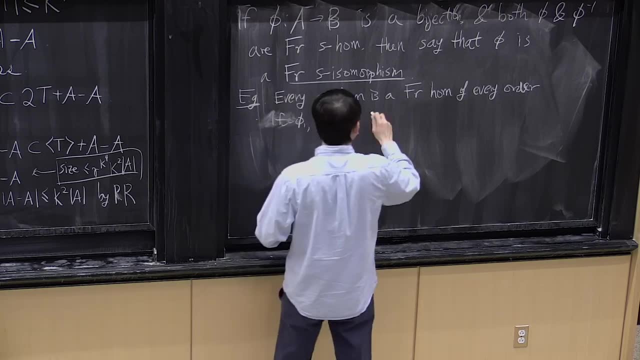 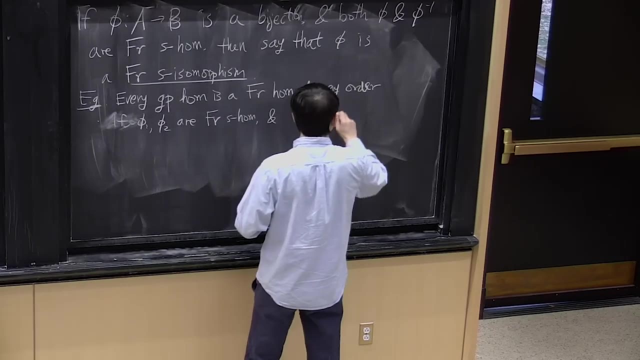 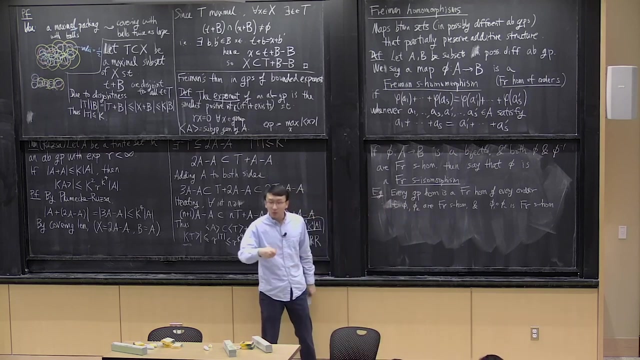 preserve additive structure, A composition. so if phi 1 and phi 2 are Freiman-S homomorphisms, then phi 1 composed with phi 2 is a Freiman-S homomorphism. OK, So compositions preserve this property. 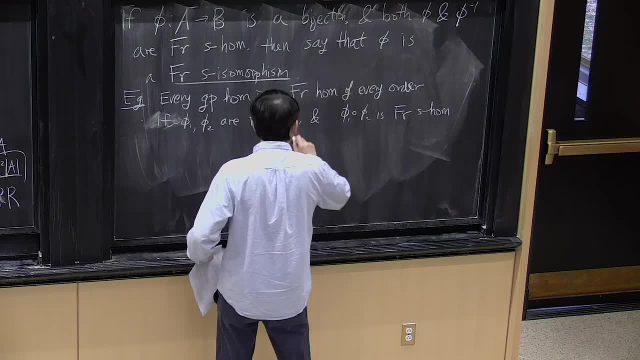 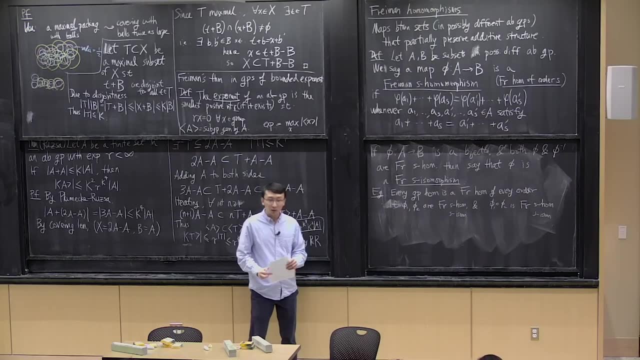 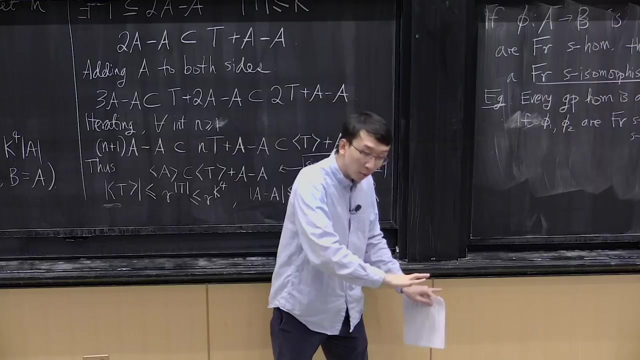 And likewise, if you have, instead of homomorphisms, if you have isomorphisms, then that's also true as well. OK, So these are straightforward things to check. So a concrete example that shows you a difference between group homomorphisms: 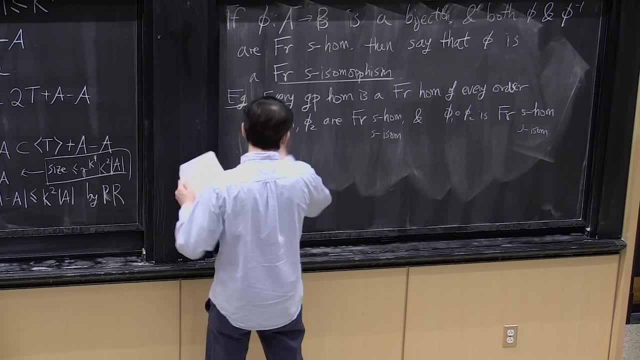 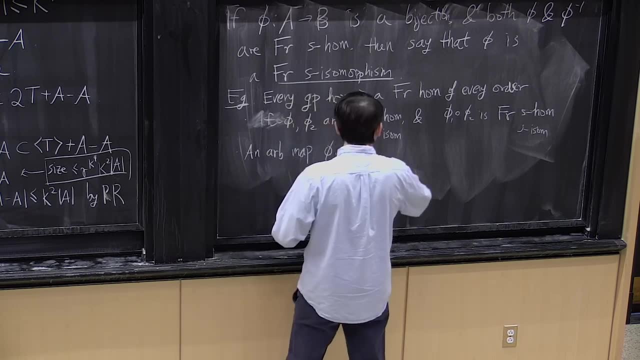 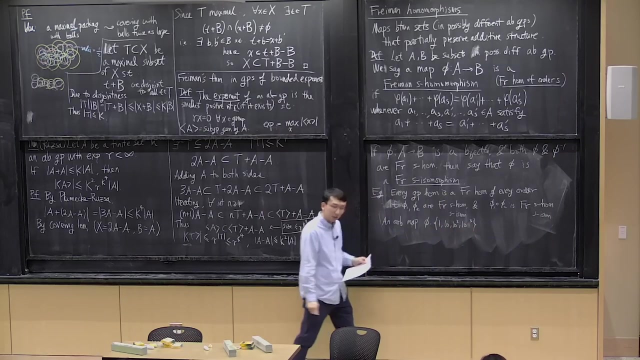 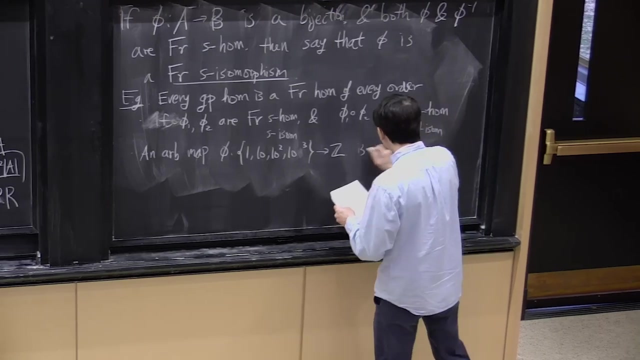 and Freiman homomorphisms is suppose you take an arbitrary map- phi 1 and phi 2, from a set that has no additive structure, So it's a four-element set has no additive structure and I map it to the integers claim: 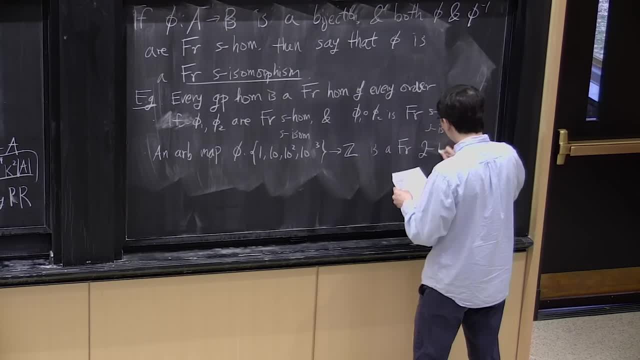 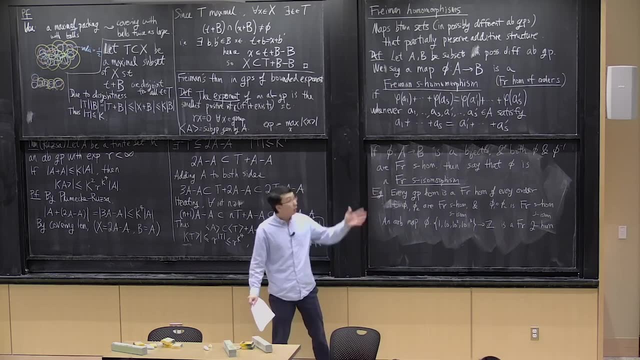 that this is a Freiman 2 homomorphism. So you can check. So you can whenever this is satisfied, but that's never non-trivially satisfied. So an arbitrary map here is a Freiman 2 homomorphism. 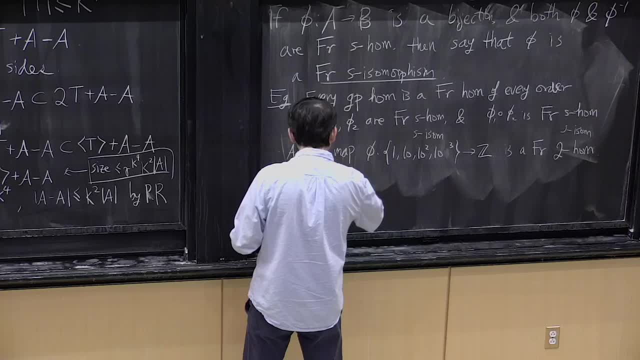 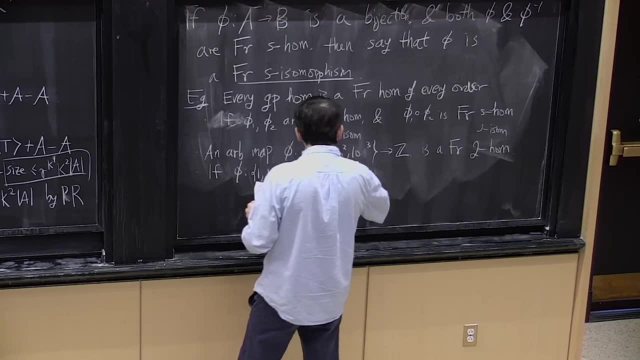 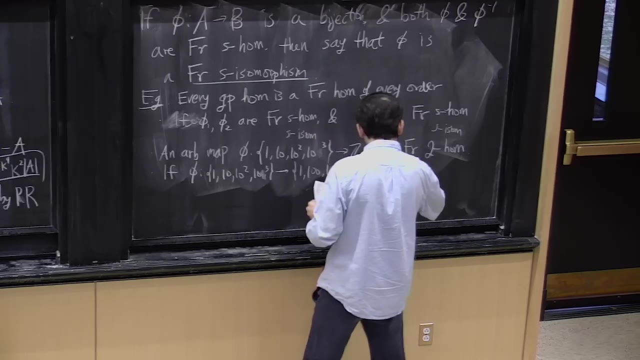 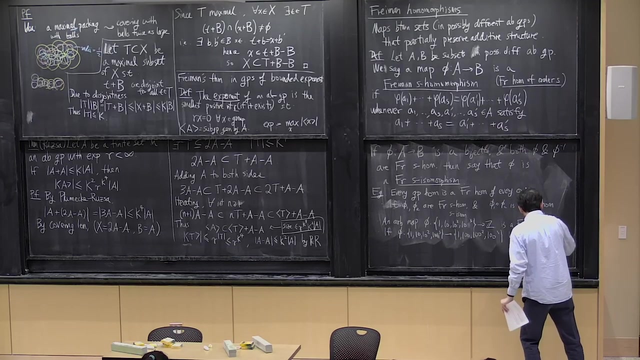 And if, furthermore, so, if you have, let's say, a bijection between two sets, both having no additive structure, if it's a bijection, OK. If it's a bijection, then it's a Freiman isomorphism of here. 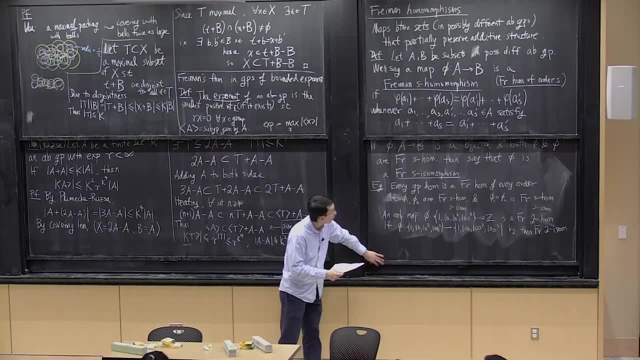 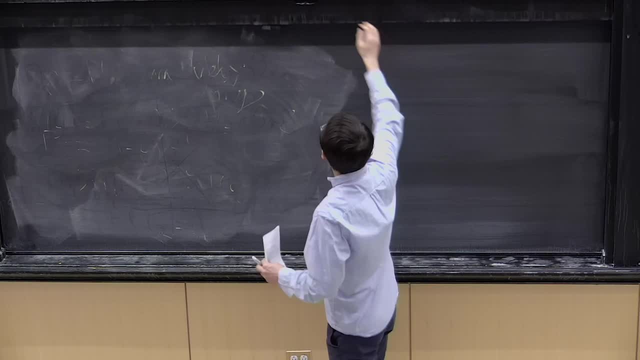 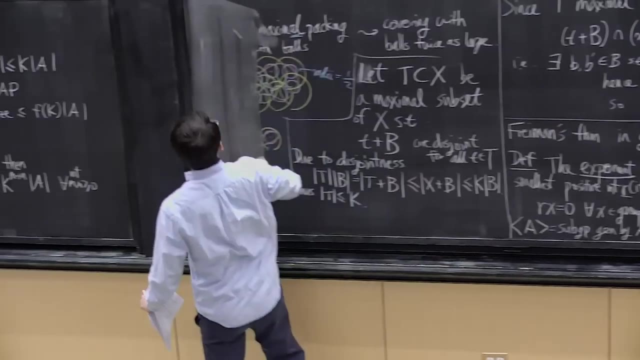 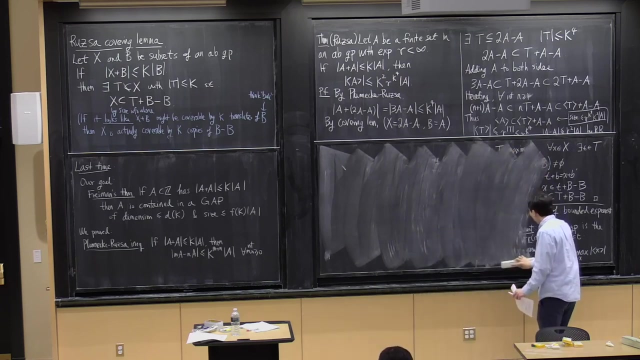 order 2.. Let me give you a few more examples. So in you know When you look, When you look at homomorphisms between finite groups. so you know that if you have a homomorphism and it's also a bijection, then it's an isomorphism. 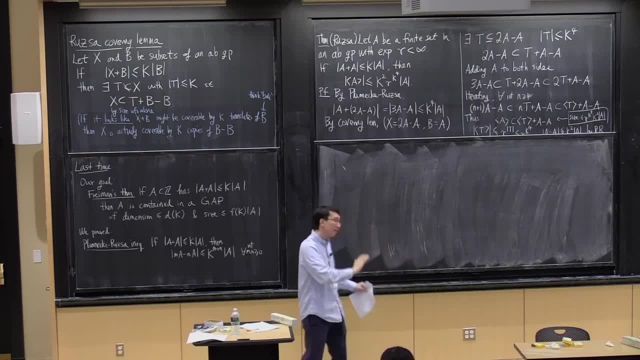 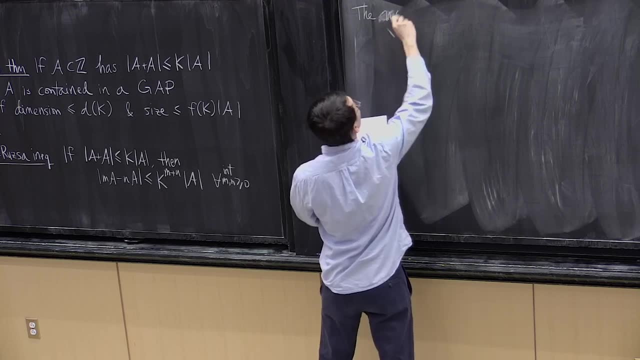 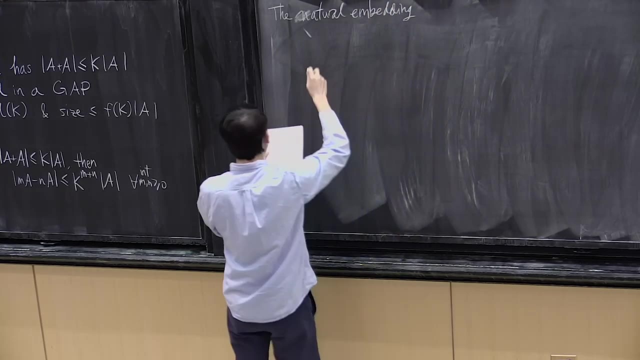 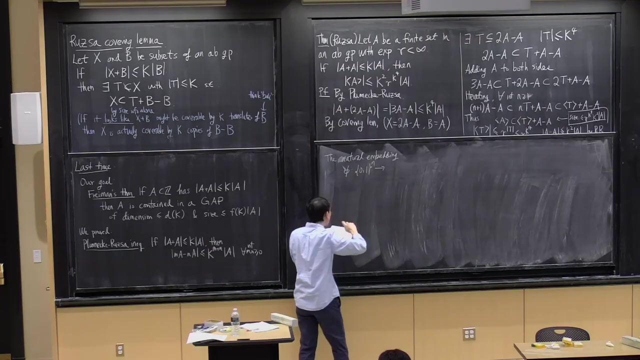 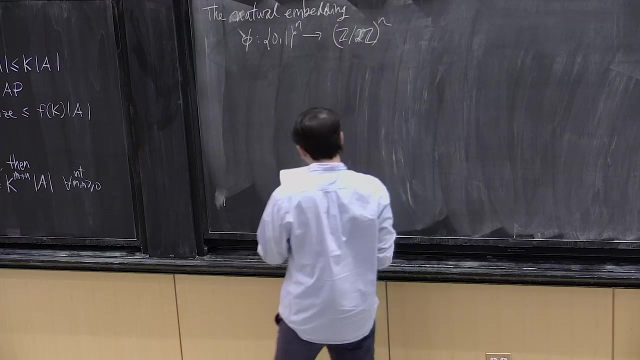 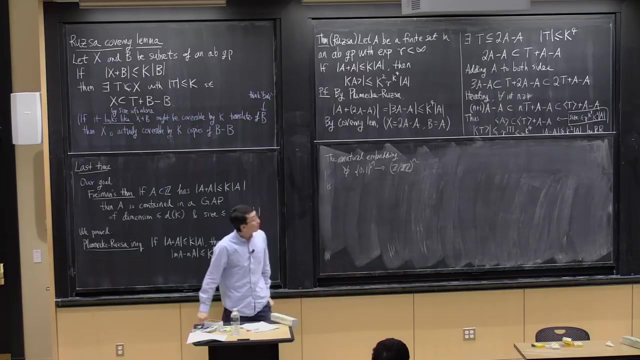 But that's not true for this notion of homomorphisms. So the natural embedding, So the natural embedding that sends the Boolean cube to The Boolean cube, are viewed as Z mod 2 to the n. So is OK. so what's happening here? 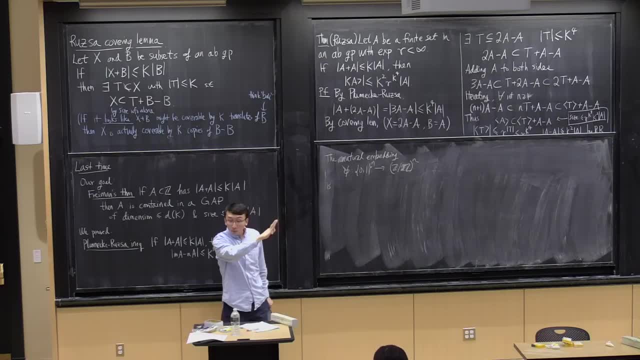 This is a part of a group homomorphism, Let's see. OK, So if you look at Z to the n, and I do mod 2, and I restrict to this Boolean cube, that's the group homomorphism if I view this. 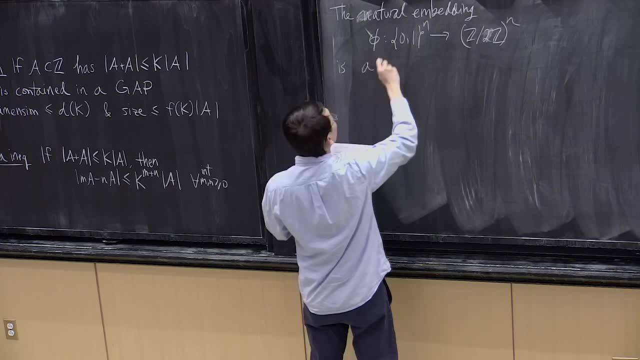 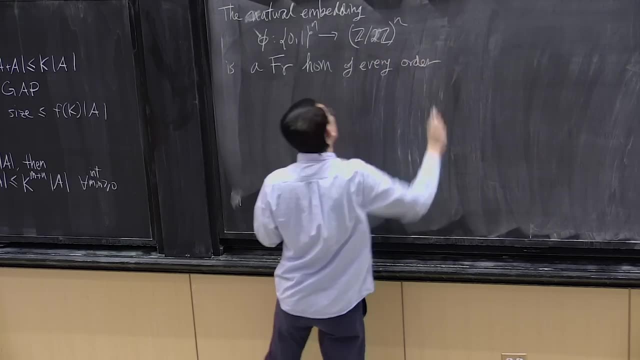 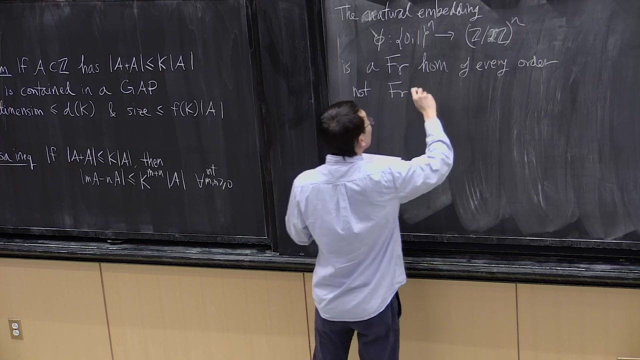 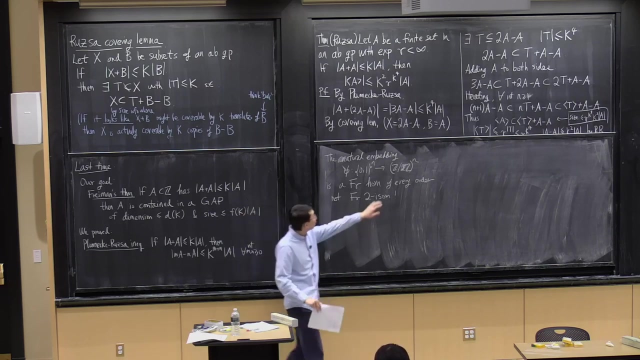 as a subset of a bigger group. So it is a Freiman homomorphism of every order And it's bijective, But it is not a Freiman 2 isomorphism. OK, So it's a Freiman 2 isomorphism because you have additive. 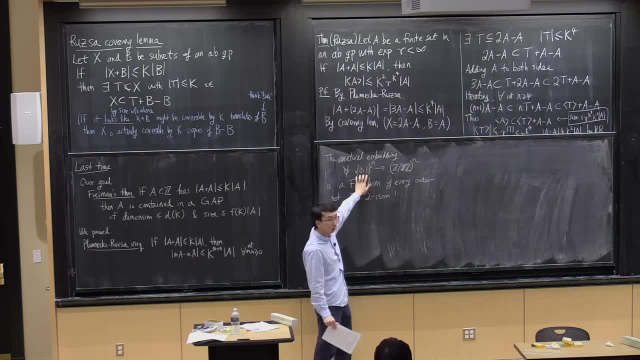 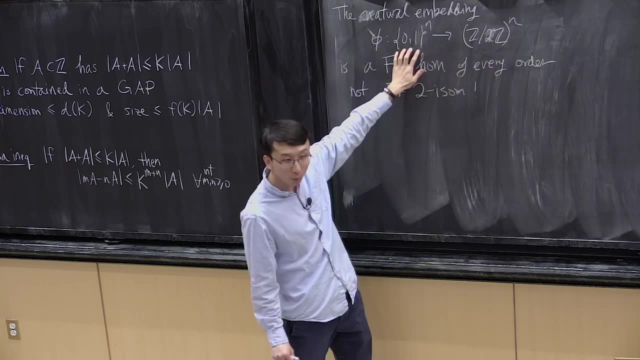 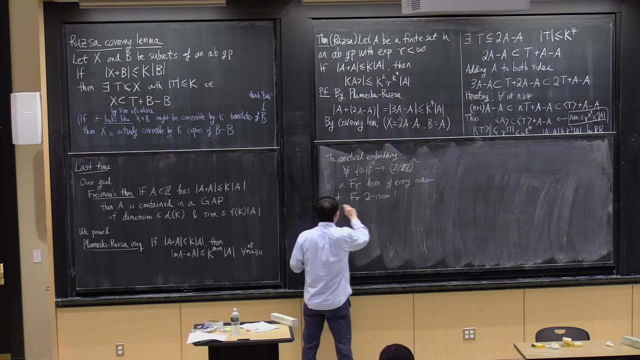 relations here that are not present over here. So if you read the definition, the inverse map, there are some additive relations here that are not preserved if you pull back. So here's another example that will be more relevant to our subsequent discussion: The mod n map. 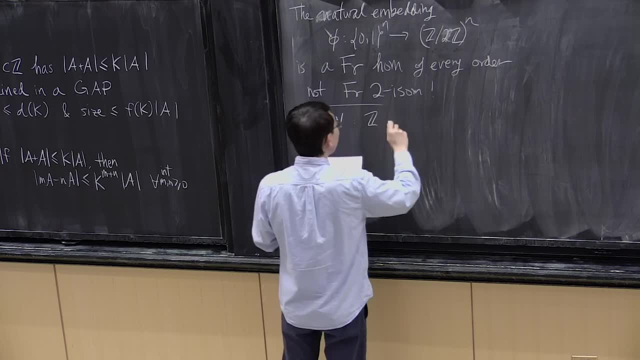 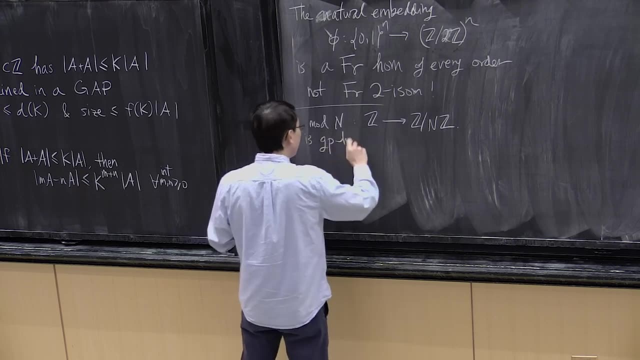 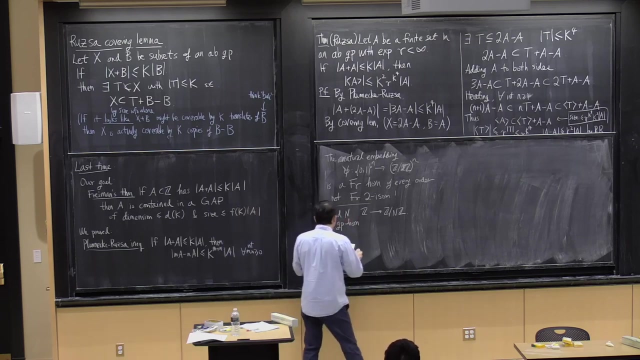 So the mod n map, which sends Z to Z, mod n, So this is a group homomorphism, So hence it's a Freiman homomorphism of every order, But it's not OK. so if you look at this map and even if I 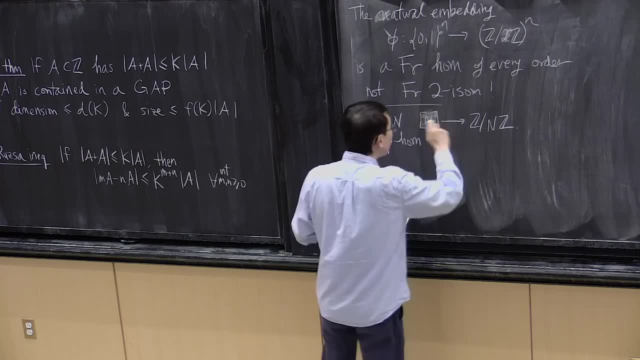 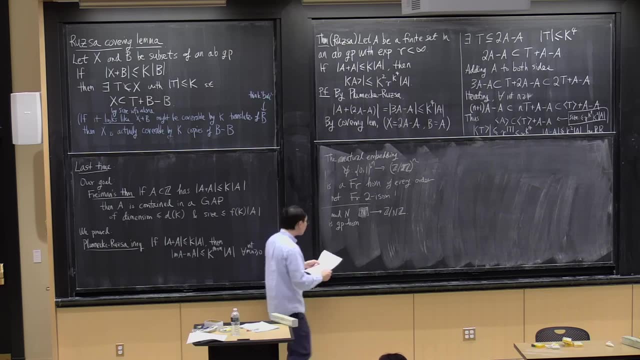 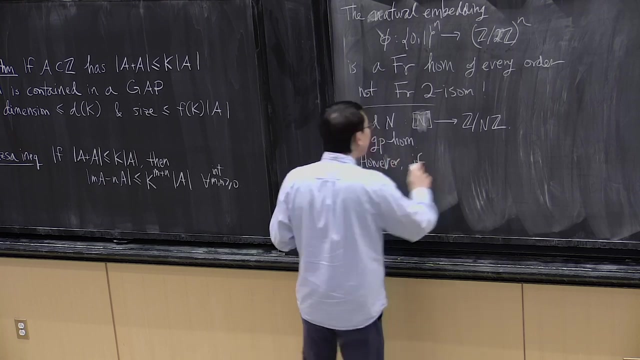 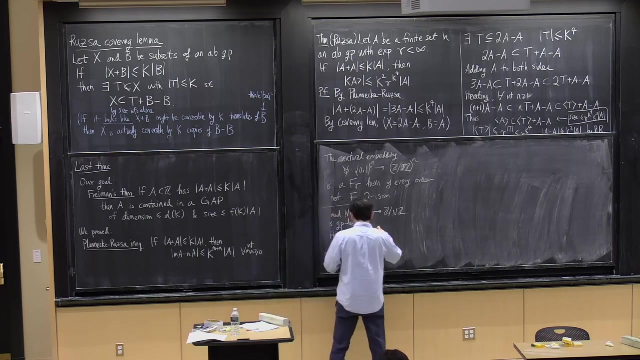 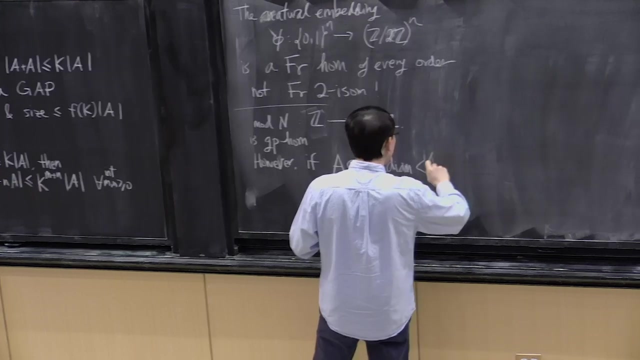 restrict to here. OK, so it's not an isofreiman, isofreiman isomorphism just like earlier, However. so if OK. so let me go back to Z again. So if A is a subset of integers with diameter less than n, 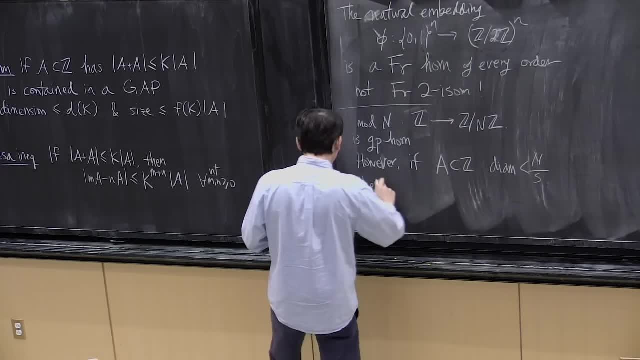 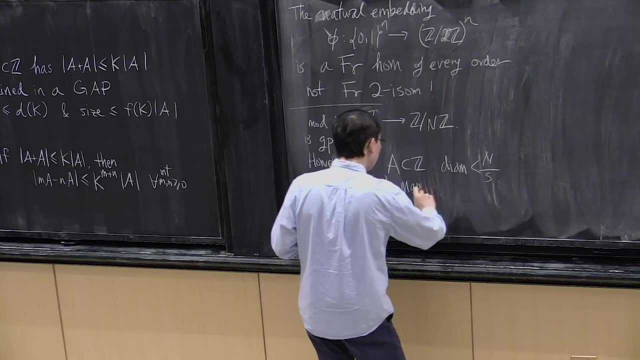 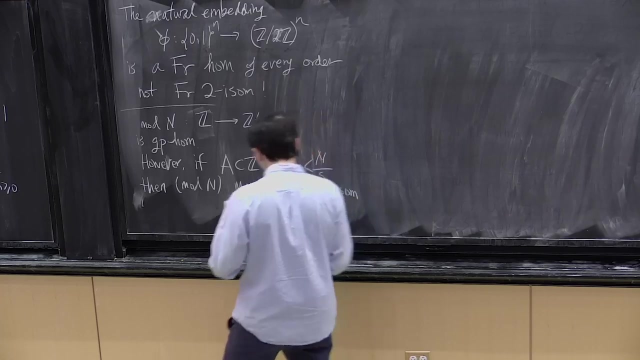 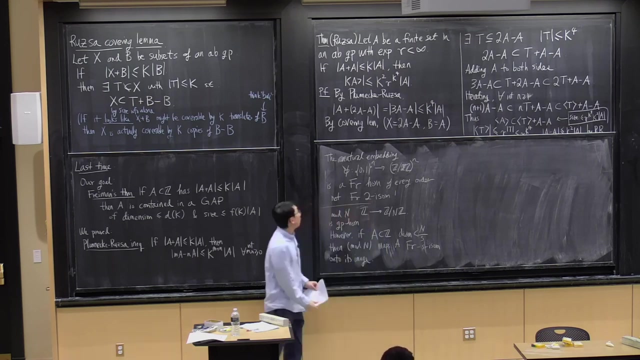 over S then. So this map, mod n, maps a Freiman S isomorphically onto its image. So even though mod n, restricted to 1 through n, is not a Freiman isomorphism, of order 2,, if I restrict, OK. 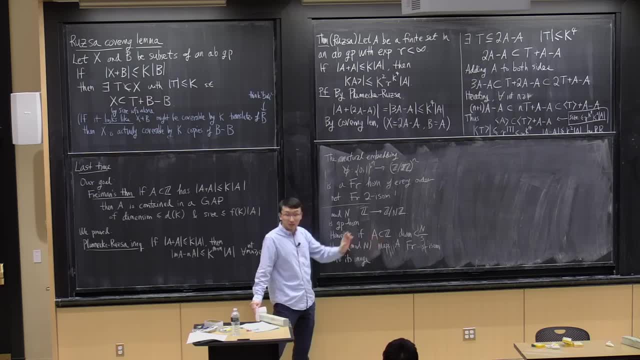 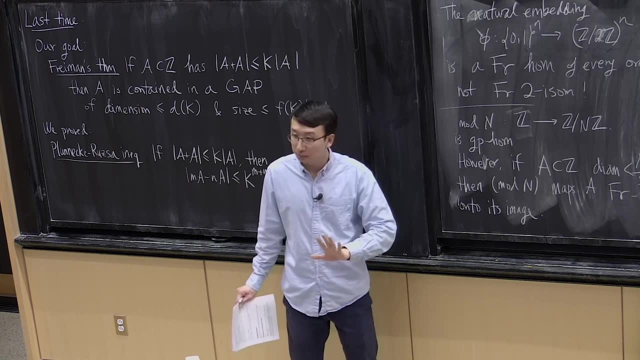 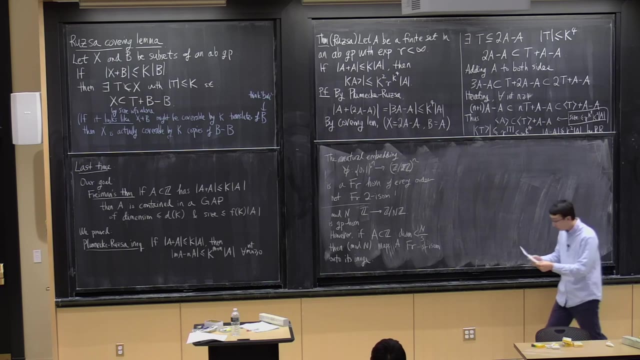 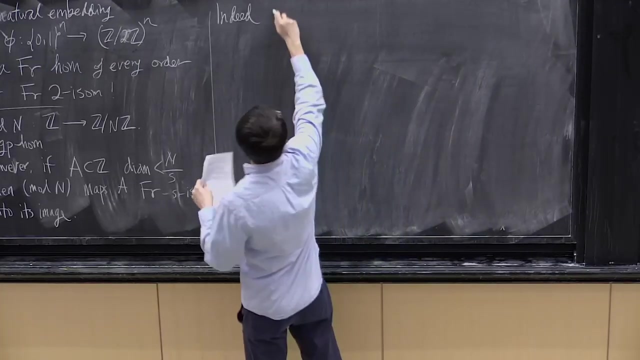 it to a subset that's, let's say, contained in some small interval, then all the additive structures are preserved. OK, so let me show you why. So this is not too hard once you get your head around the definition. So, indeed, if you have group elements A1 through As 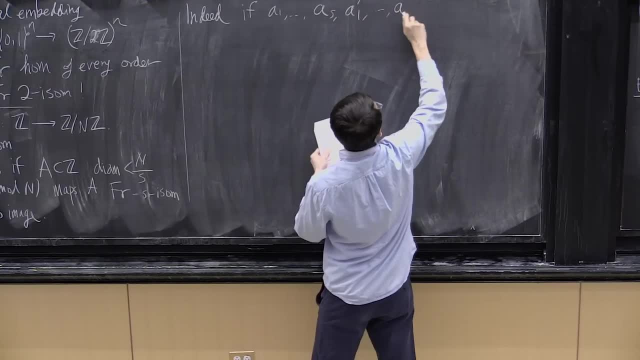 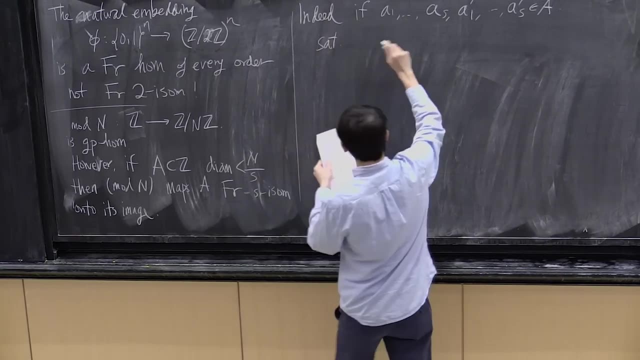 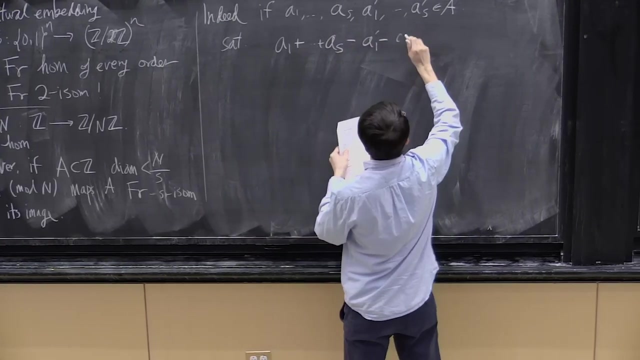 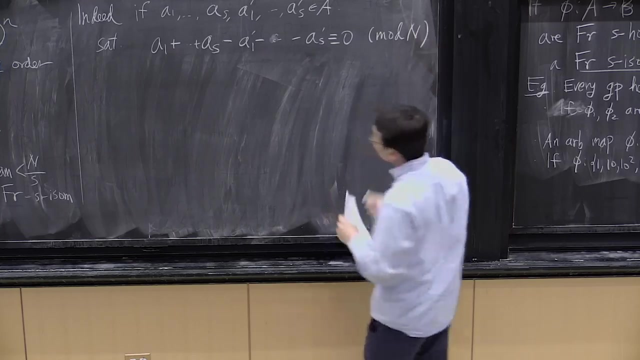 OK, OK, S, A prime 1 through A prime S And if they satisfy the equation, OK. so if they satisfy this equation. so we're trying to verify that it is a Freiman S isomorphism, namely that inverse 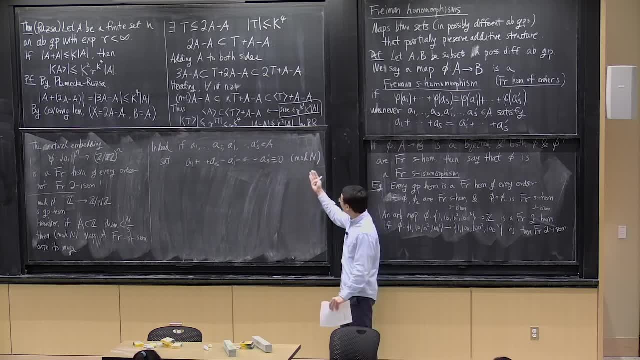 The inverse of this map is a Freiman S homomorphism. So if they satisfy this equation, so this is satisfying this additive relation. in the image in Z, mod n. then note that the left-hand side, so all of these A's, are contained in a small interval. 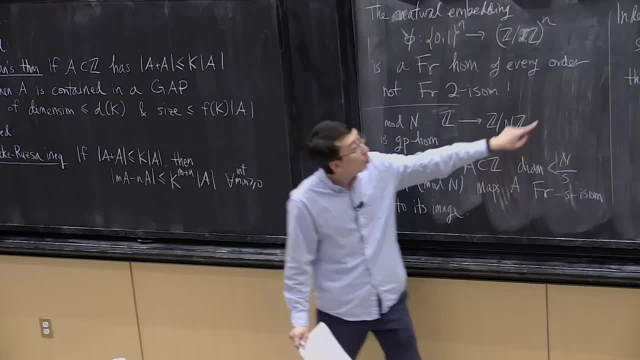 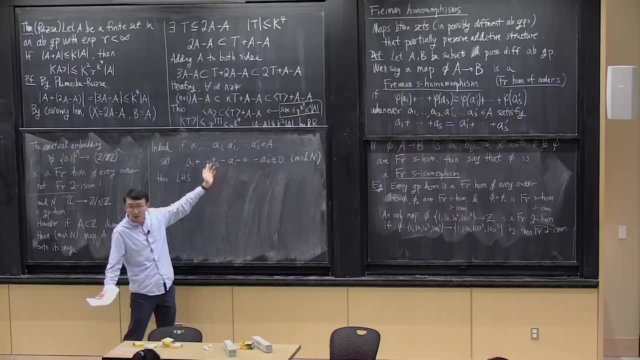 because the diameter of the set is less than n over S. So if you look at how big A1 minus A1 prime, OK, OK. OK, So A1 prime can be at most less than n over S in size. So the left-hand side in absolute value. 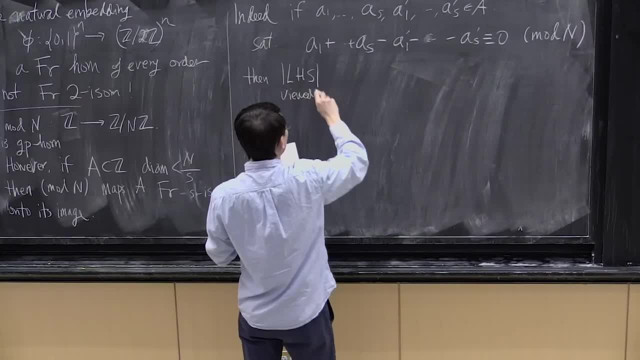 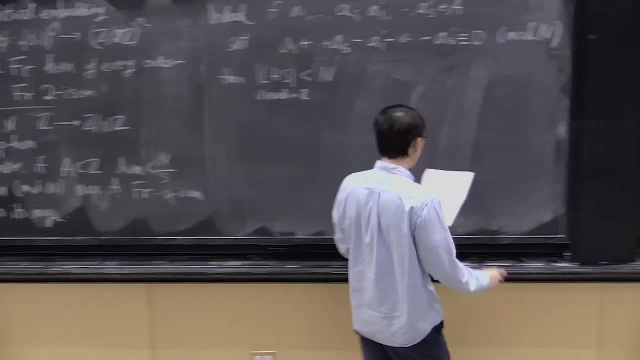 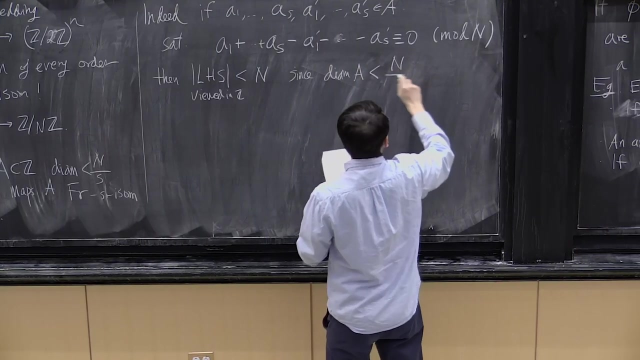 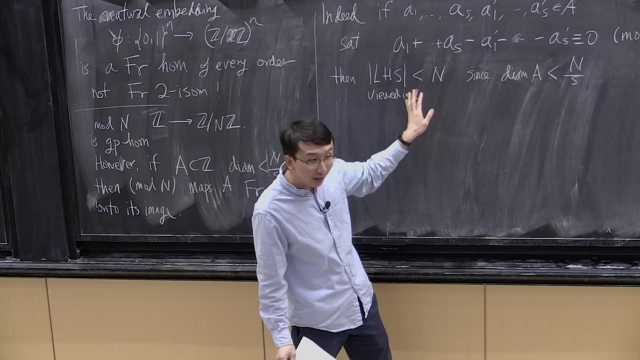 viewed as an integer. so the left-hand side is less than n in absolute value, since the diameter of A is less than n over S. So you have some number here. So you have some number here which is strictly less than n in absolute value and is 0 mod n. 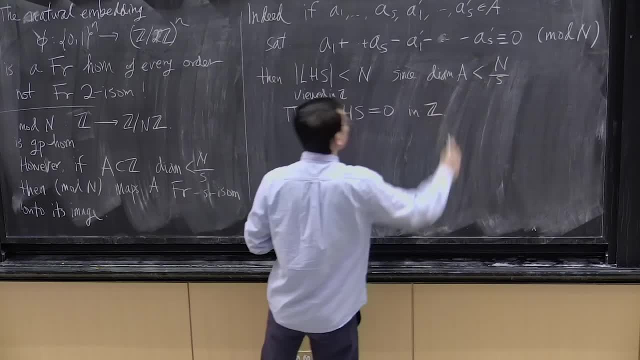 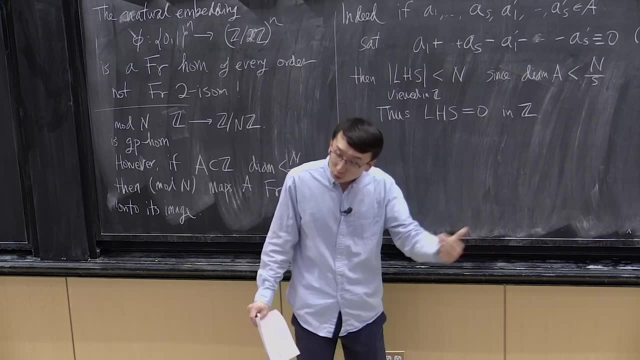 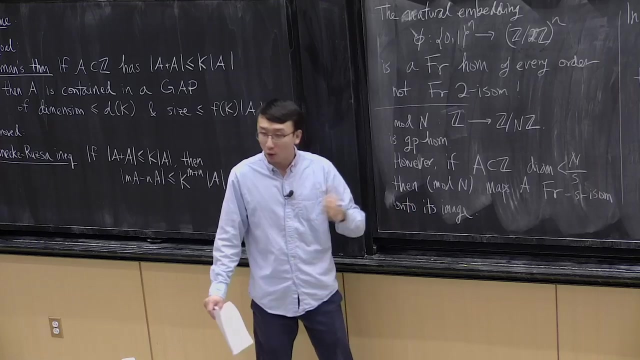 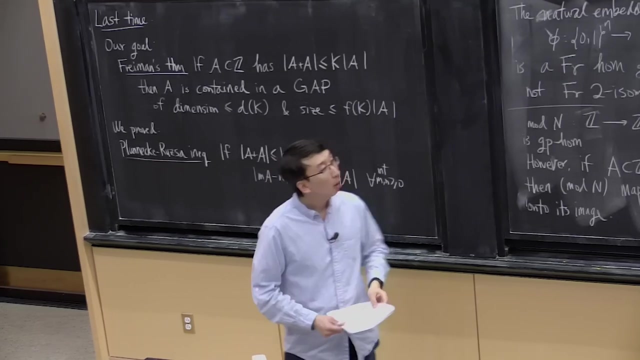 So it must be actually equal to 0 as a number, as an integer. So this verifies that the additive relations up to S-y sums are preserved under the mod n map. if you restrict to a small interval, All right. Any questions so far? 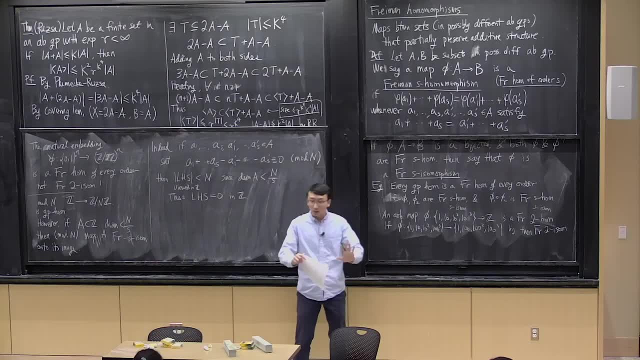 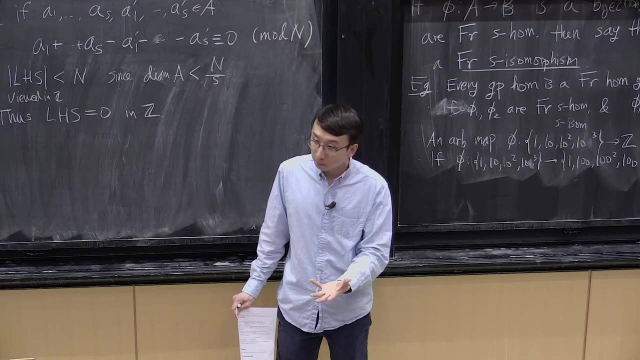 So in additive combinatorics, we are trying to understand specific additive properties And the notion of Freiman homomorphisms and Freiman isomorphism capture, what specific properties we need to study and what are the maps that preserve those properties. And the next thing we will do is to understand this. 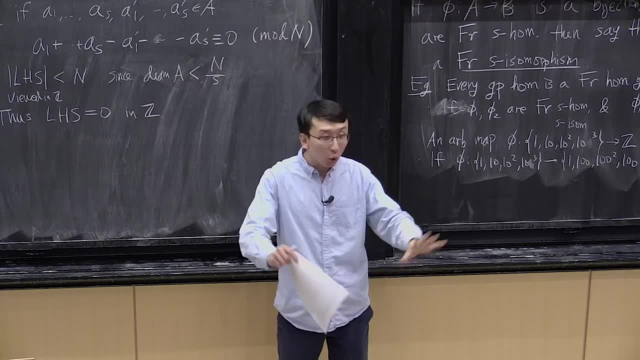 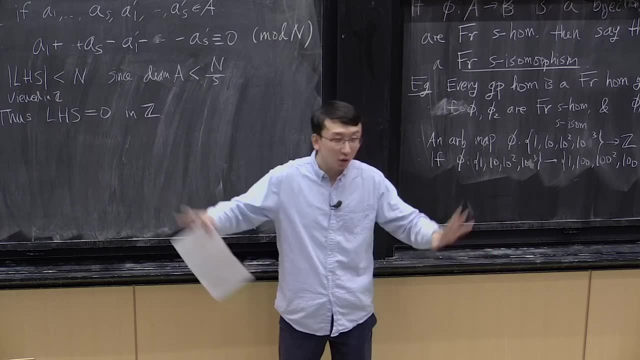 model lemma, the modeling lemma. that tells us that if you start with the set A with small doubling, initially A may be very much spread out in the integers. It may have very large elements, very small elements, very spread out. But if A has small doubling properties, 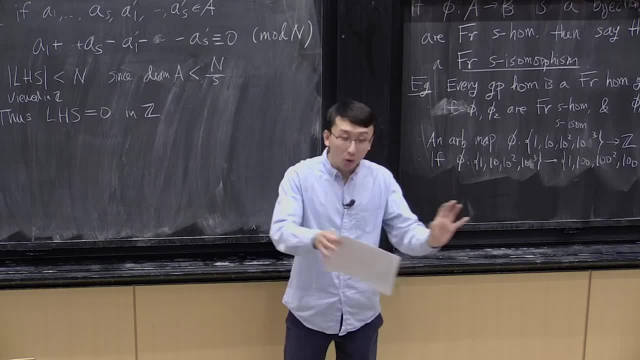 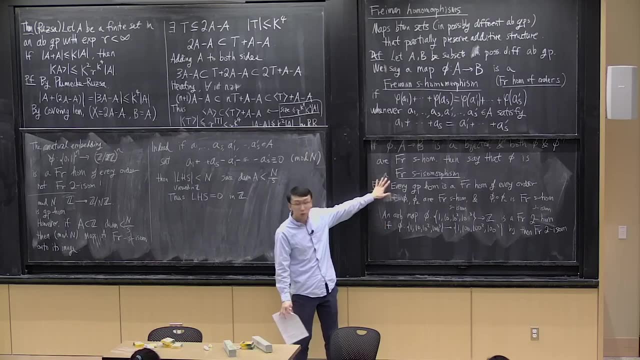 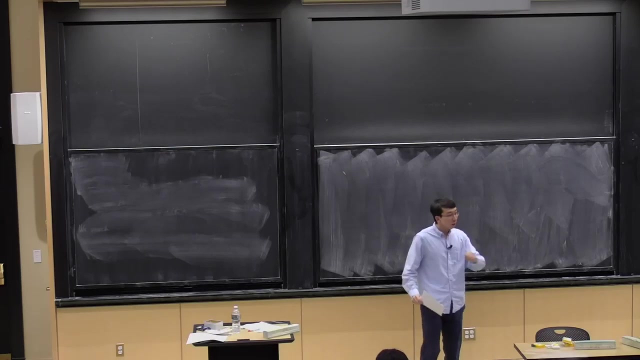 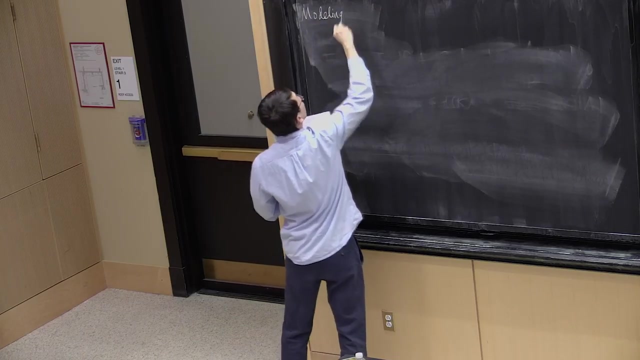 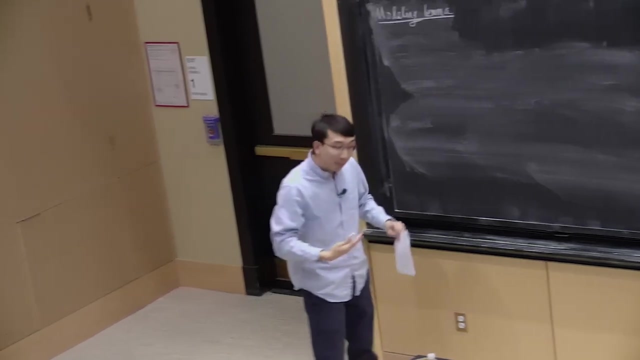 then I can model A by a small inside a small group, such that all the relevant data, namely relative to these Freiman homomorphisms, are preserved under this model. OK, So let's move on to the modeling lemma. The main message of the modeling lemma: 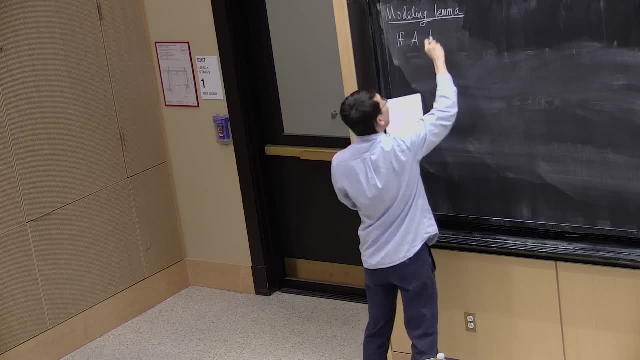 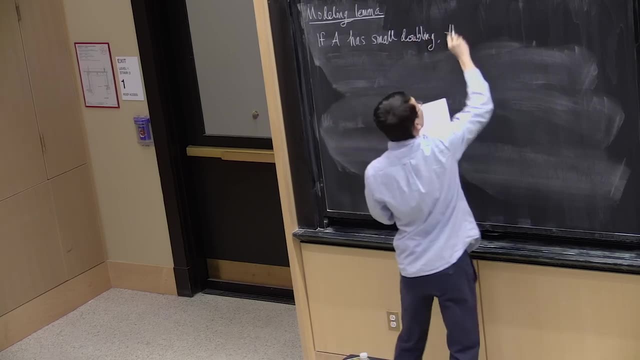 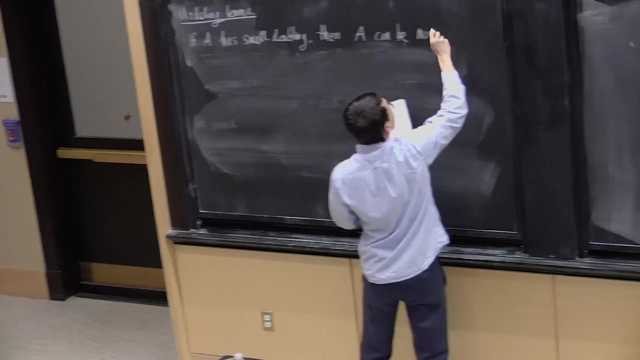 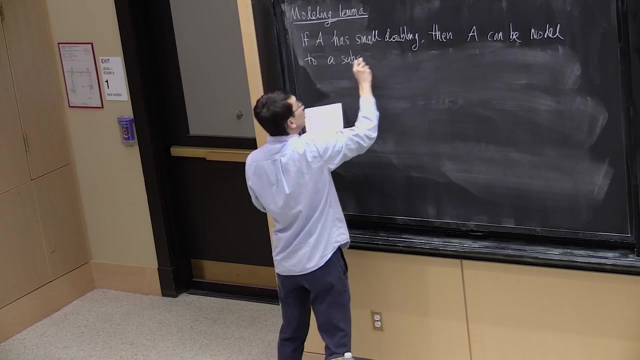 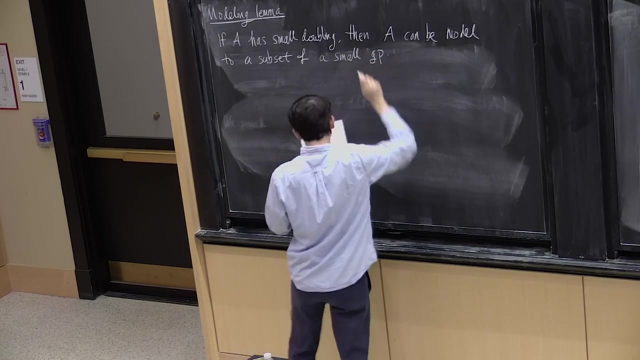 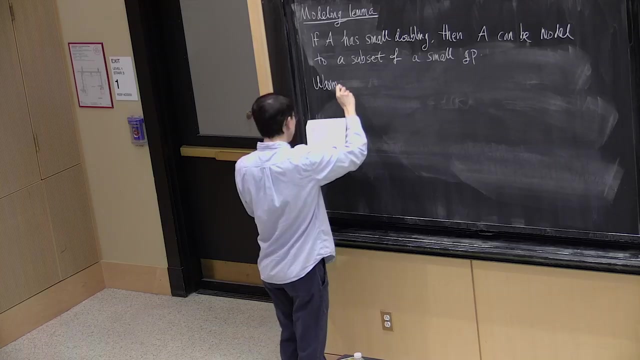 is that if A has small doubling, then A will be very much spread out. OK, A can be modeled, And here that means being Freiman isomorphic to a subset of a small group. So first, as a warm-up, let's work in the finite field model. 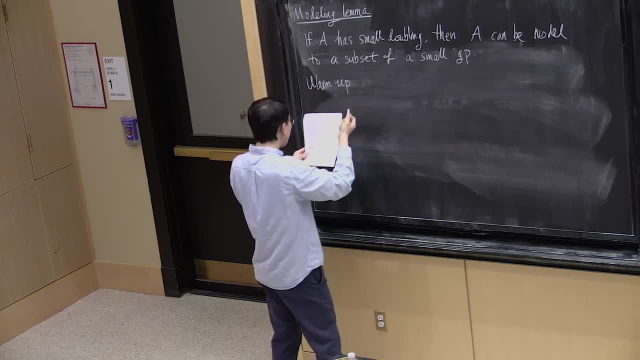 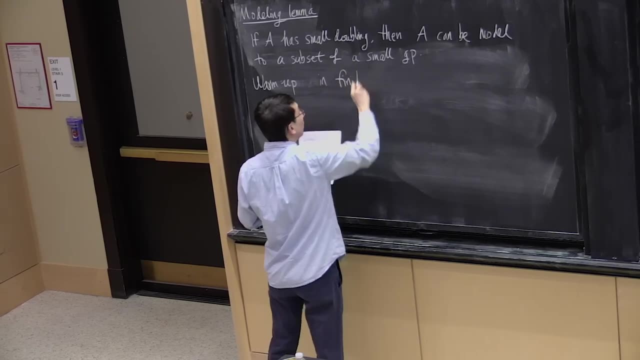 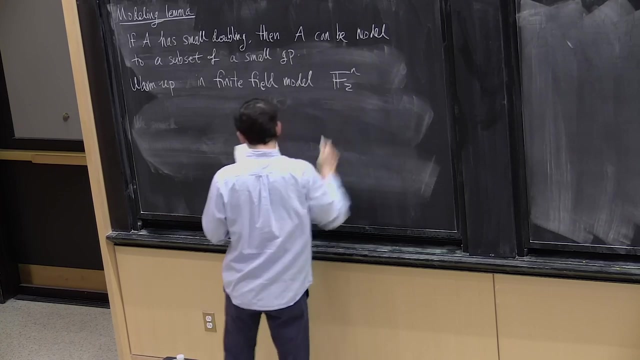 just to see what such a result looks like, And it contains most of the ideas, but it's much cleaner than in the integers. So in the finite field model, specifically f2 to the n. so what do we want to say? 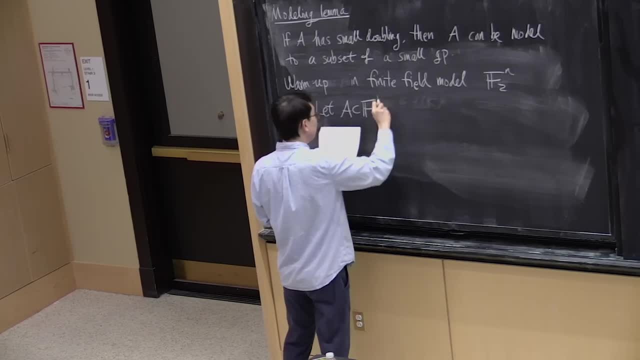 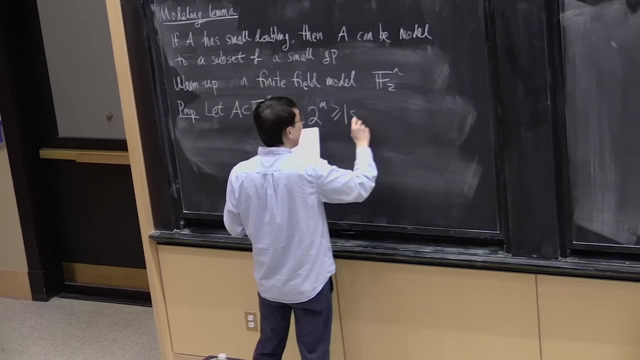 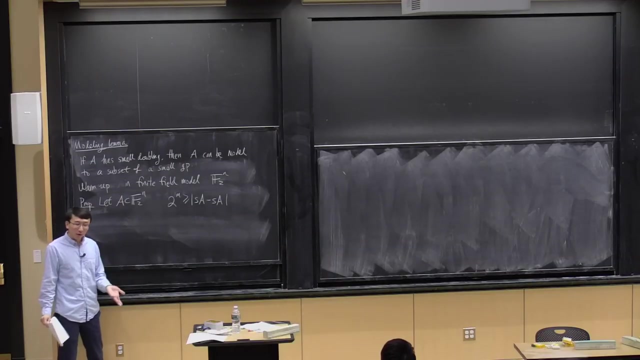 Suppose you have a, a subset of f2 to the n, And suppose that m is small. It's some number such that 2 to the m is at least as large as S A minus S A. So remember from Plunica-Ruzsa you: 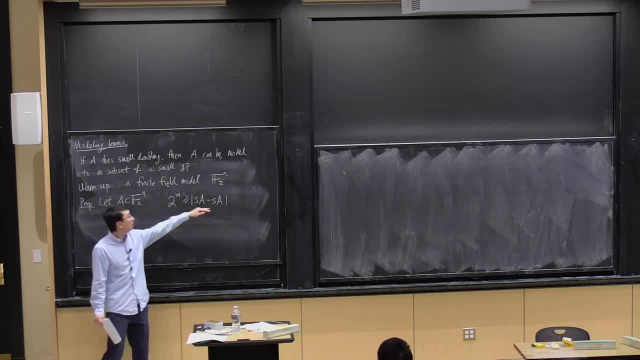 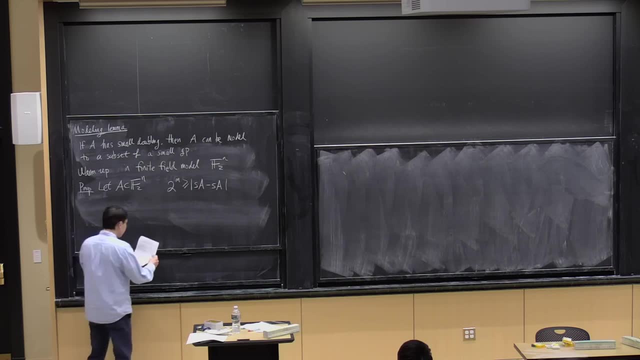 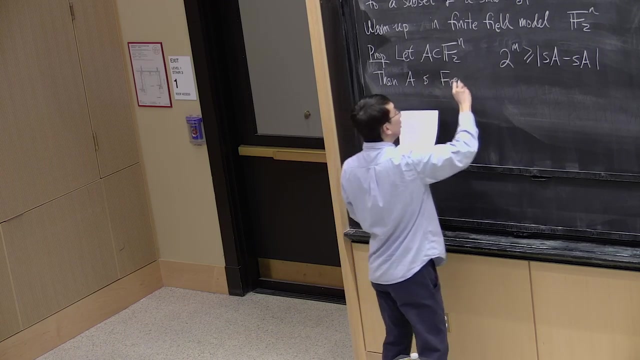 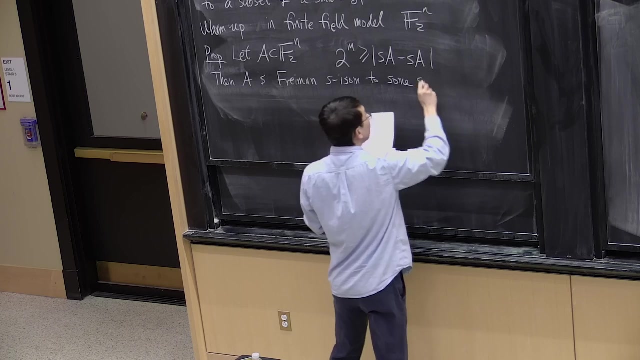 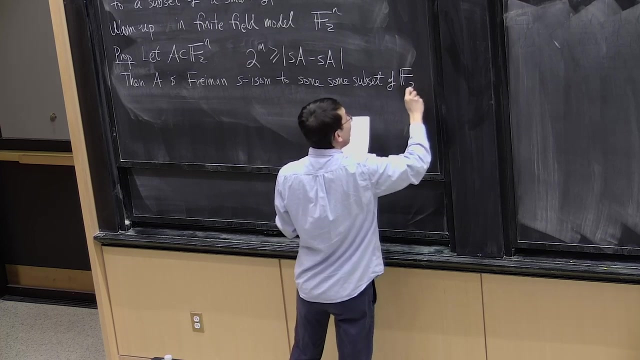 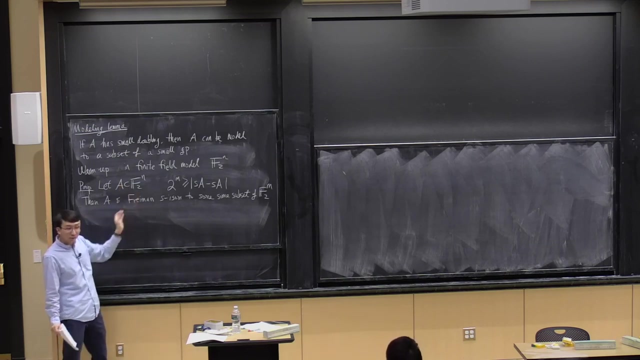 know that if a plus a is small, then this iterated sum is small. So suppose we have these parameters and sets. The conclusion is that a is Freiman isomorphic to some subset of f2 raised to m. So initially a is in a potentially very large vector. 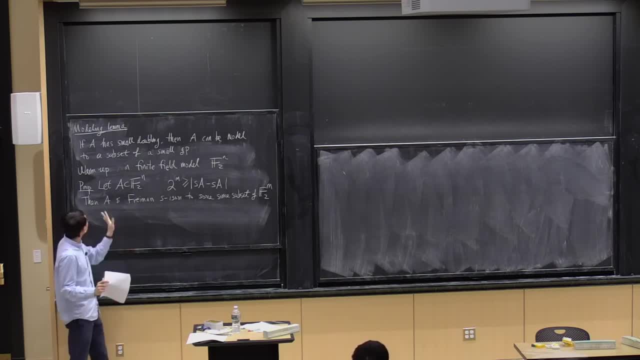 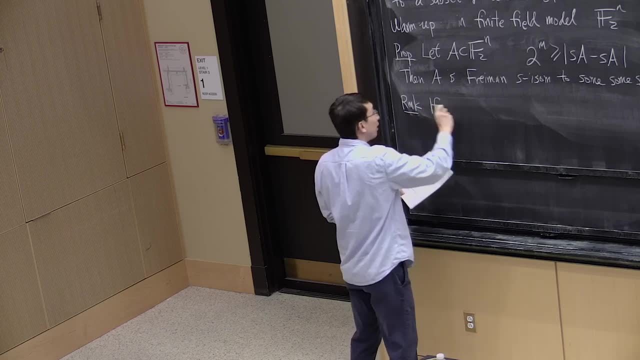 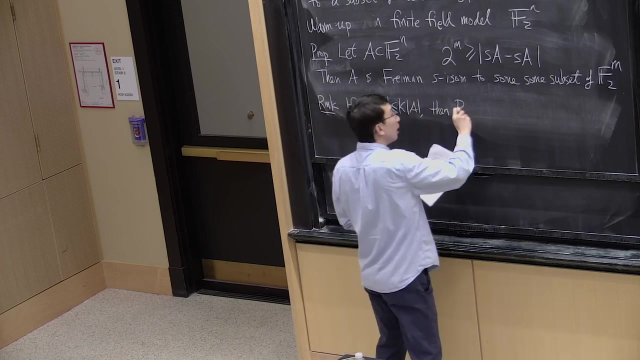 space, or it could be all over the place. And what we are trying to say here is that if a has small, small doubling, so if a has small doubling, then by Plunica-Ruzsa S A minus S A has size, not too much. 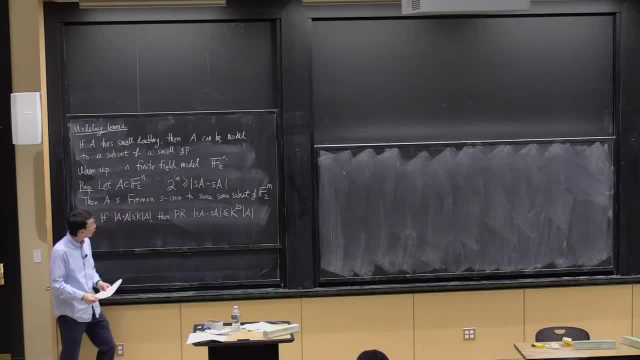 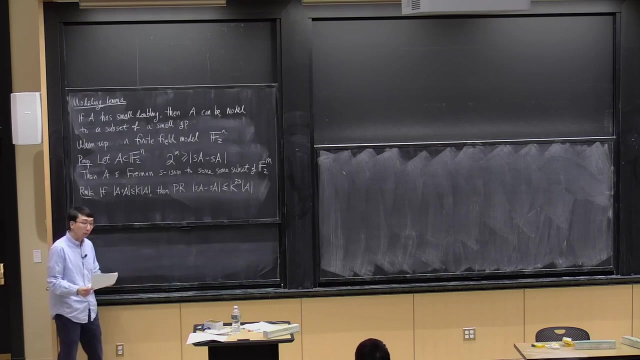 bigger than a itself, only a bounded times the size of a itself. So I can take an m so that the size of this group is only a constant factor larger than the size of a itself. So we're in a pretty small group, So we are able to model a, even though initially it 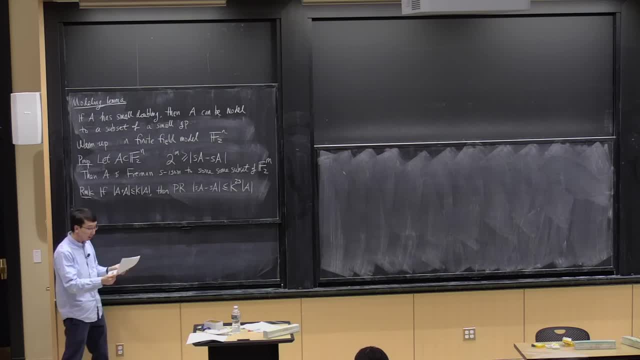 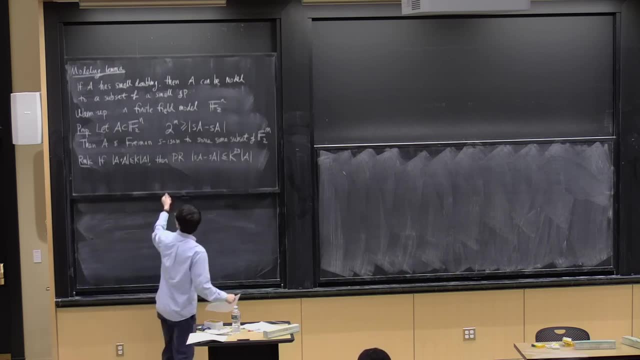 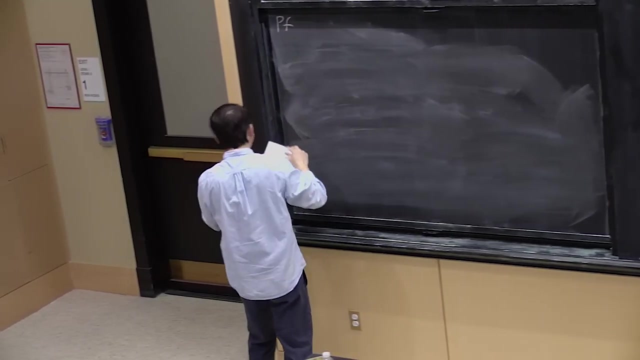 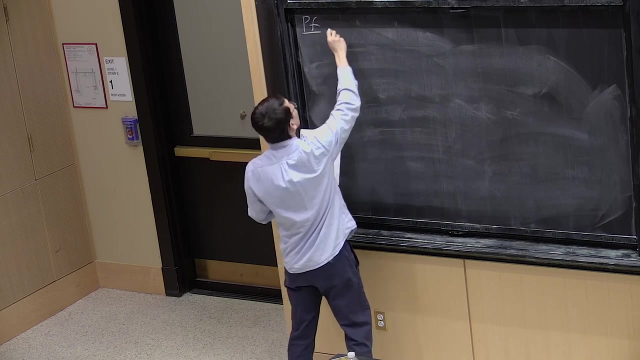 sits inside a pretty large n-b-n group by some subset in a pretty small group. All right, so let's see how to prove this modeling lemma. So the finite field setting is much easier. It's not too hard to do, It's not too hard to deal with because we 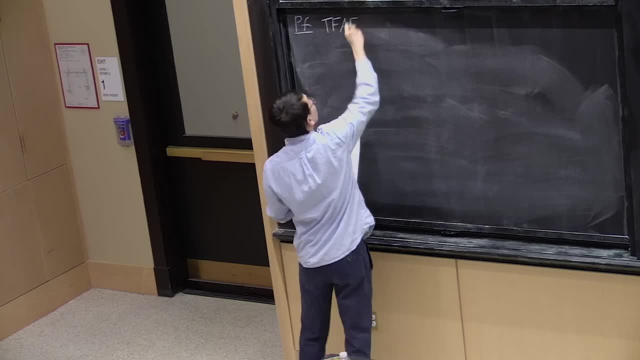 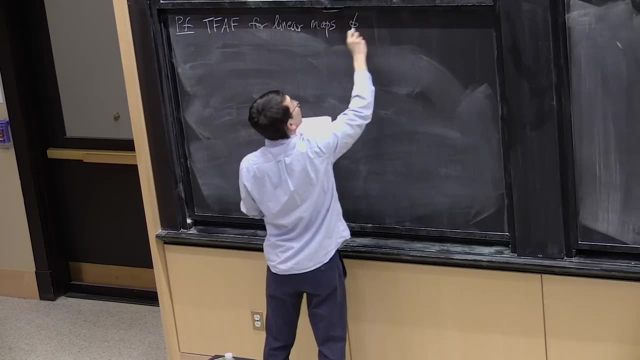 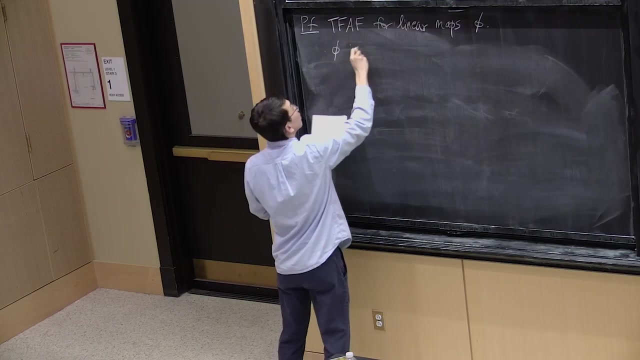 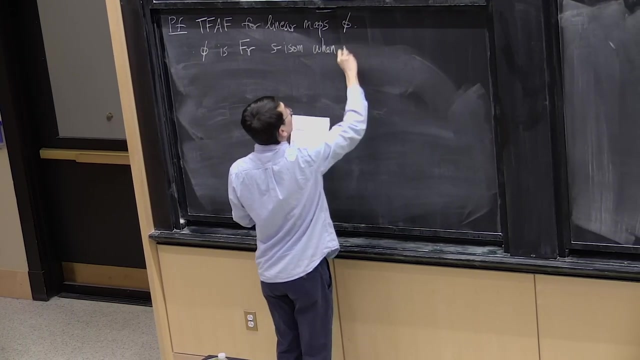 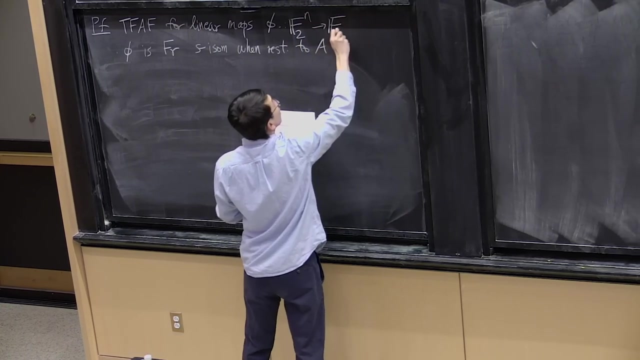 can look at linear maps. So the following are equivalent for linear maps: phi, so for group homomorphisms. So phi is a Freiman S-isomorphism when restricted to a. So here, phi, I'm going to let it be a linear map from F2. 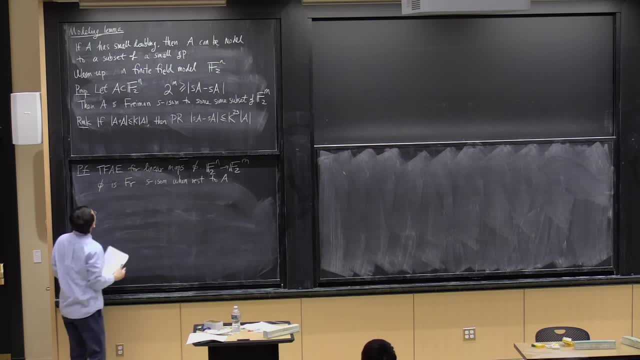 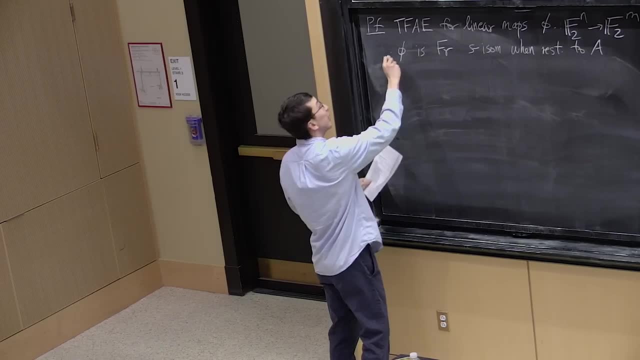 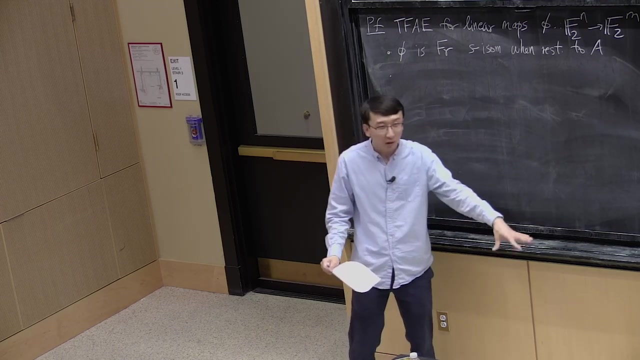 to the n, to F2 to the m, the following are equivalent. So we would like phi to be a Freiman S-isomorphism when restricted to a, because this means that I restrict to a and I restrict to its image. so it's Freiman isomorphically map. 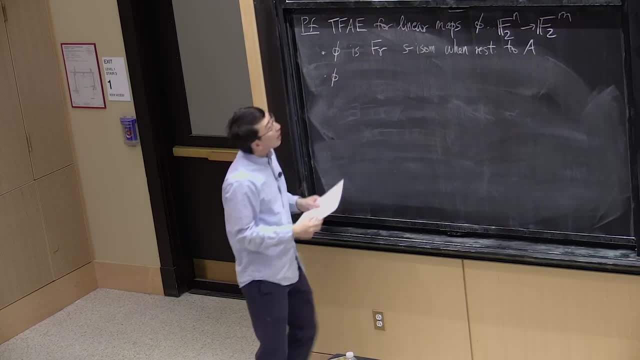 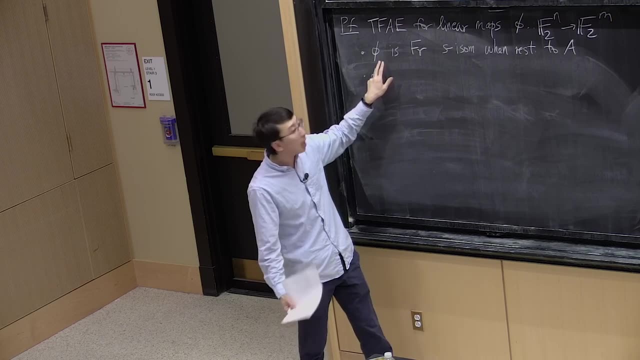 onto the image. So what does that mean? So well, if S so phi is already a homomorphism, so it's automatically a Freiman S-homomorphism. For it to be an S-isomorphism, it just. 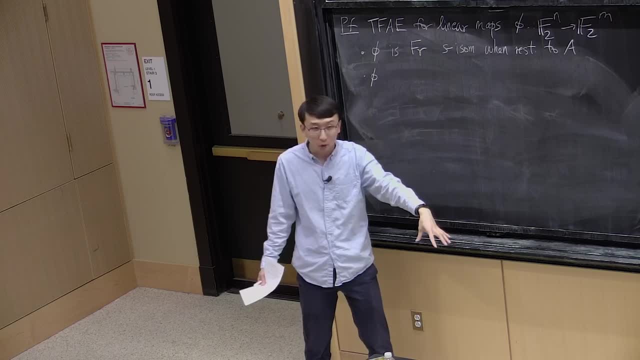 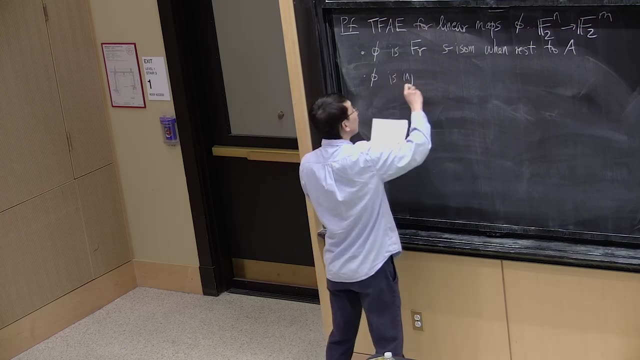 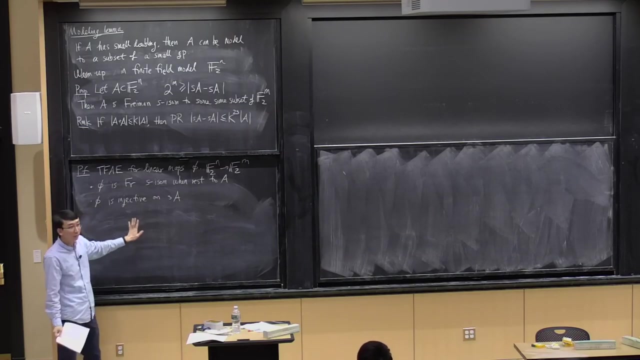 means that there are no additional linear relations in the image that were not present earlier, which means that phi is injective. So that's a. So let's just think about the definition. And in the definition, if you know additionally that phi is a homomorphism, everything is much cleaner. 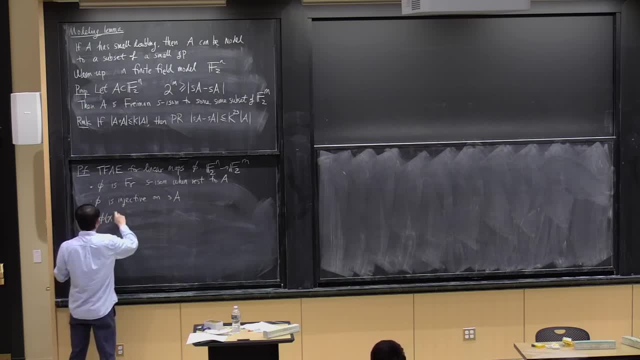 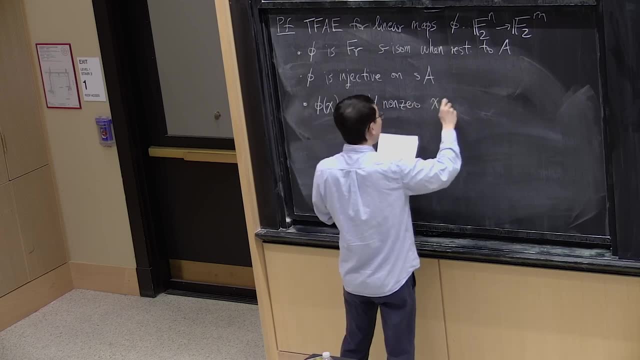 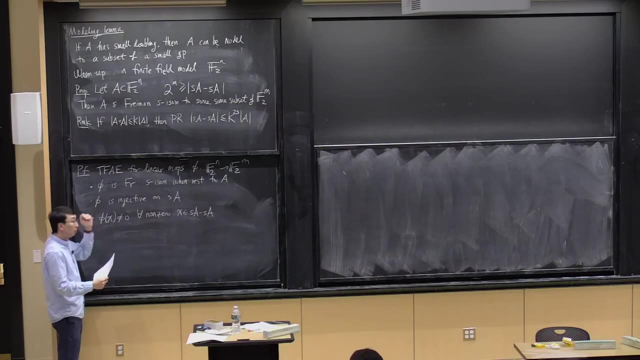 It is also equivalent to that phi of x is non-zero. for every non-zero element, x of S-a minus S-a. OK, so this is a very clean characterization of what it means to be a Freiman S-isomorphism when you are in a bilinear group and you have linear maps. 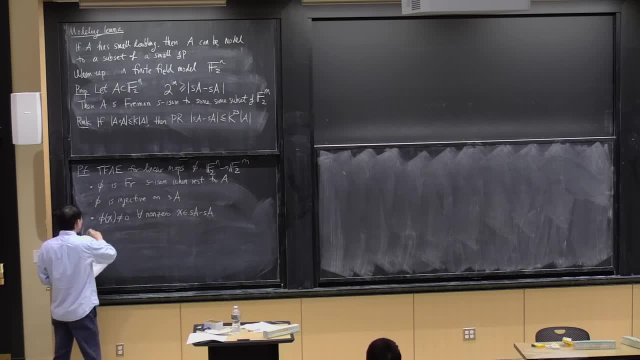 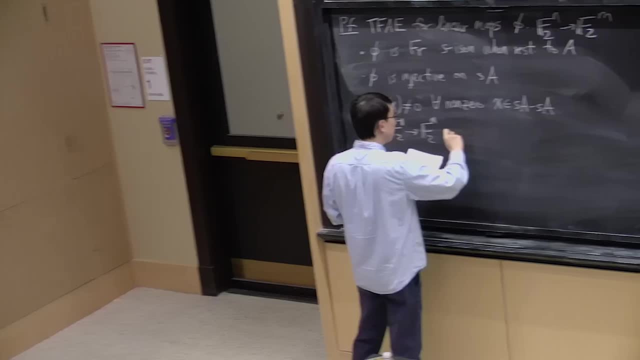 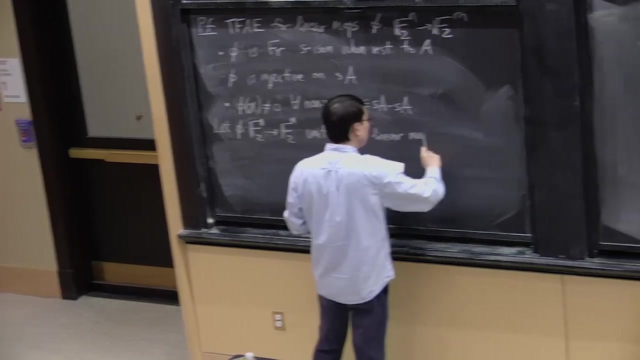 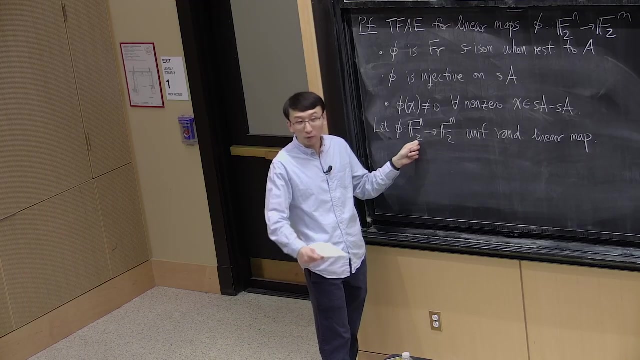 You have homomorphisms. So if we start by taking phi to be a uniformly random linear map, OK, so in particular. so, for example, you find you pick a basis and you send each basis element to a uniformly random element. 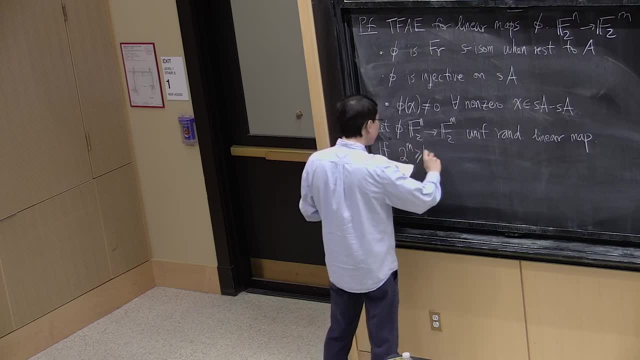 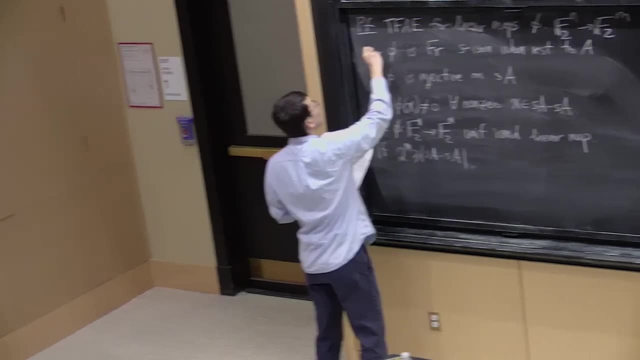 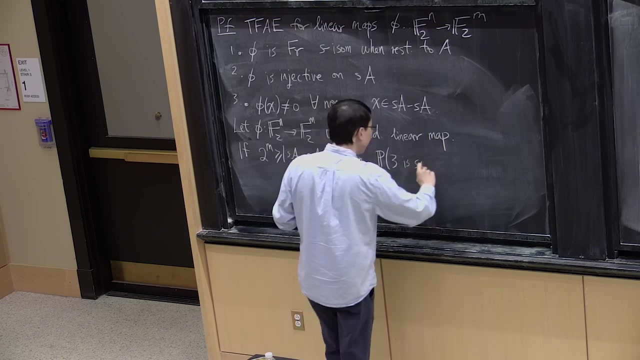 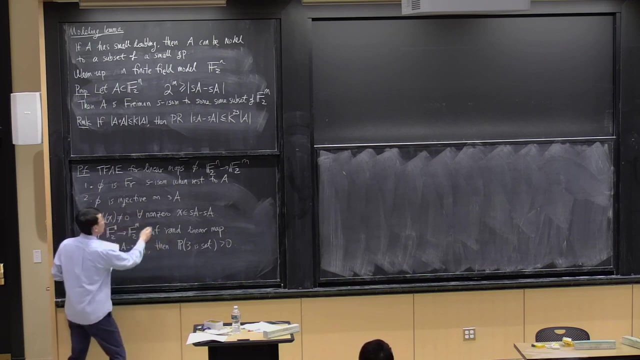 Then we find that if 2m is at least S-a minus S-a, then so let me call these properties 1, 2, 3.. So then the probability that 3 is satisfied is positive, because each element of S-a minus S-a. 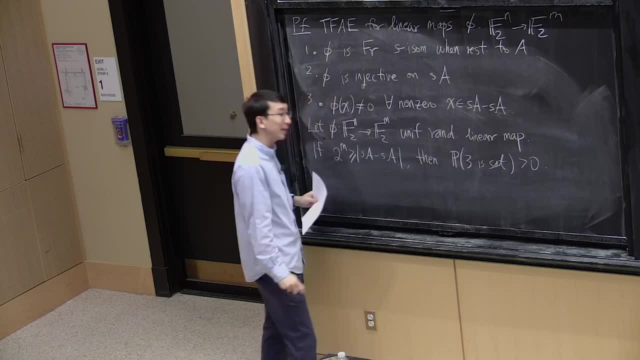 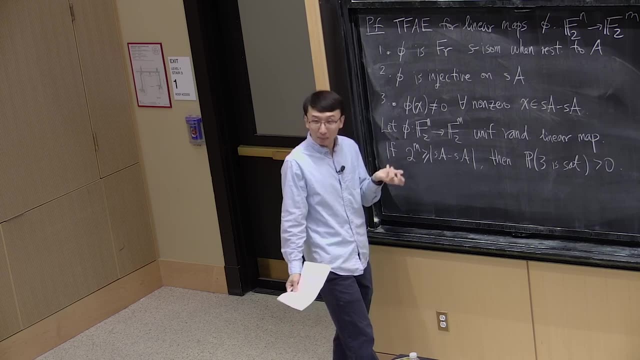 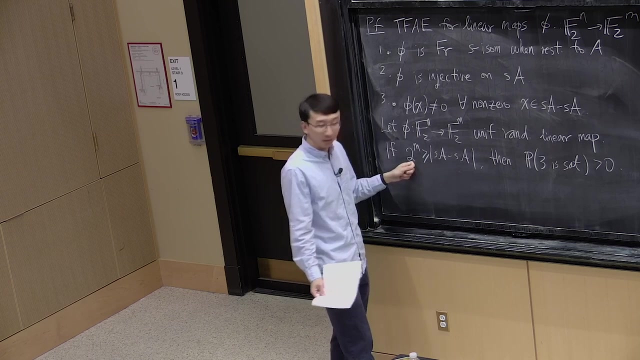 well, I can also ignore 0. So each non-zero element of S-a minus S-a violates this property with probability exactly 2 to the minus m. Everything's uniform. So if there are very few elements and the space is large enough, then the third basis. 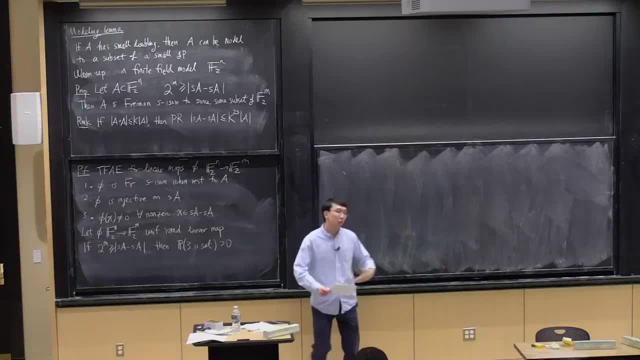 the third bullet is satisfied with positive probability. So you get a Freiman S-isomorphism. Any questions To get this model in this case in the finite field setting, it's not so hard. So you kind of project the whole set. 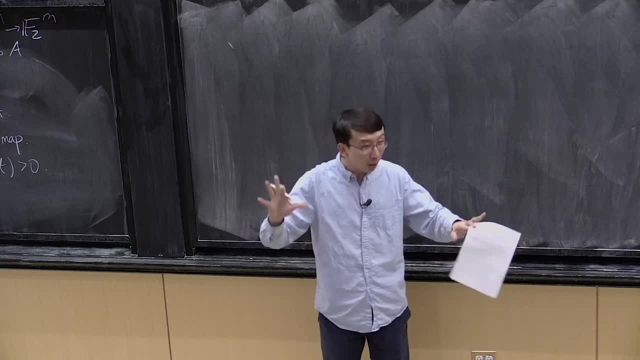 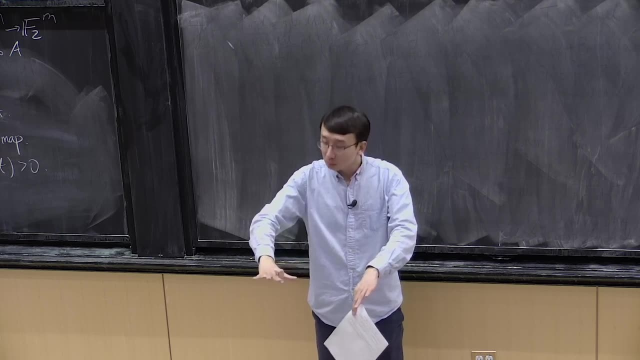 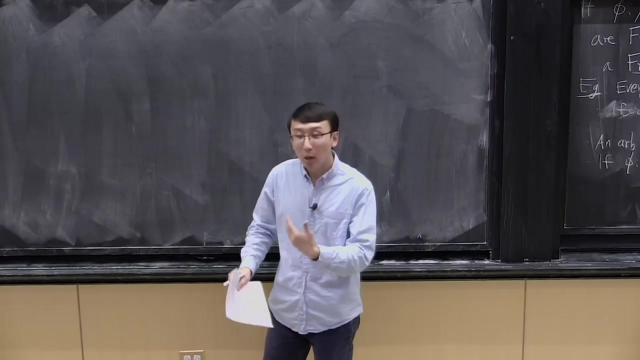 even though initially it might have very be very spread out into a lot of dimensions. You project it down to a small dimensional subspace randomly And that works So that with high probability preserves all the additive structures that you want, provided that you have small doubling. 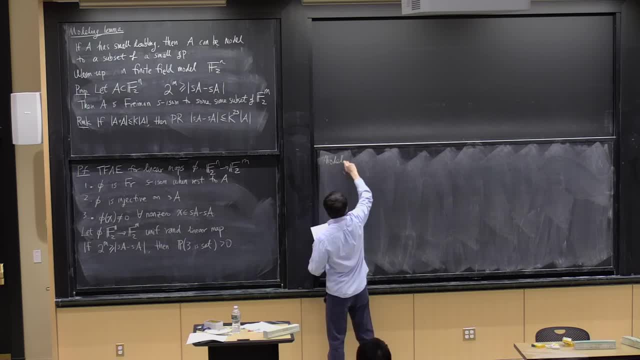 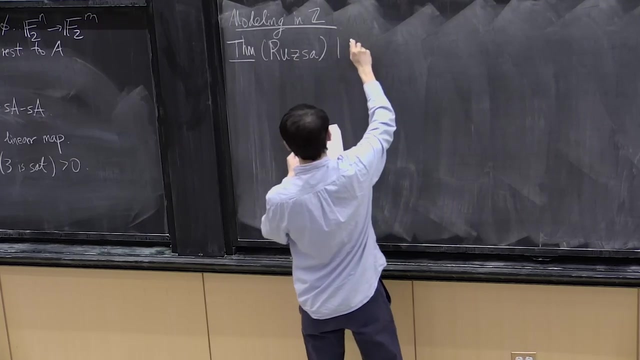 Now let's look at what happens in Z. So in Z things are a bit more involved, But the ideas, actually a lot of the ideas, come from this proof as well. So Rucha's modeling lemma tells us that if you have a set of integers, always a finite set. 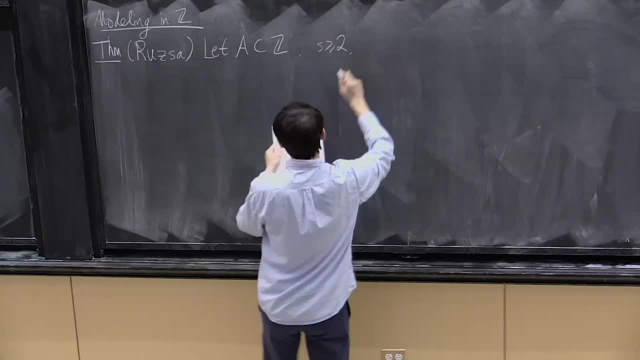 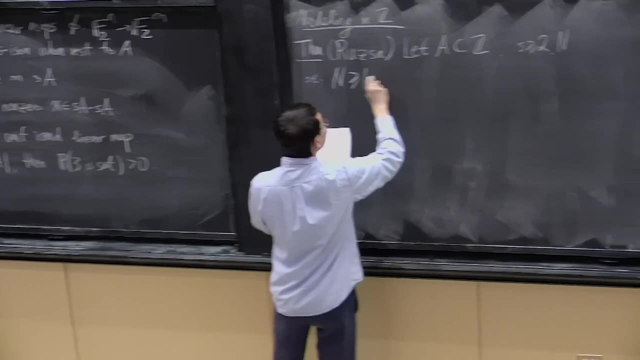 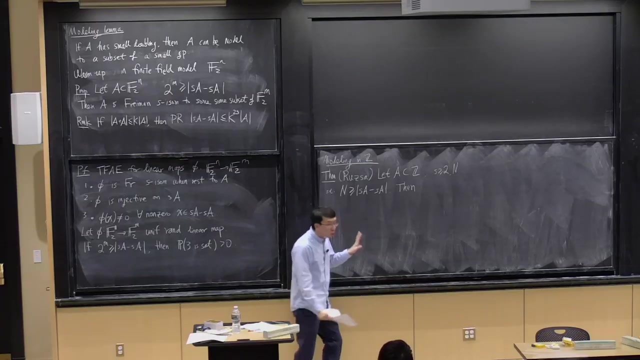 and integers s and n are such that n is at least S-A minus S-A, then OK. OK, So it turns out you might not be able to model the whole set A, But it will be good enough for us to model a large fraction. 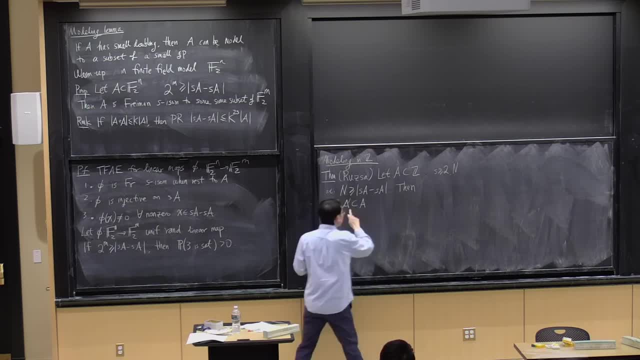 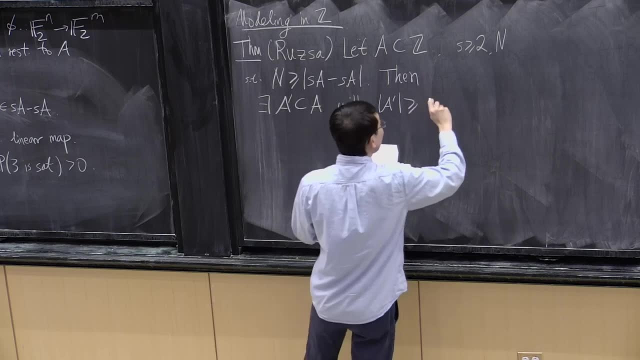 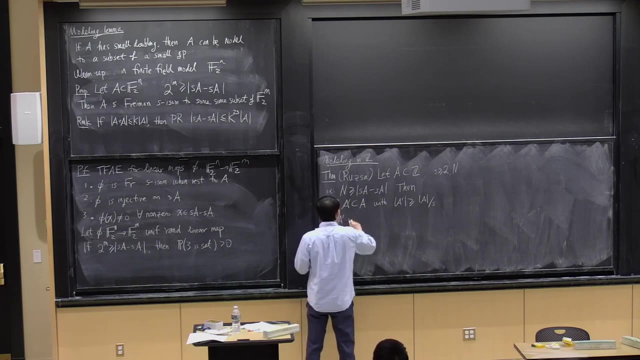 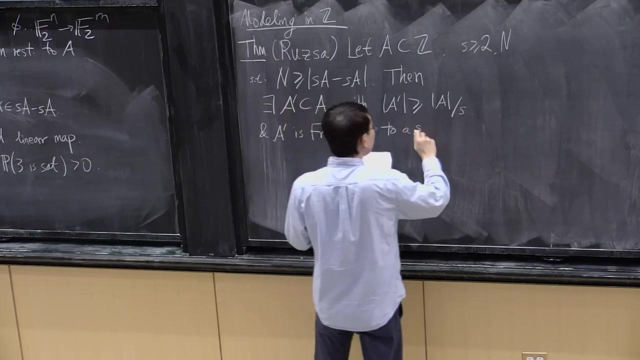 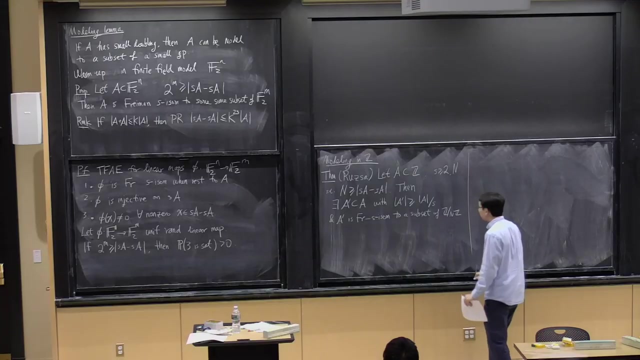 But then there exists an, A prime subset of A, with A prime being at least an S fraction of the original set And A prime is Freiman S-isomorphic And A prime is Freiman S-isomorphic to a subset of Z mod M. 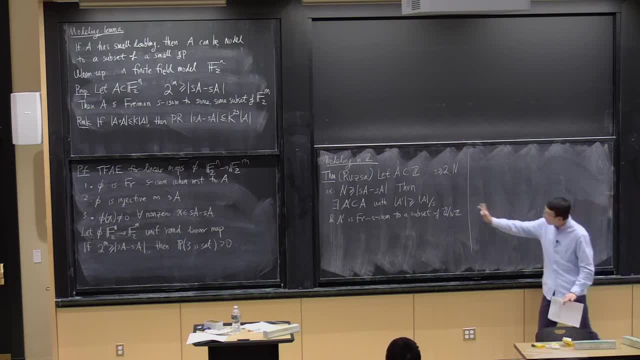 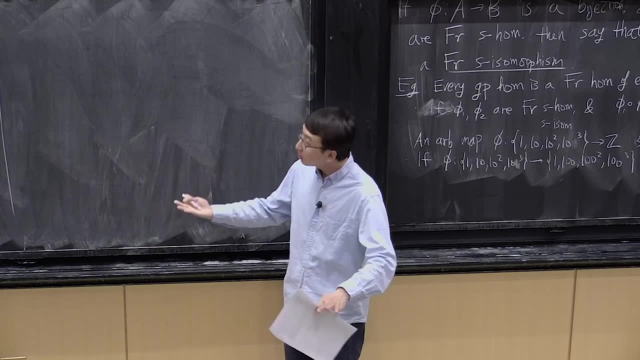 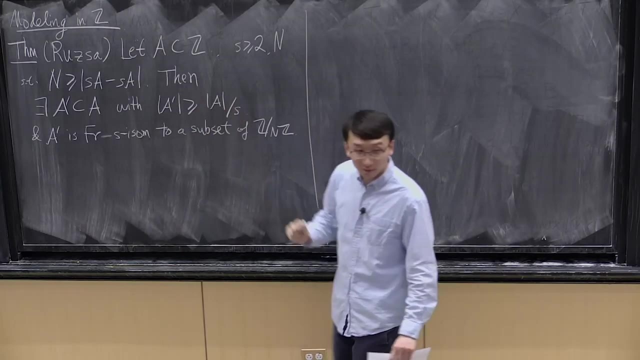 So same message as before, with an extra ingredient that we did not see before. But the point is that if you have a set A with controlled doubling, then well, now you can take a large subset, a large fraction of A, that is, Freiman isomorphic. 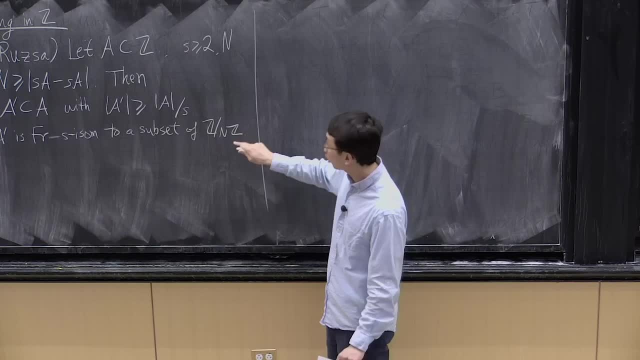 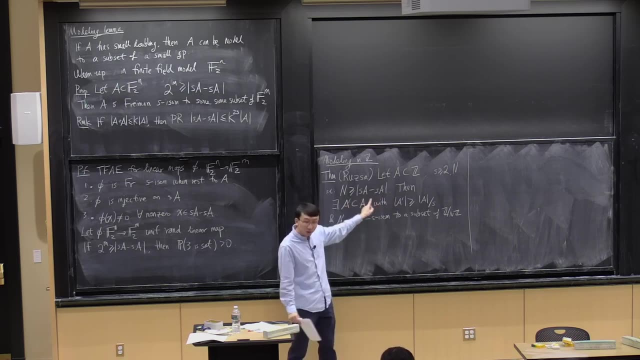 to a subset of a small group. This is small because we only need n to exceed S-A minus S-A, which are only constant factor, more than the size of A. Yeah, Is S greater than 2 comma n or YUFEI ZHAOBENGALLER- So X greater than 2. 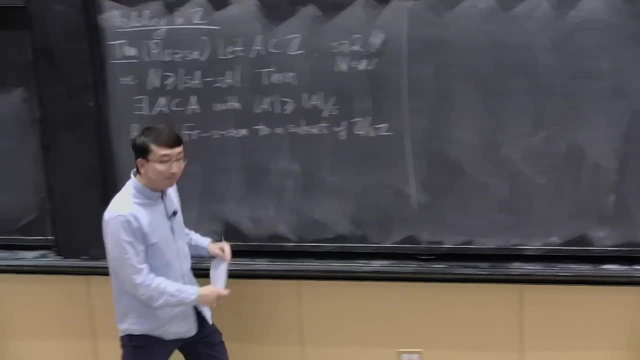 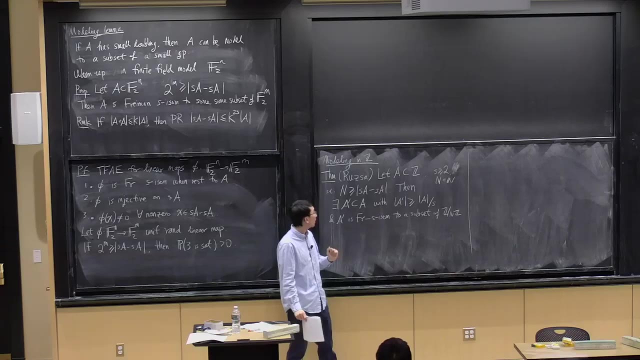 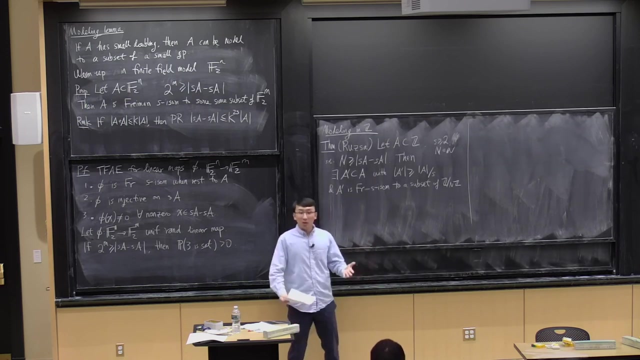 separately and some integer. Thank you, YUFEI ZHAOBENGALLER- So in our application, S will be a constant, S will be 8. So think of S as some specific constant. Any questions? So let's prove this modeling lemma. 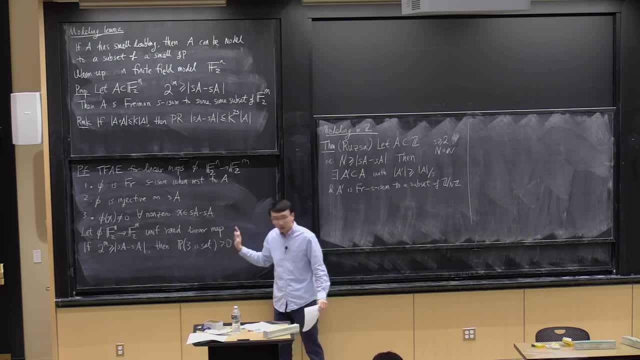 We want to try to do some kind of random map, But it's not clear how to start doing a random map if you just start in the integers. So what we want to do is first place ourself in some group where we can consider. 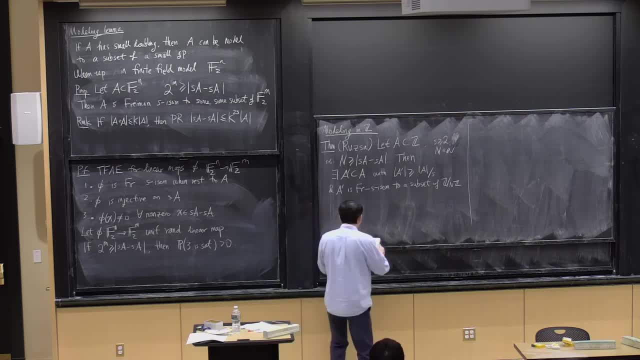 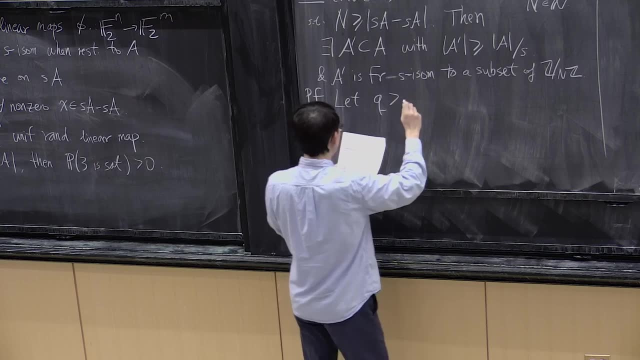 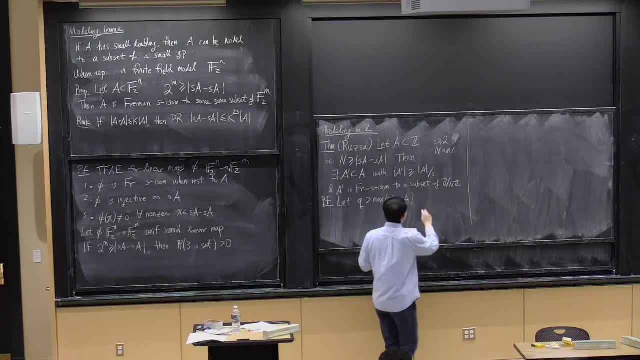 random automorphisms. So we start by- perhaps very wastefully, choosing a prime q bigger than the maximum possible S-A minus S-A. So just choose a large enough prime. I don't care how large you pick. q can be very, very large. 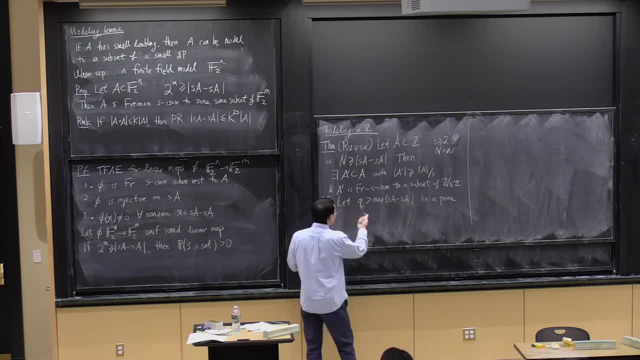 Pick a prime. And now I work inside Z mod q. I notice that if I make q large enough, then A sits inside Z mod q, Freiman isomorphically, S isomorphically. So just pick q large enough so that you don't. 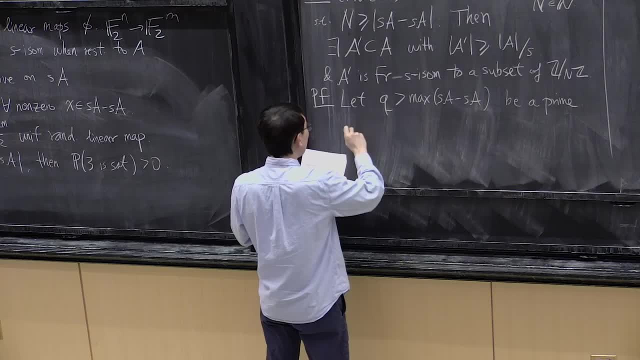 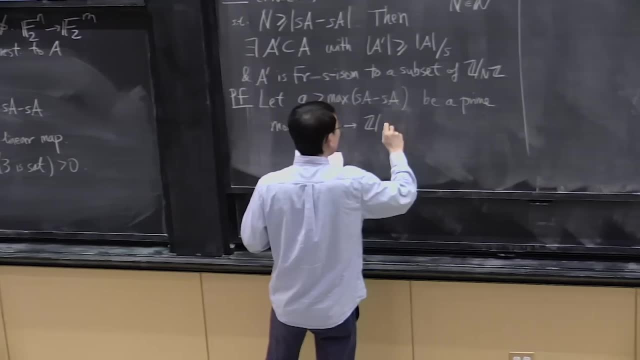 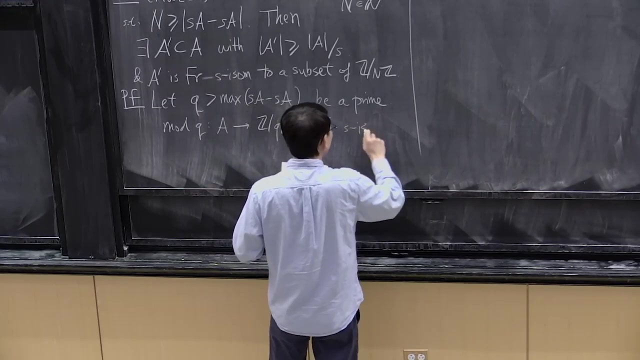 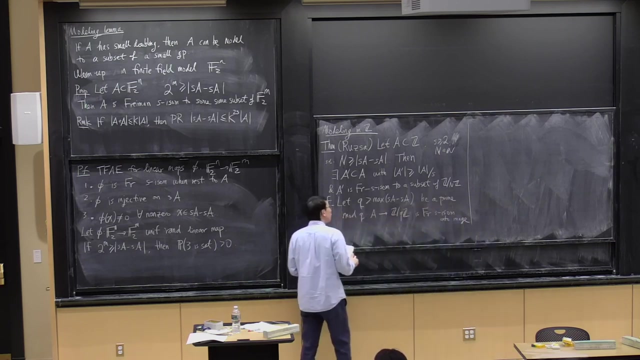 have to worry about any issues. So OK, And yeah, So the mod q map from A to Z. mod q, So it's Freiman isomorphic, Freiman S isomorphic onto its image. So let's now consider a sequence of maps. 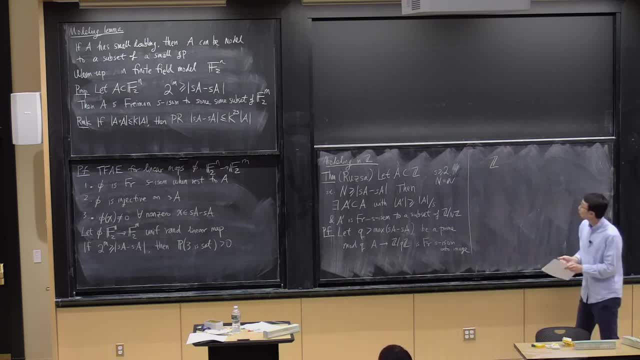 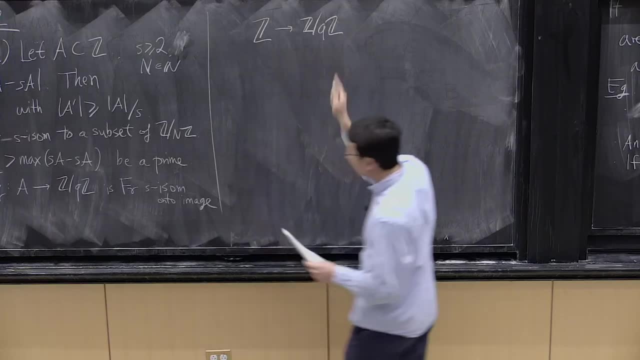 And we're going to denote the sequence like this. So we start with Z, So that's where A originally sits, And maps to Z, mod q. So that was the first map that we saw, And now we want to do a random automorphism. 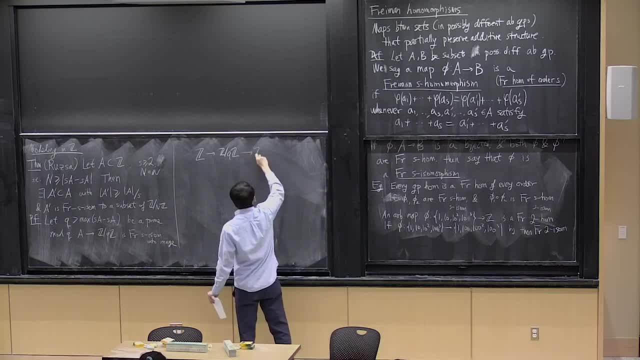 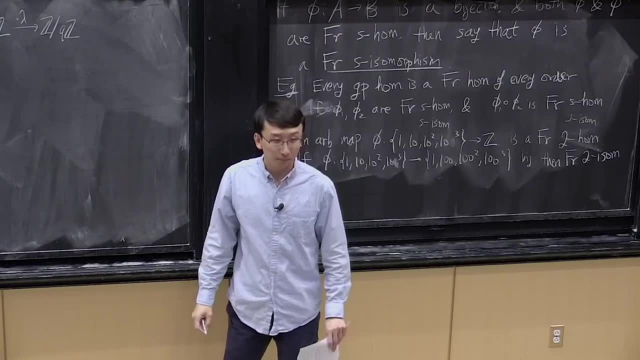 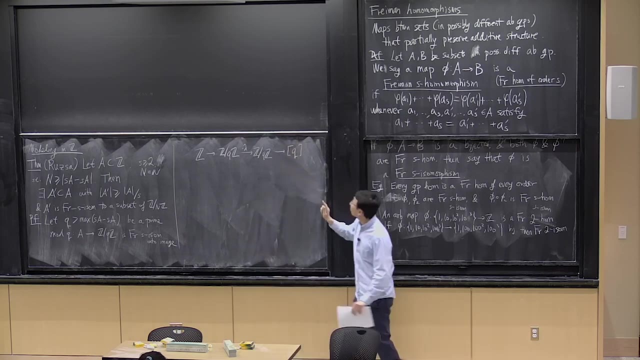 like the random map earlier, But in Z mod q there are lots of nice random automorphisms, namely multiplication by some non-zero element. And finally we can consider the representative map OK, Where every element of Z mod q I. 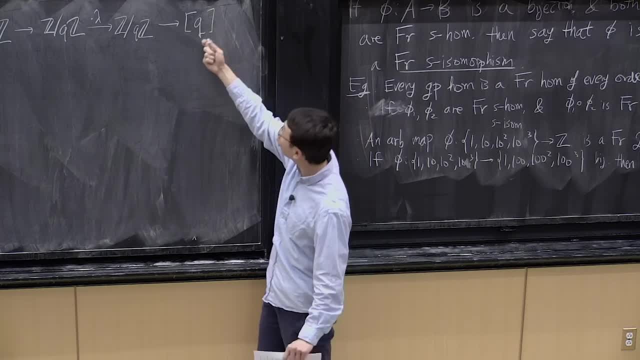 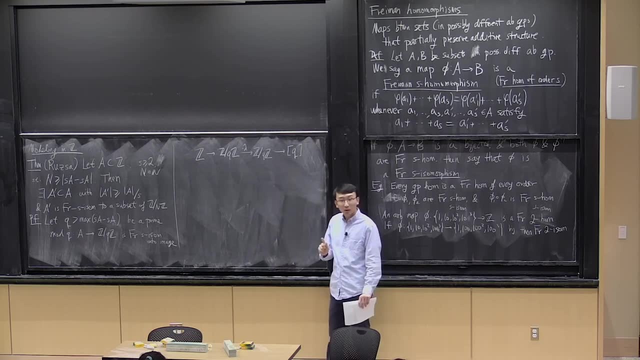 can associate to it a positive integer from 1 to q which agrees with Z mod q. So the final step is not a group homomorphism, So we need to be more careful. So let me denote by phi this entire map, So from the beginning to the end, this composition. 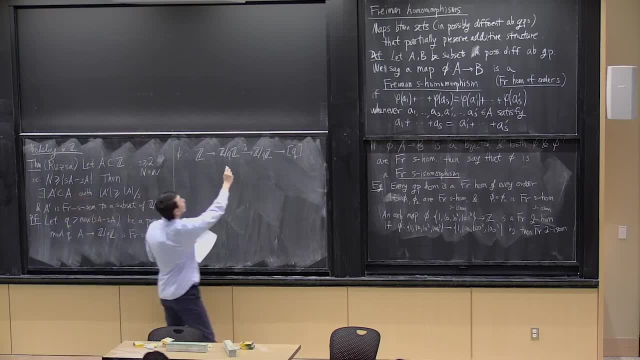 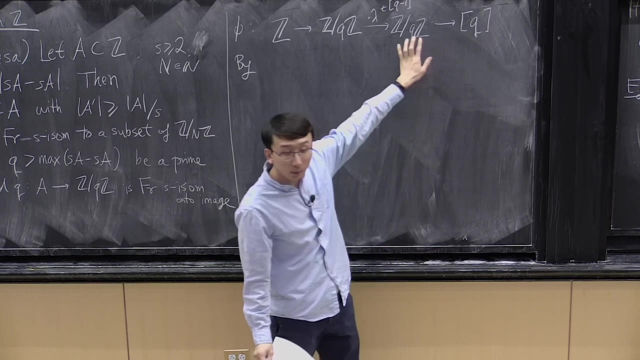 I'll denote by phi And lambda. here is some element. And lambda here is some element between 1 and q minus 1.. Now remember what we said earlier, that this map, this final map here, might not be a Freiman homomorphism. 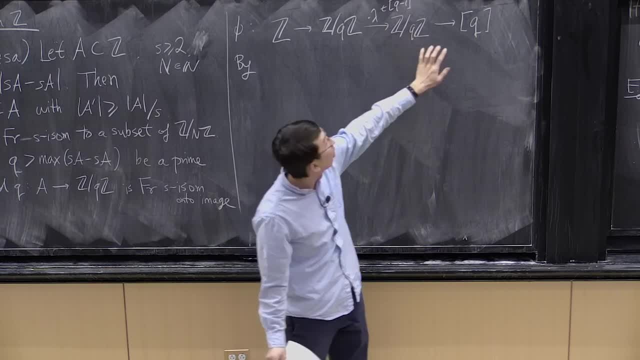 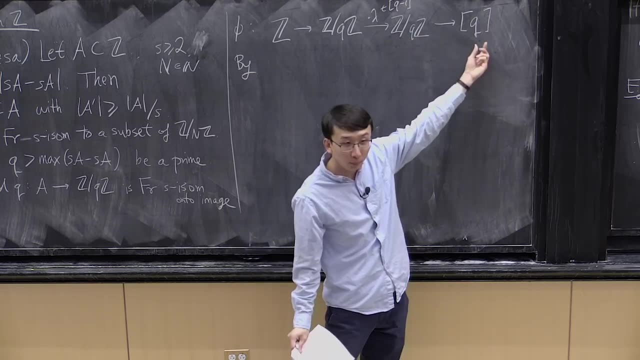 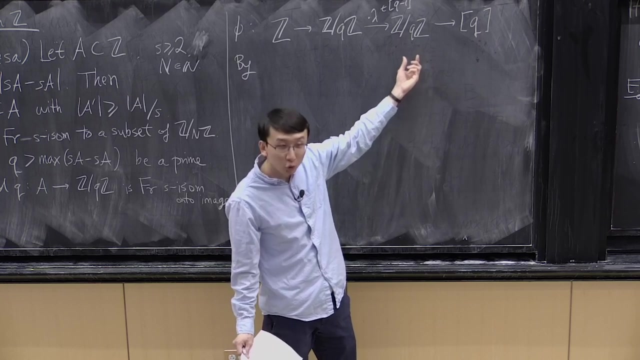 because there are some additive relations here that are not preserved over here. But if I restrict myself to a small interval, then it is a Freiman homomorphism. if you restrict yourself to an interval, If you restrict yourself to an interval, you cannot have extra relations over here. 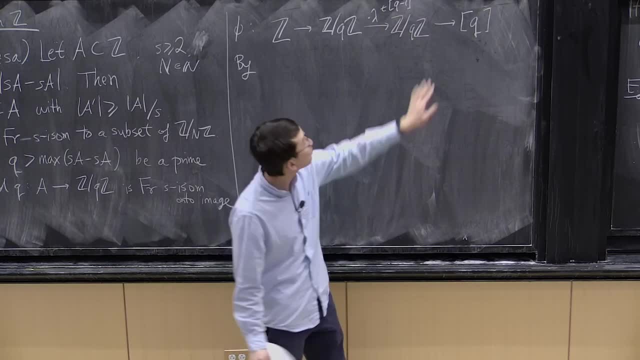 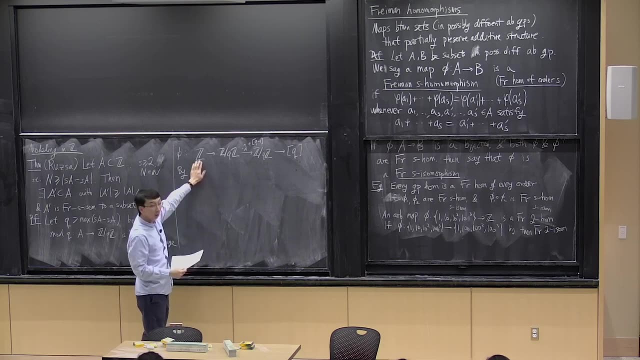 because they cannot. the interval is small enough, you can't wrap around. So let's consider restrictions to small intervals. But I start with a over here, So I want to restrict myself to some interval so that I still have lots of a in that restriction. 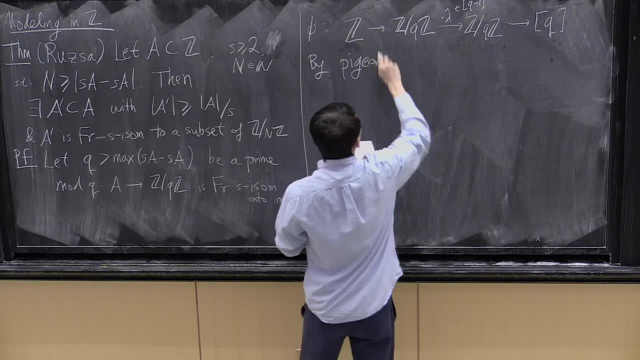 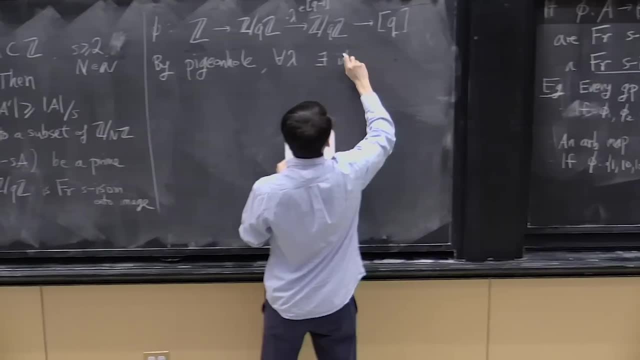 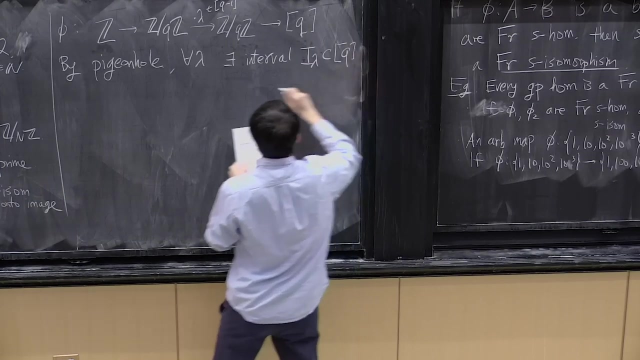 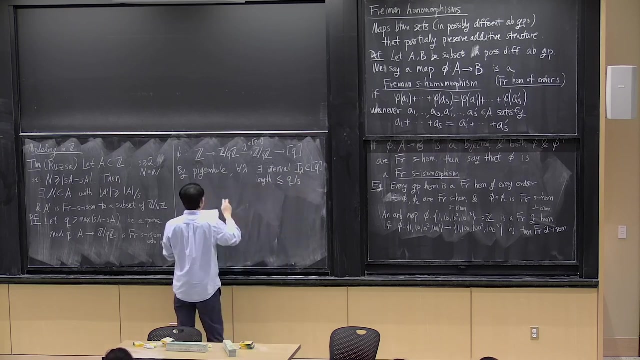 And you can do this by pigeonhole, So by pigeonhole. for every lambda there exists some interval, we'll denote by i sub lambda, inside q. So the length of this interval will be, at most, q over s, such that if I look at the restriction of this interval, 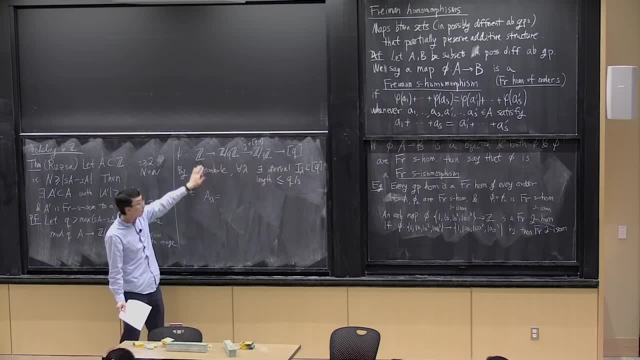 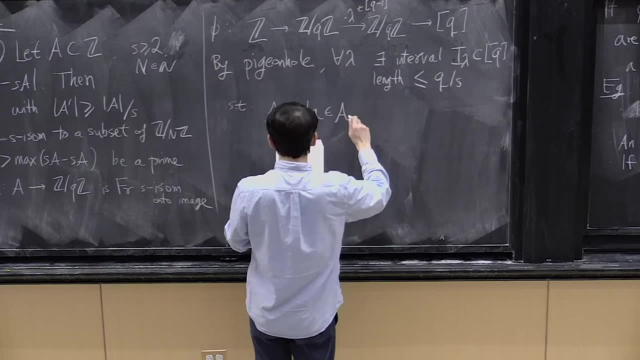 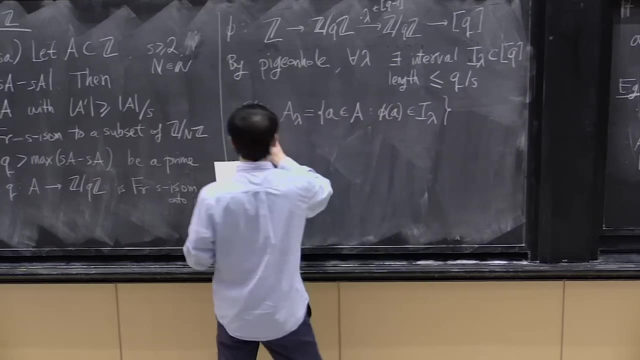 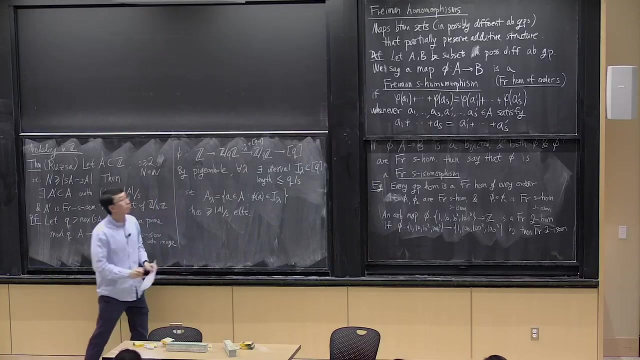 if I pull it all the way back to the beginning, then I still get lots of elements of a. So a sub lambda, meaning the elements of a whose map gets sent to, this interval has at least a over s elements. So, for instance, you can chop up q into s different. 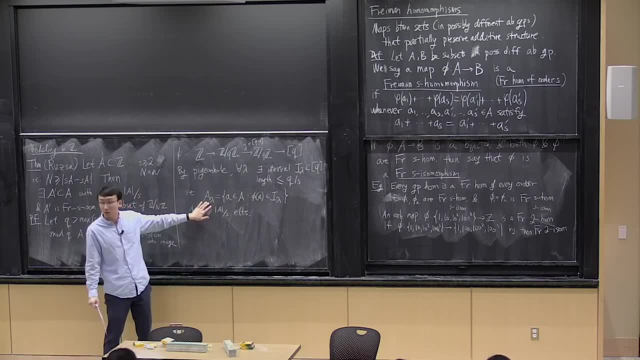 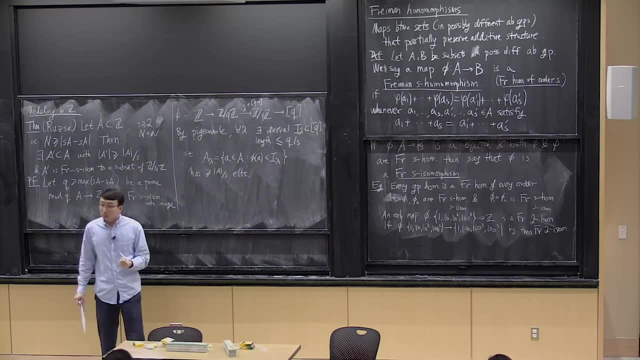 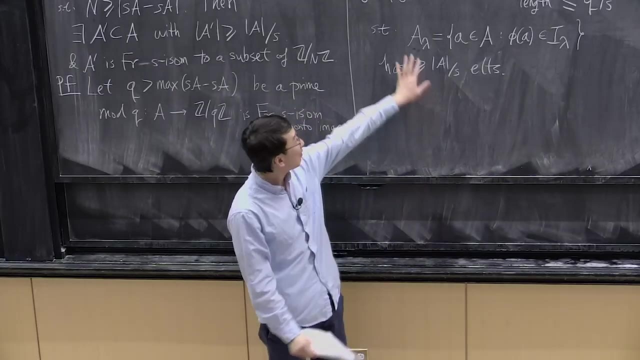 intervals, So one of them will have lots of elements that came from a, And this is why, in the end, we only get a large subset of the a, because we're going to forget about everything else and focus our attention on this set here. 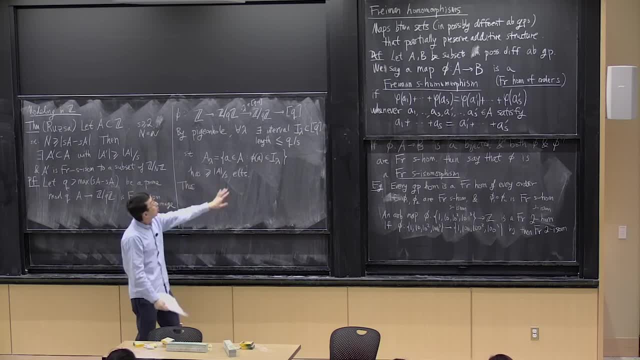 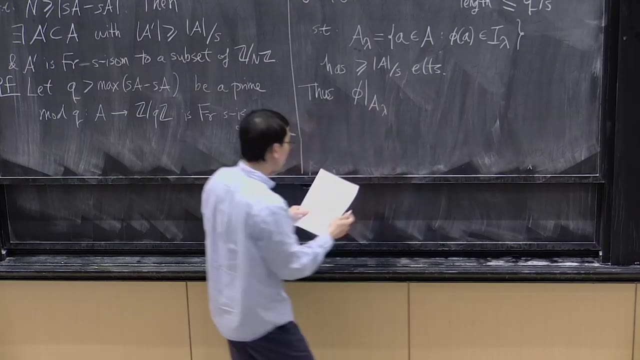 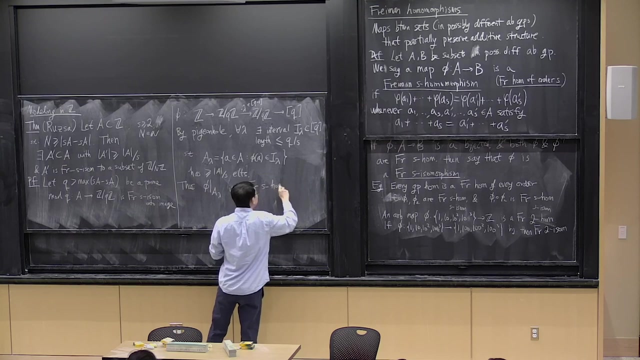 Thus by our earlier discussion having to do with with the final map being the Freiman-S homomorphism, when you're working inside a short interval, we see that phi, if you restrict to this a sub lambda, is a Freiman-S homomorphism. 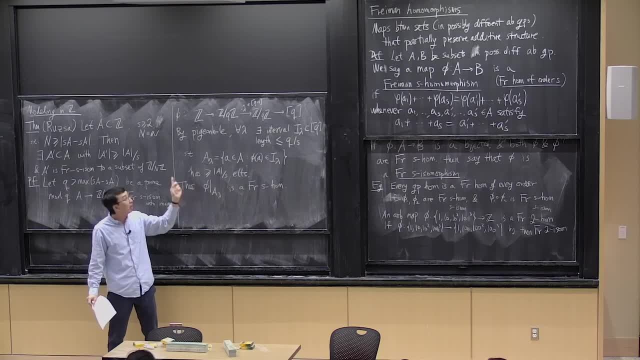 Each step is a Freiman homomorphism because it's a group homomorphism. And the final step in this restriction is also a Freiman-S homomorphism. OK, It's a Freiman homomorphism, Freiman-S homomorphism. 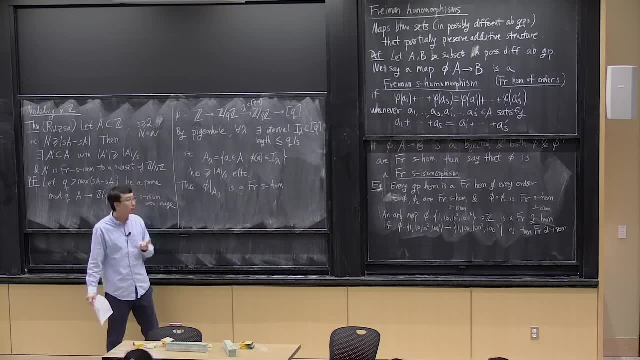 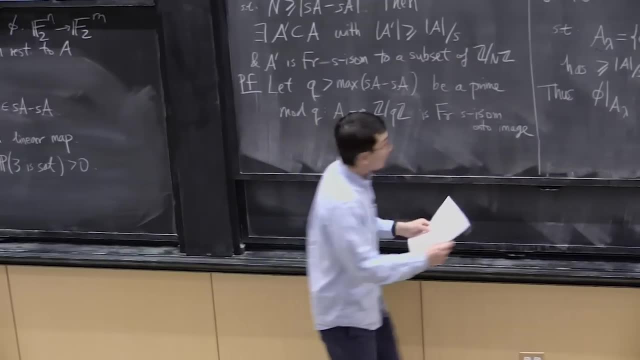 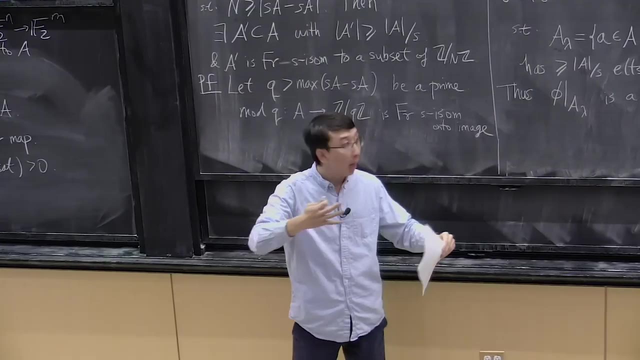 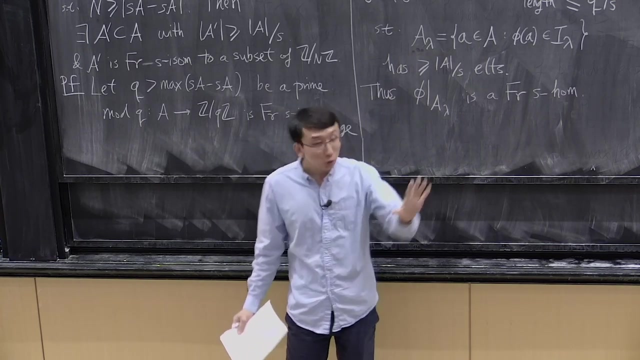 because what we said about working inside short intervals, So this part is very good, All right. so now let me consider one more composition. So, at the end of the day, we would like to model this: a lambda inside some small cyclic group. 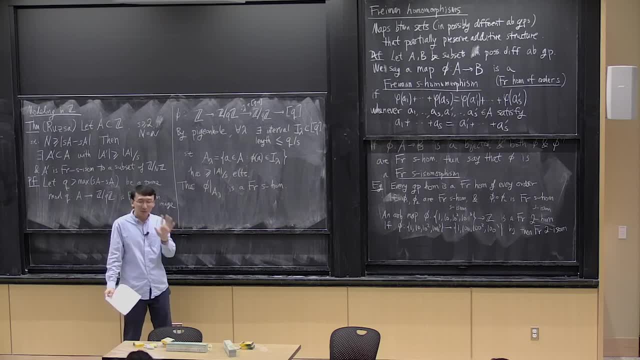 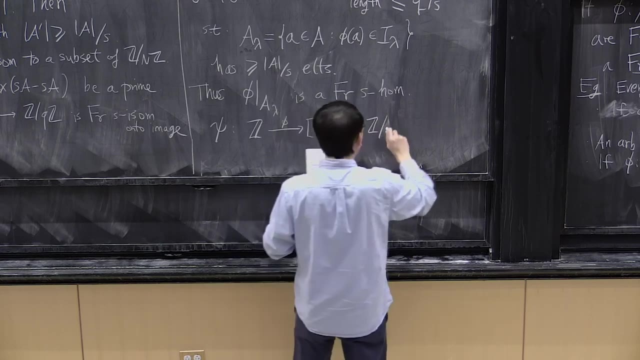 So far we don't have small cyclic groups yet, But I'm going to manufacture a small cyclic group. So we're going to consider a map where first you take that phi all the way until the end And now you take a mod M map. 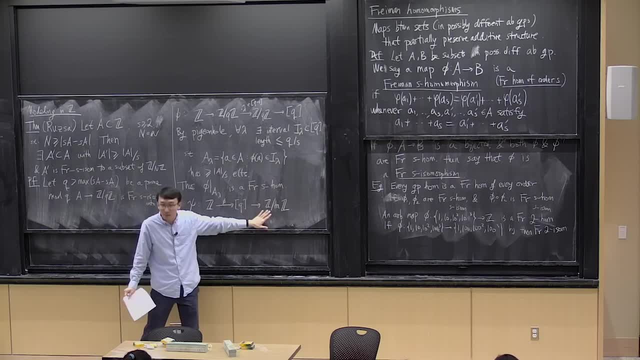 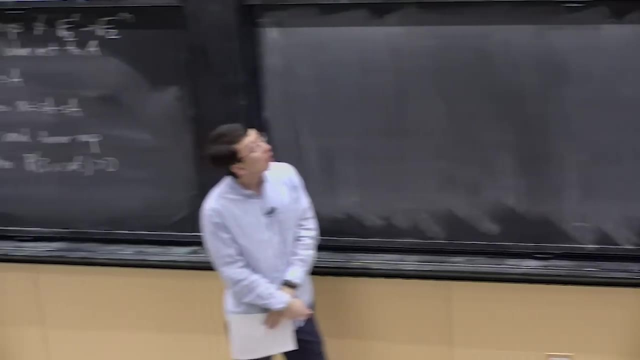 So if I don't write anything, if it goes to Z, mod M, it means the mod M map. So let me consider phi or psi, psi, which is the composition of these two maps. All right, so we would like to say: 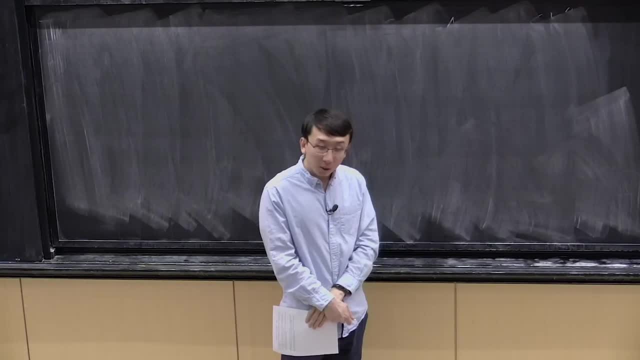 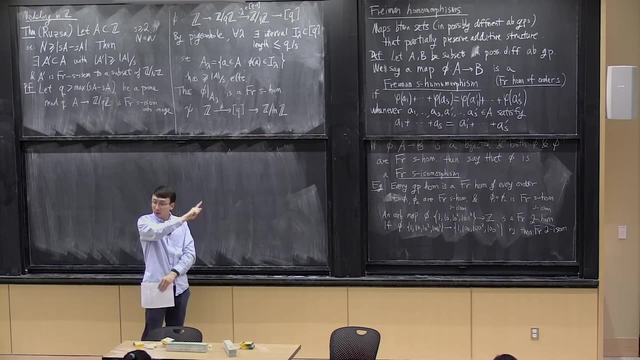 that you can choose this lambda so that this, A sub lambda, gets mapped Freiman-S isomorphically until to the end. So far everything looks pretty good. So you have Freiman-S homomorphism and you have a group homomorphism. 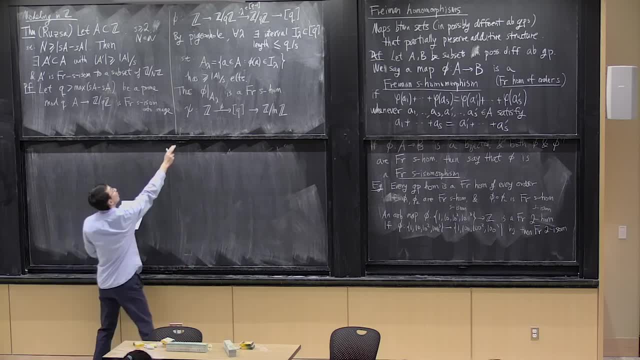 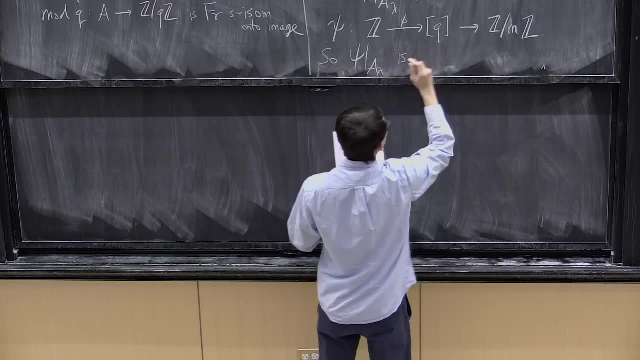 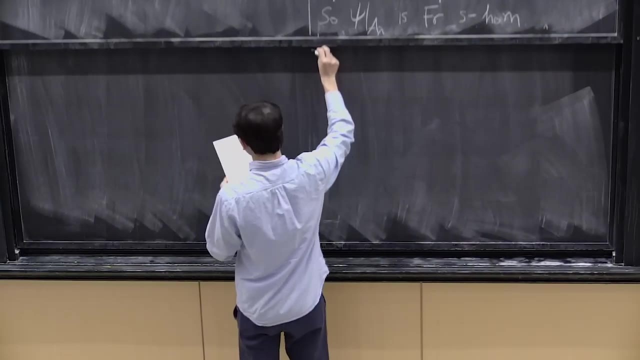 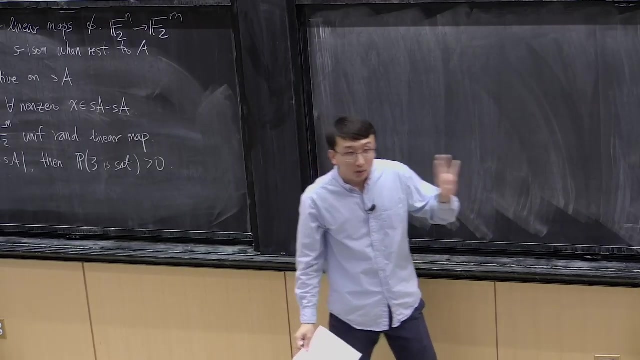 You have a. so the whole thing is a Freiman-S homomorphism. So phi- the psi is restricted to A sub lambda- is a Freiman-S homomorphism. But now the thing that we really want to check is if there are some relationships that are present. 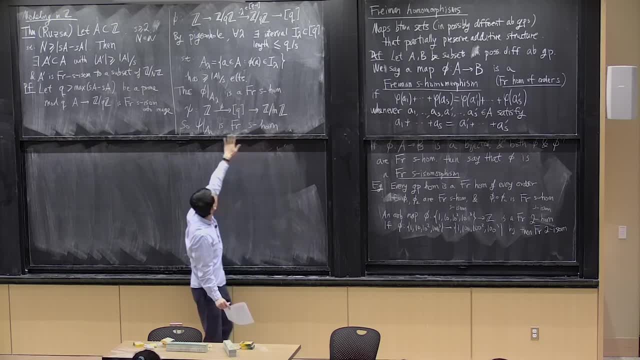 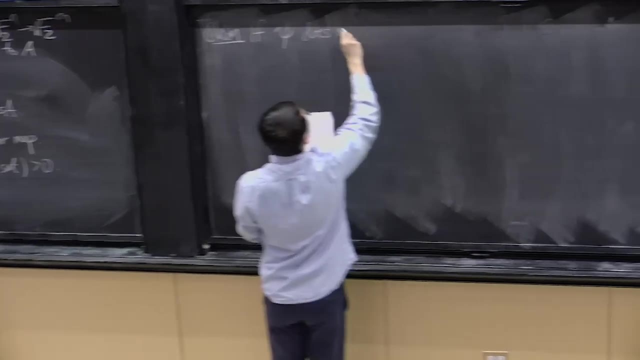 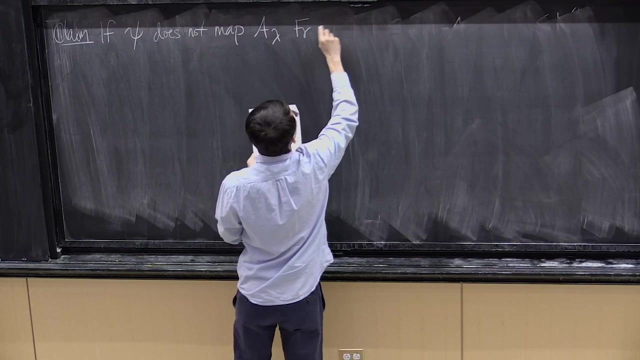 at the end in Z mod M that were not present earlier. All right, so we need to check that and we claim that if psi does not map A sub lambda Freiman-S isomorphically, then something has to have gone wrong. 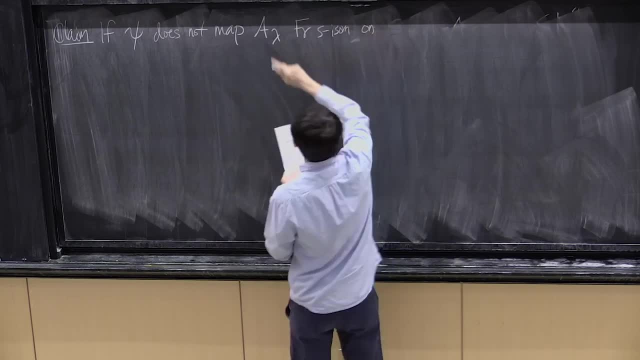 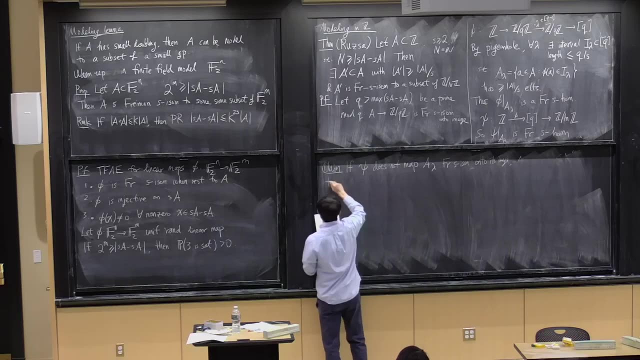 All right. so if it does not map A sub lambda Freiman-S isomorphically onto its image, then so what could have gone wrong? Claim that there must be some D which depends on lambda, in SA minus SA. 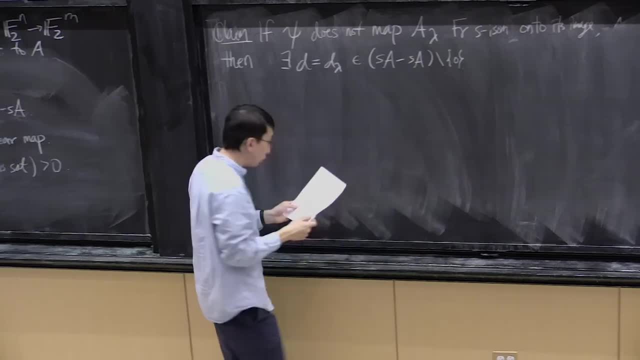 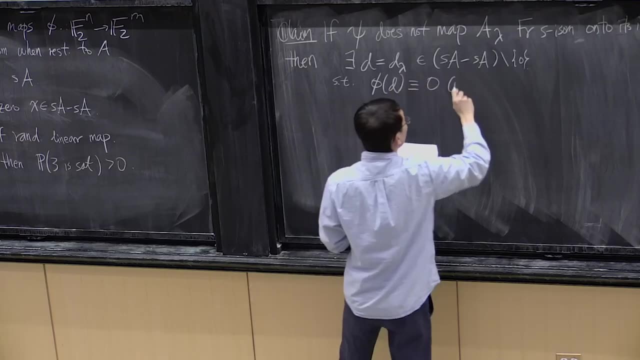 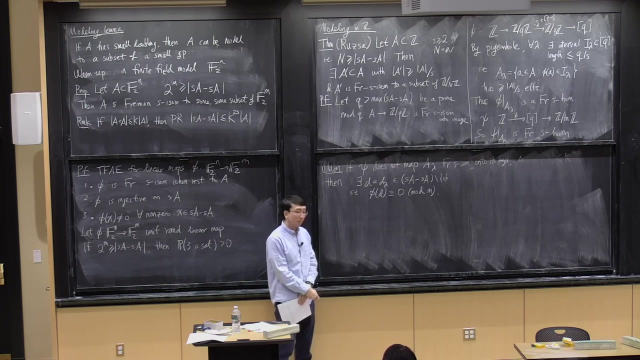 And D is not 0, such that the relationship between some D which depends on lambda and some D which depends on lambda, phi of d is 0 mod m. So we'll prove this, But, like before, it's a very similar idea. 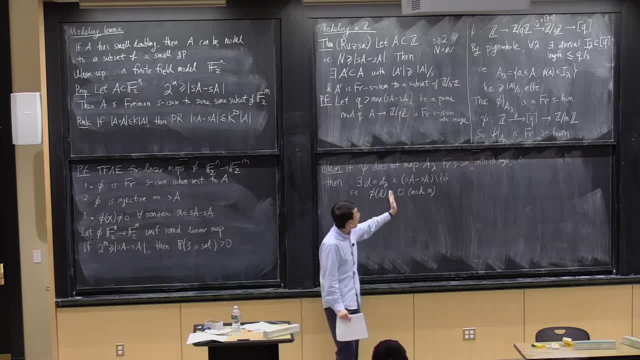 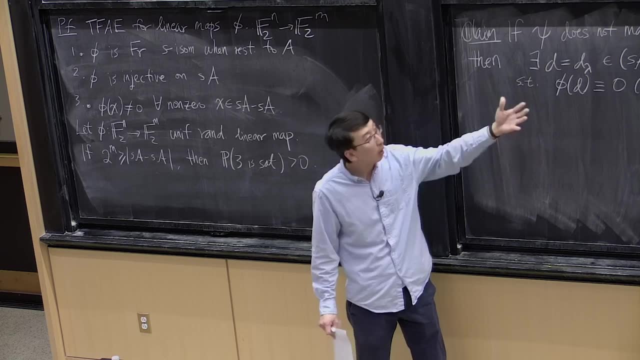 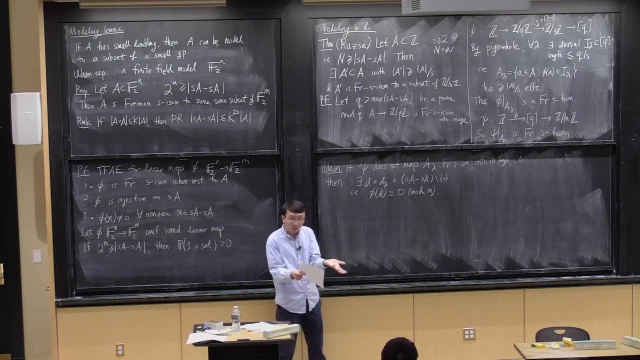 to what's happening earlier. The idea is that if you have- I mean we want to show that there are no additional additive relations in the image, So we would like to. so if it's not from isomorphism, then there has to be some accidental collisions. 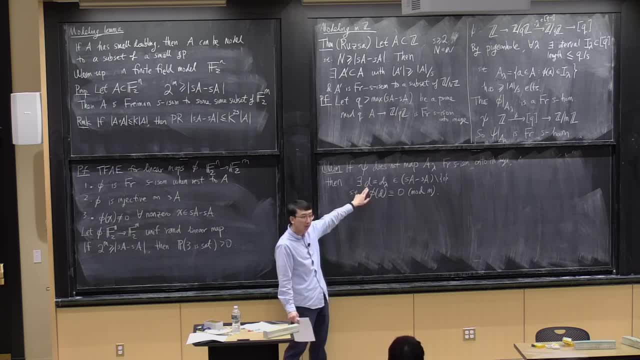 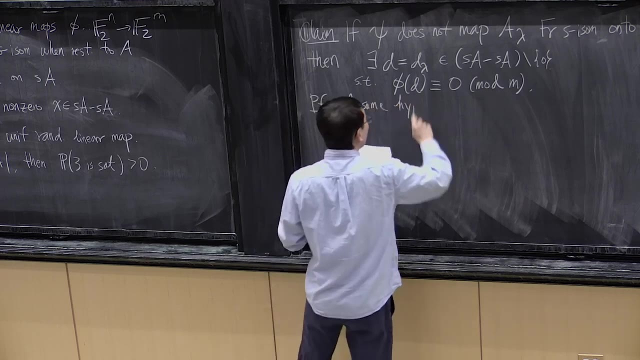 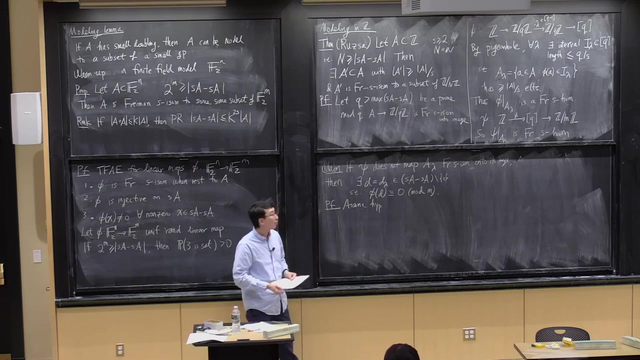 And that accidental collision has to be witnessed by some. d So this requires some checking. So suppose, indeed suppose the hypothesis, suppose that we suppose that the psi does not map a sub lambda from an s isomorphically onto its image. 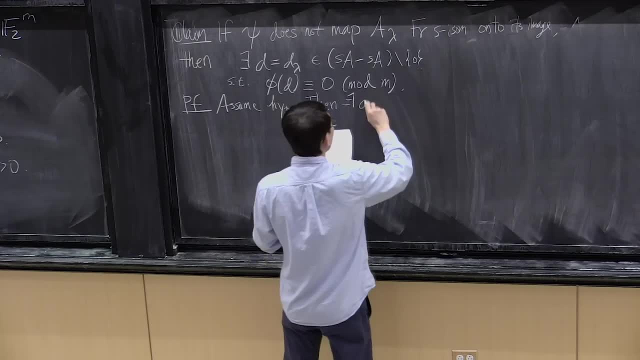 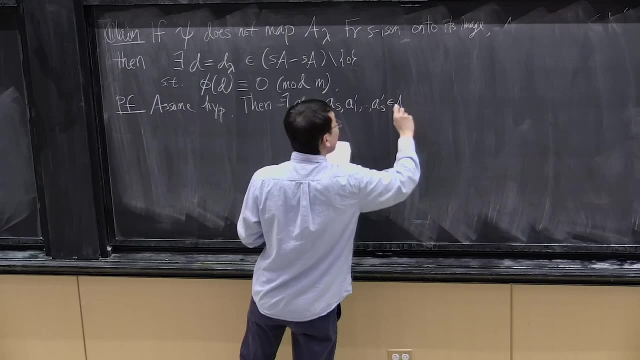 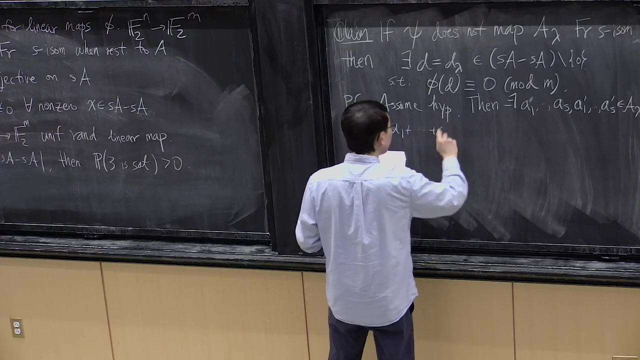 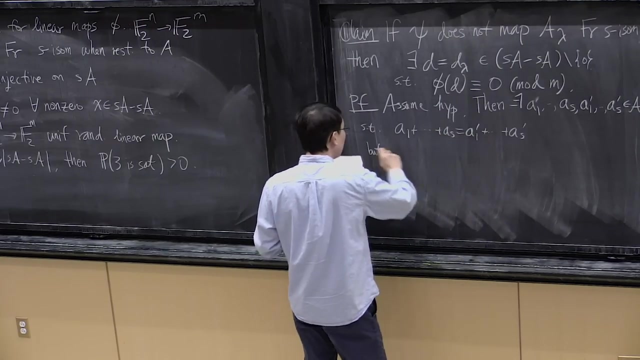 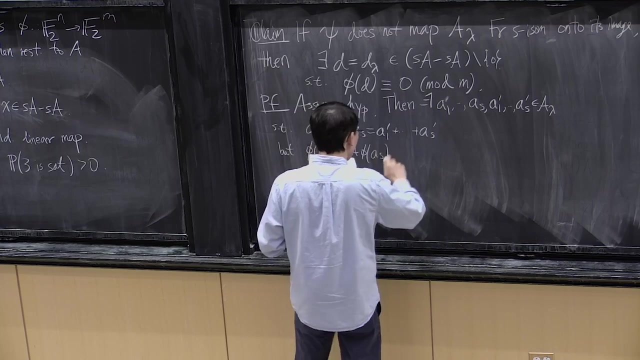 then there exists a1 through as a1, prime through as prime in a lambda, such that they do not have additive relation. but So their images do have this additive relation Now, their images all the way until the end. having the additive relation means 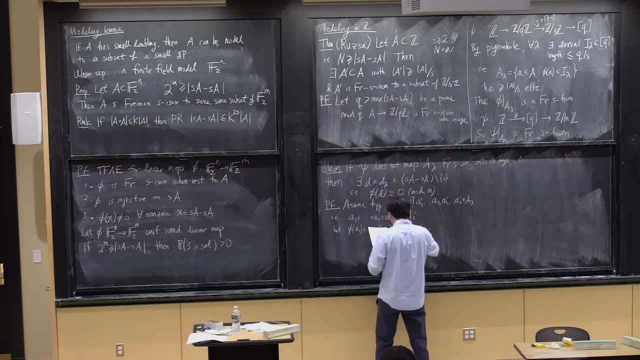 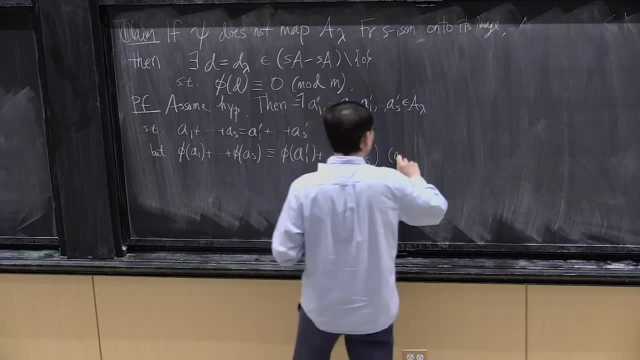 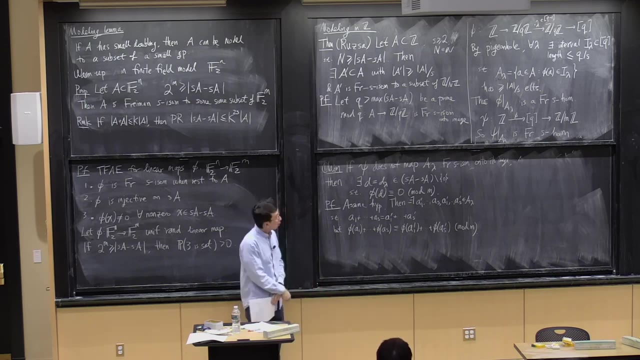 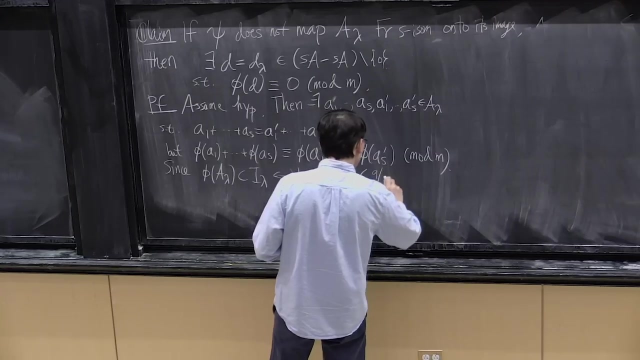 that phi has this additive relation, mod m. OK, So how can this be? Recall that, since the image, so all of these elements, lie inside some short interval, the interval has length less than q minus s. OK, So we saw this argument, a very similar argument. 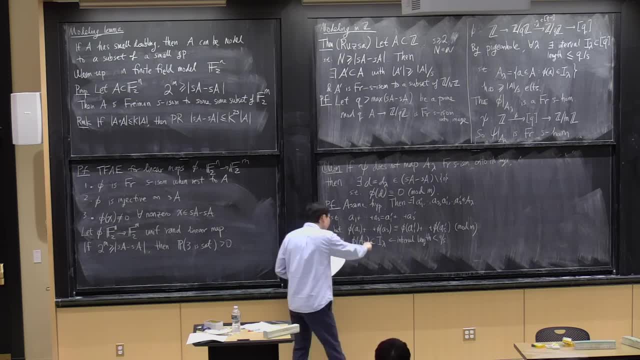 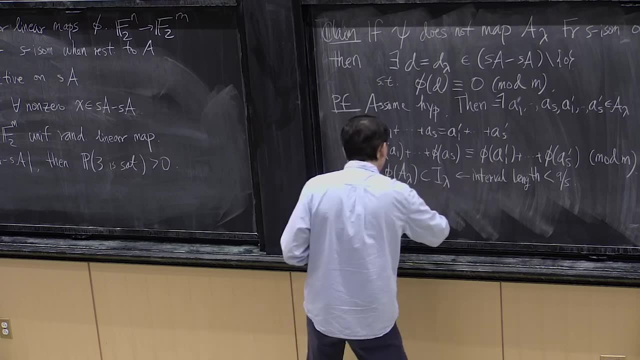 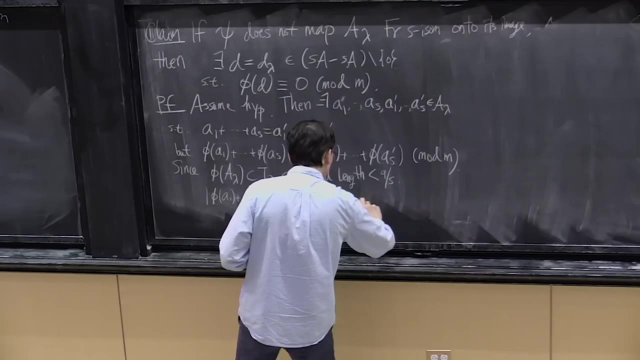 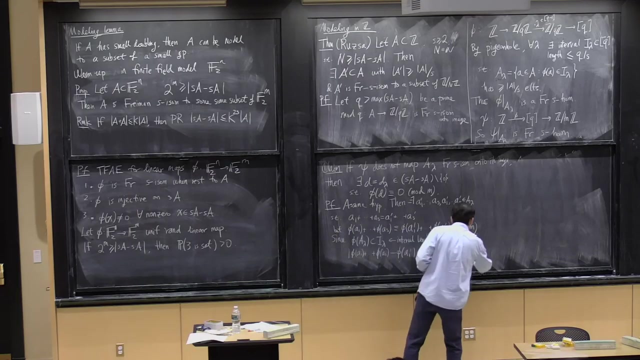 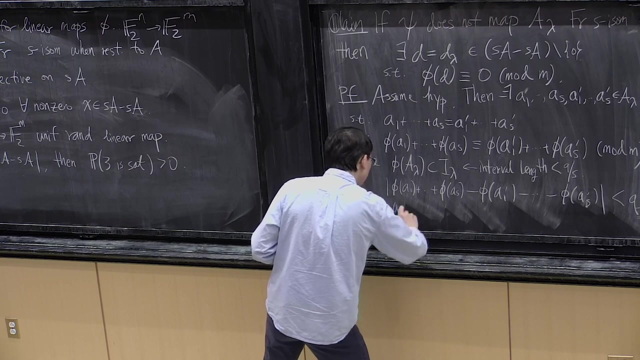 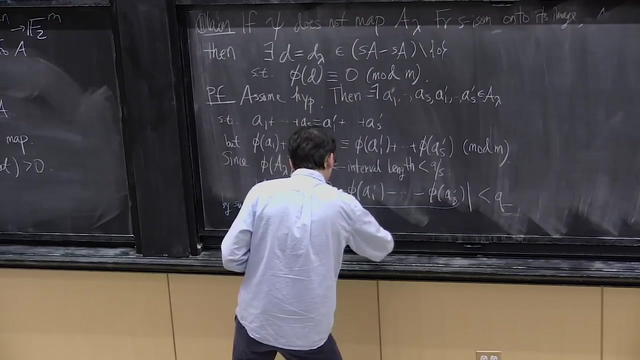 earlier before the break, Because everything lies in a short interval. we see that this difference between the left and the right-hand sides, this difference is strictly less than q. Now, by switching the a's and a primes if necessary, we may assume that this difference is non-negative. 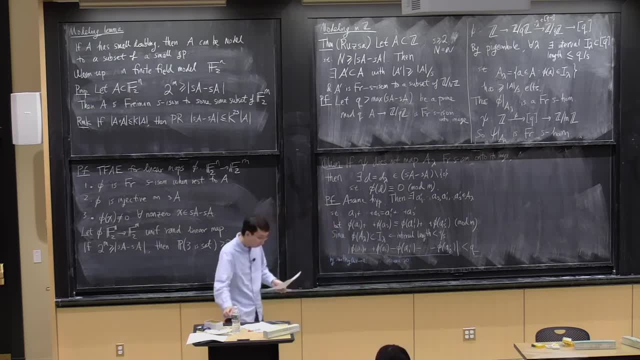 Otherwise it's just a labeling issue, Otherwise I relabel them. OK, So, So, So, So, So, So, So. then this here: so what's inside this expression? So let me call this expression inside the absolute value. 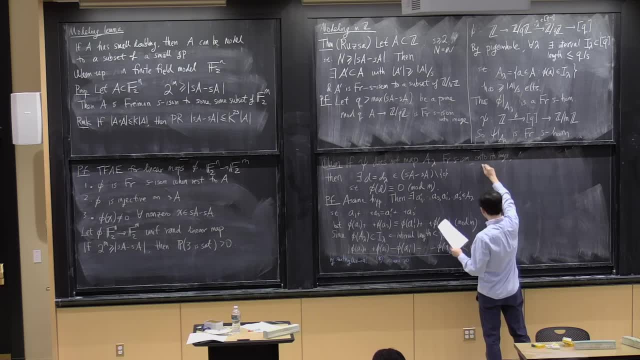 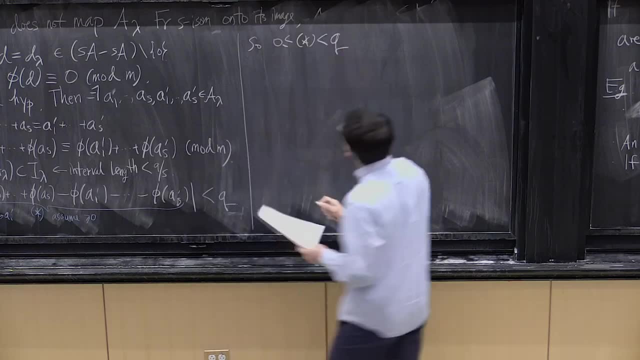 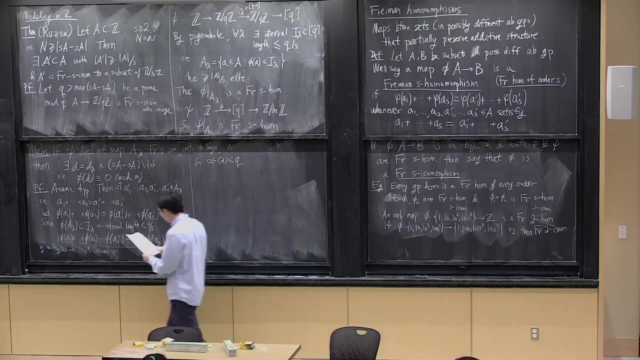 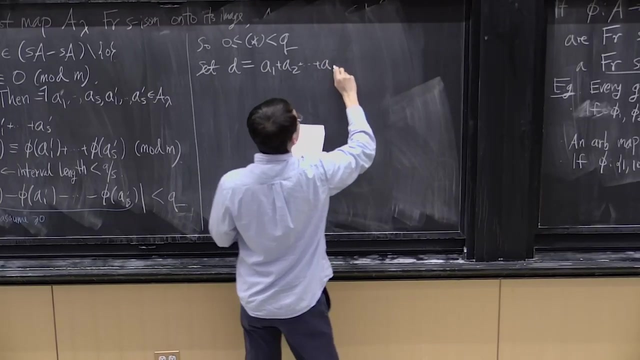 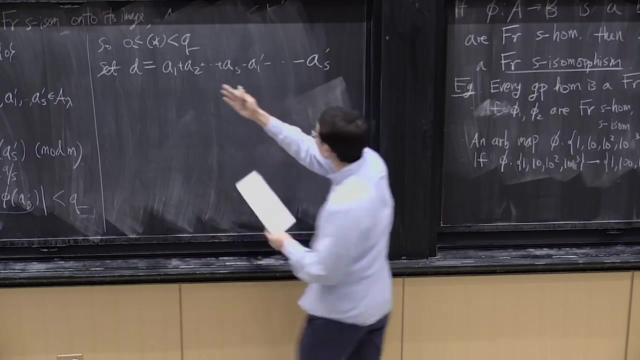 call it star. So then, so star is some number between 0 and strictly so at least 0 and strictly less than q. So if we set d to be OK, so d to be this expression. so sum up so the difference between these two sums. 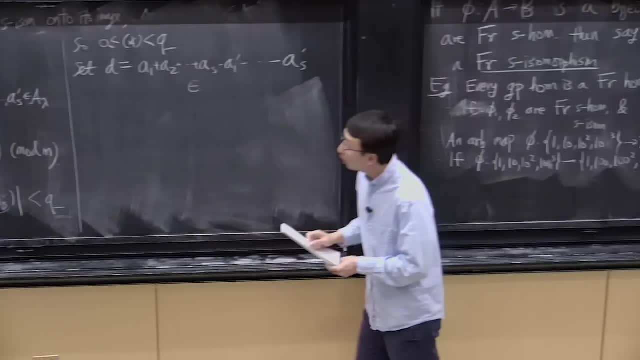 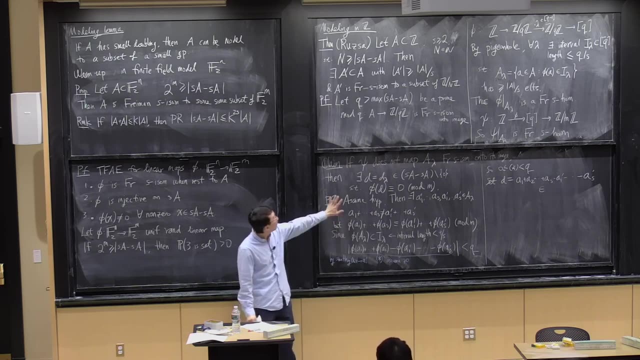 on one hand, this d here, So So this is a Sorry, That's what I want to say. Suppose you don't have an. OK, so if you are not mapping from and isomorphically onto the image, then I can exhibit some witness for that non-isomorphism. 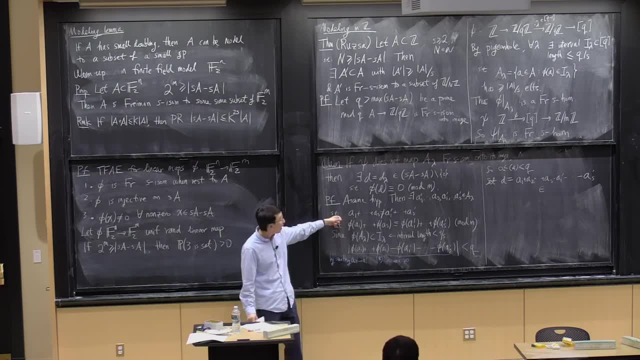 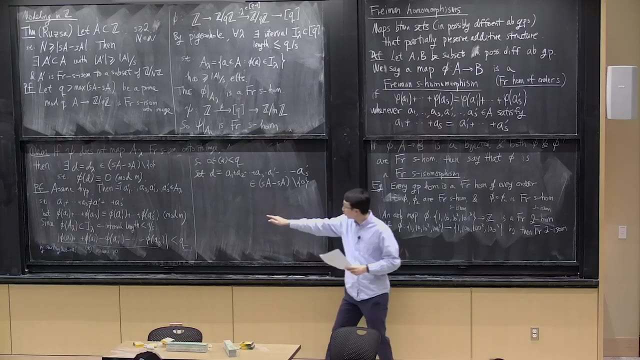 meaning a bunch of elements that do not have additive relations in the domain but that do have additive relation in the image. So if we set this d, then it's some element of SA minus SA And it's non-zero, because we assume that d is non-zero. 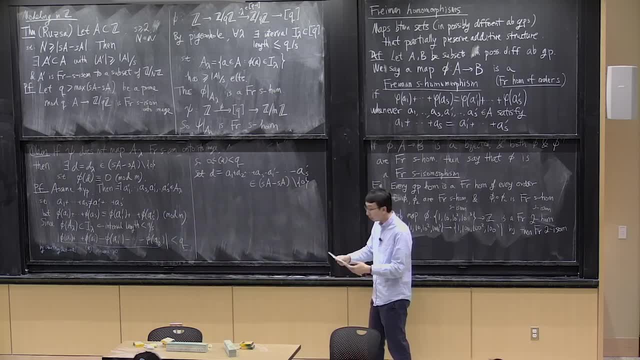 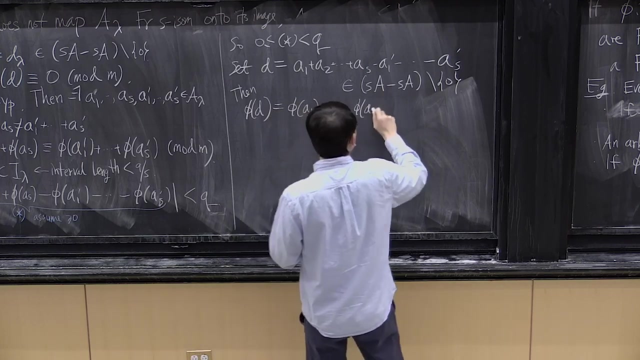 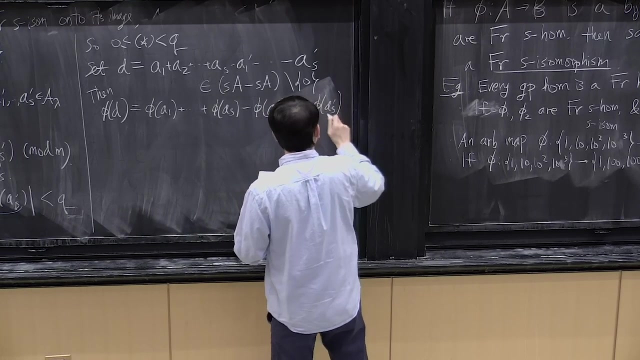 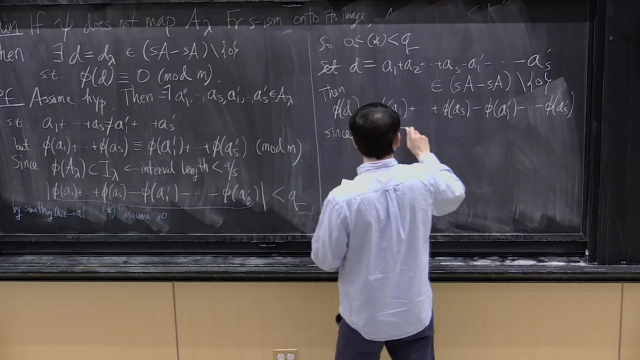 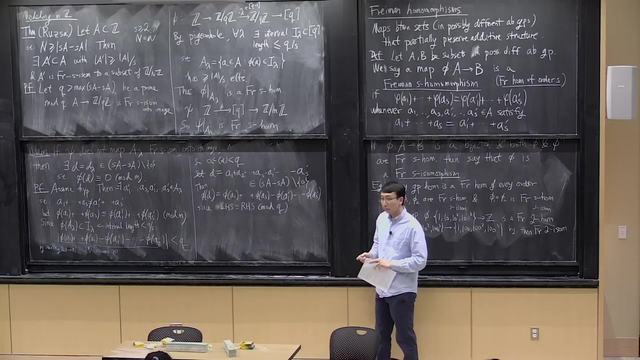 And so then, what can we say about phi of d? So phi of d, I claim must be, So this expression over here, the difference of the corresponding sums in the image, because the two sides are congruent, mod q. two sides are congruent, mod q. 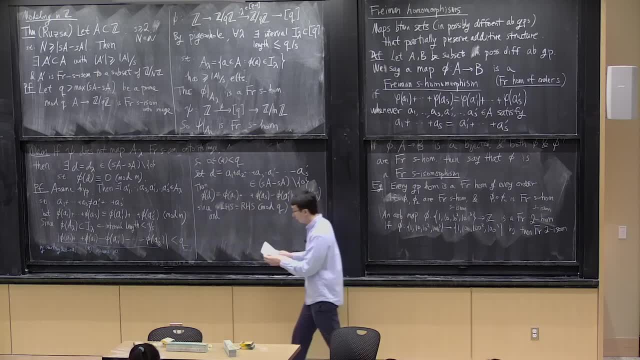 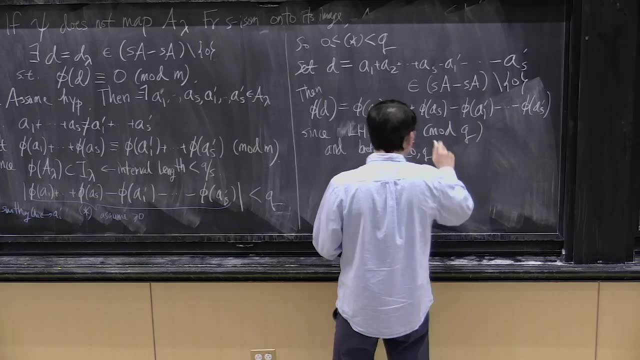 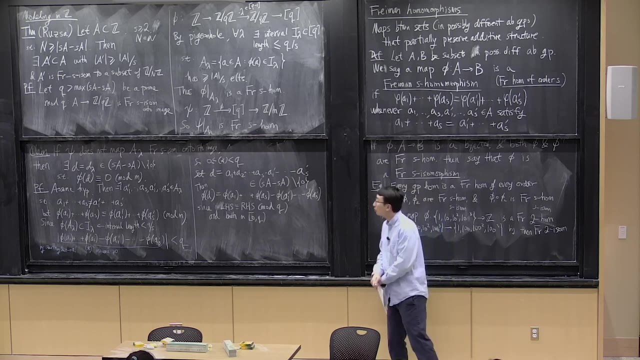 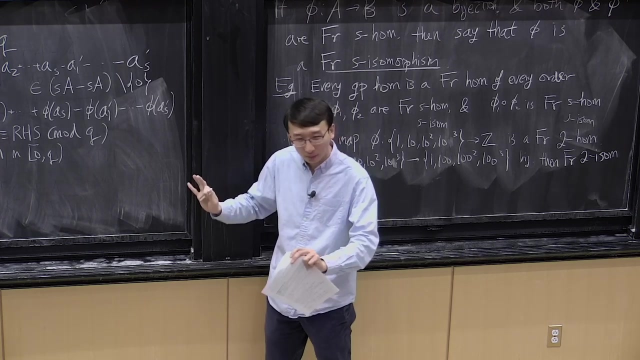 And Furthermore they are in the interval from 0 to strictly less than q. So this is a slightly subtle argument, But the ideas are all very simple. You just have to keep trying. You have to keep track of the relationships between what's. 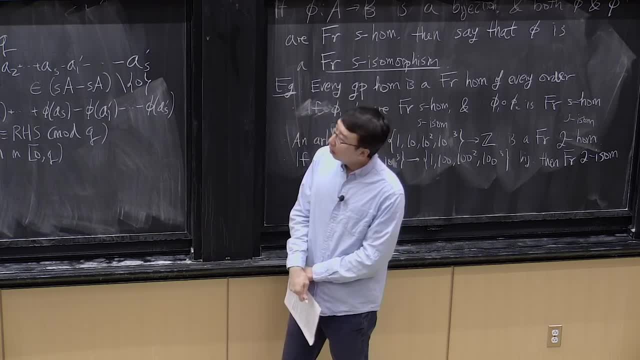 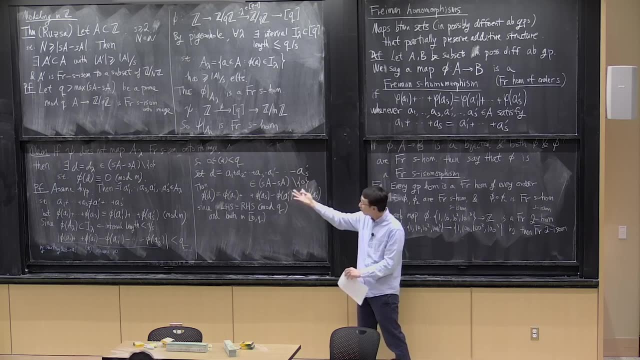 happening in the domain, what's happening in the image, But somehow I think the finite field case is quite illustrative of there. what goes wrong is similar to what goes wrong here, Except here you have to keep track of a bit more things. 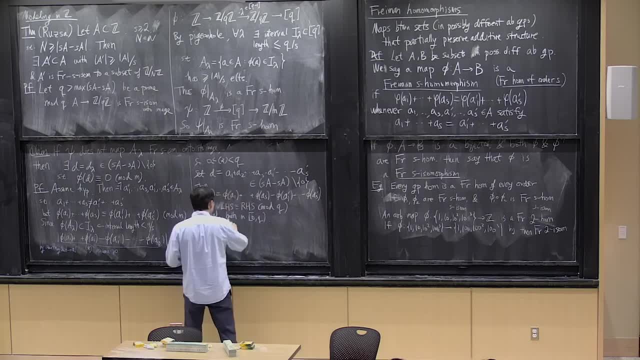 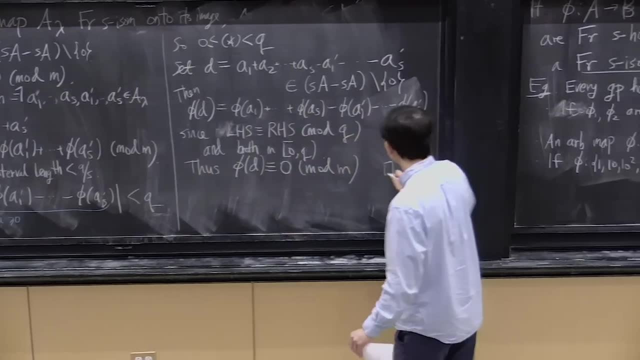 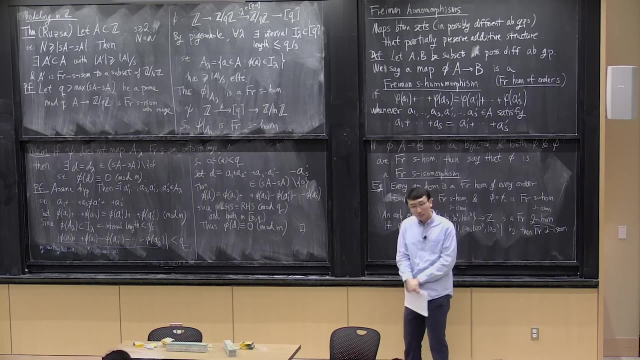 So consequently, thus, phi of d is congruent to 0 mod m, which is what we're looking for. So that proves the claim. Any questions? Yeah, OK, so this part. So we set d to be this expression. 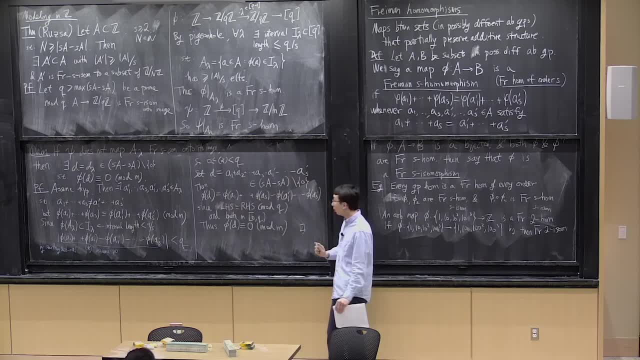 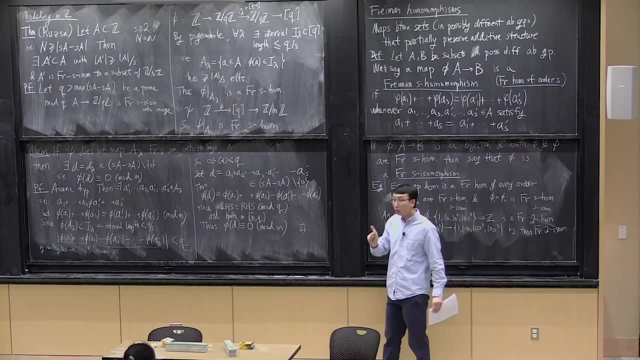 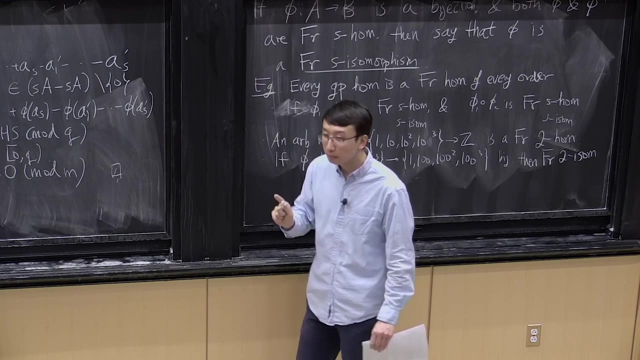 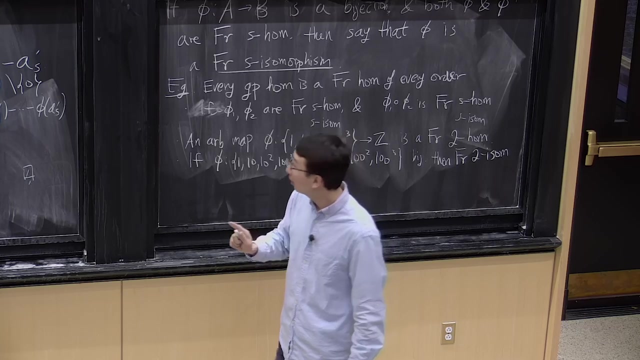 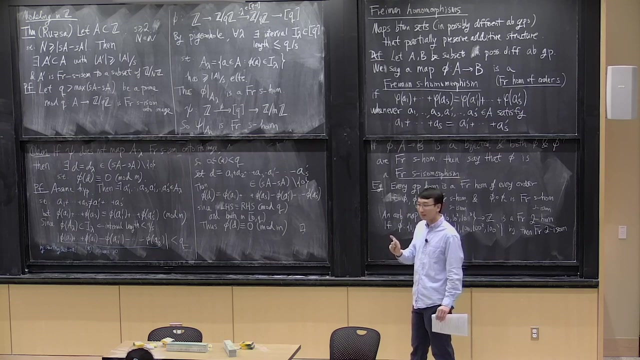 I claim this equality. So why is this true? First, the left-hand side And the right-hand side, they are congruent to each other, mod q. So why is that? Sorry Yeah, The first, every part of the prime. 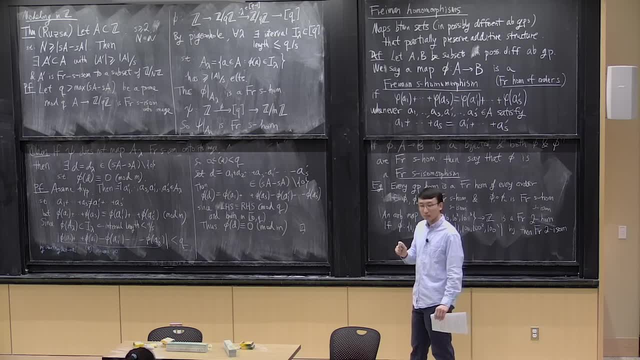 Yeah, So why should preserve? like the first two parts are group homomorphism, and then we just take things, mod q, Exactly, If you look at phi, where was it OK? so up there you see that everything preserves. 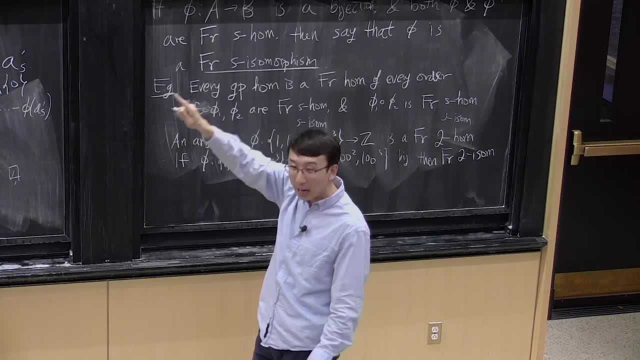 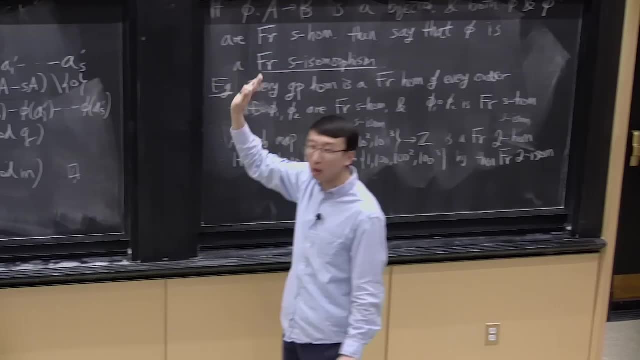 even though the very last step is not a group homomorphism, Mod q is preserved. So, even though the last step is not group homomorphism, it is so mod q. So if you're looking at mod q, everything is group homomorphism. 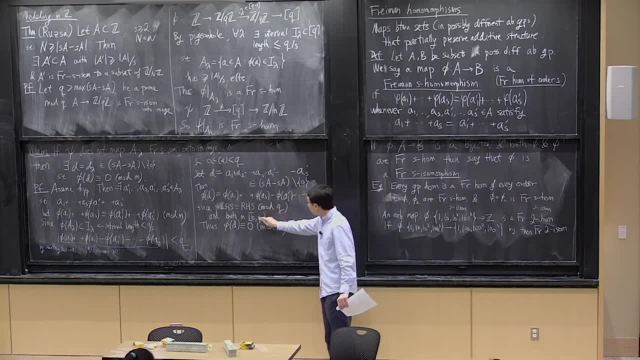 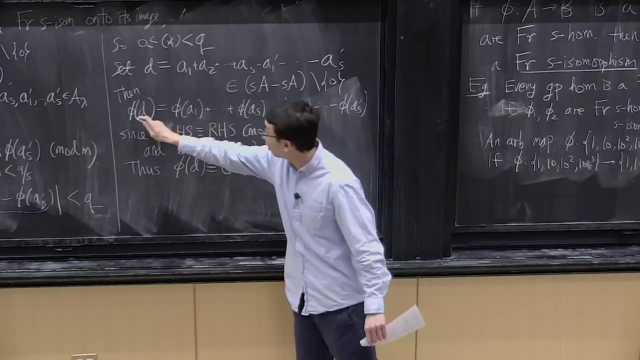 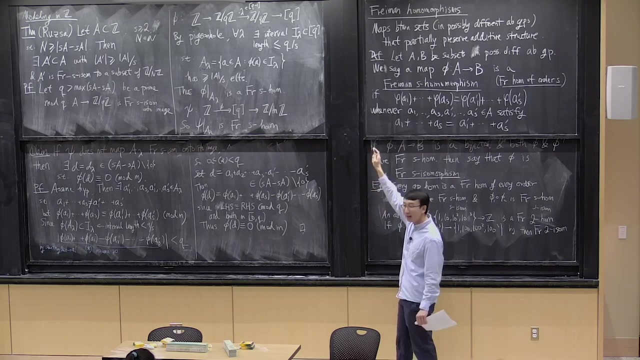 So here we're good. Both are in this interval. The right-hand side is in the interval because of our assumption about everything living inside a short interval, And the left-hand side is by definition, because the image of phi is in that interval especially. 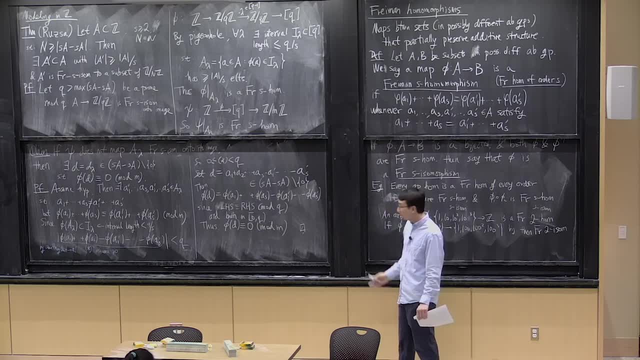 if, given that d is not equal to 0.. OK, is that OK? OK, yeah, so it's not hard, but it's a bit confusing, So you need to think about it. All right, so we're almost done. 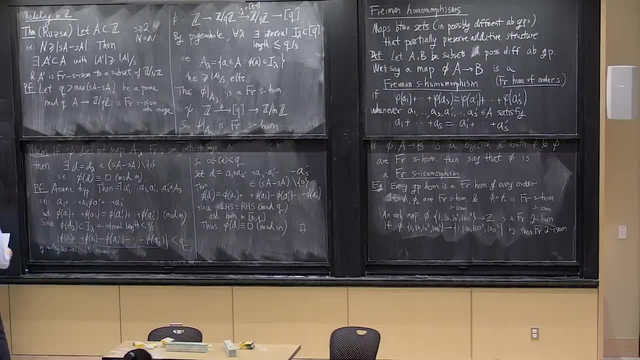 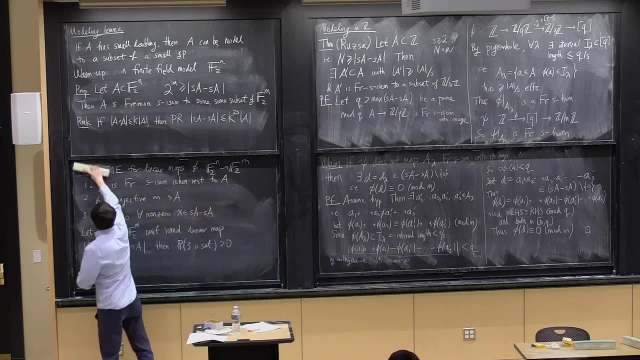 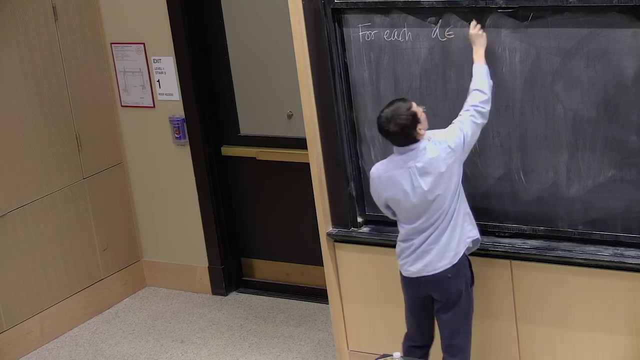 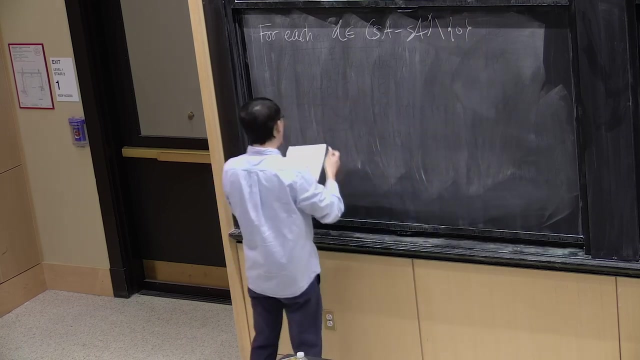 So we're almost done proving the Freiman to the Rucha modeling lemma in Z mod n. So let me finish off the proof. OK, so for each non-zero d in this iterated sum set, we would like to pick a lambda so that that map up there. 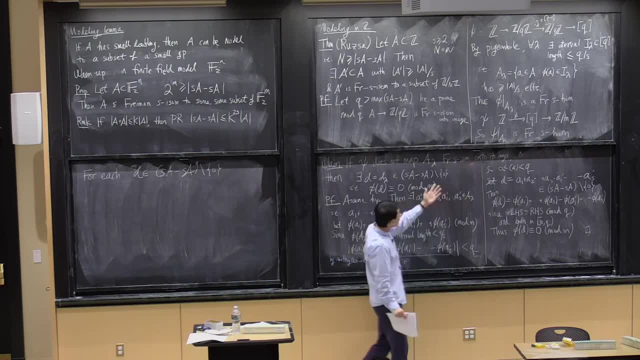 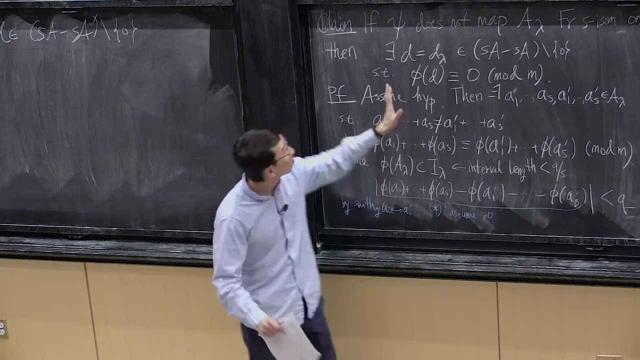 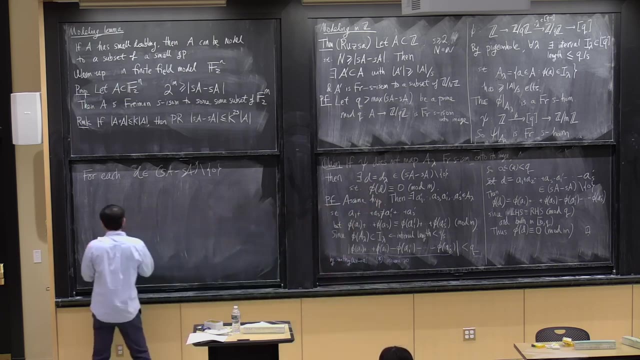 does what we want to do. If it doesn't do what we want to do, then it is witnessed by some d like this: OK, OK, Those are in the bad lambda. So if there exists such a d, then this lambda is bad. 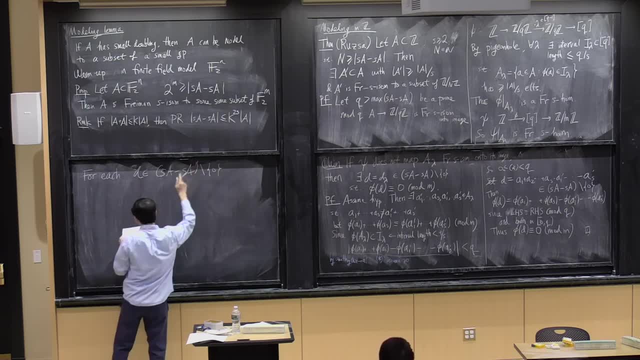 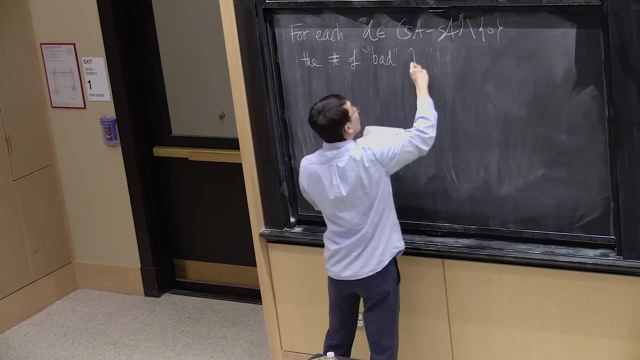 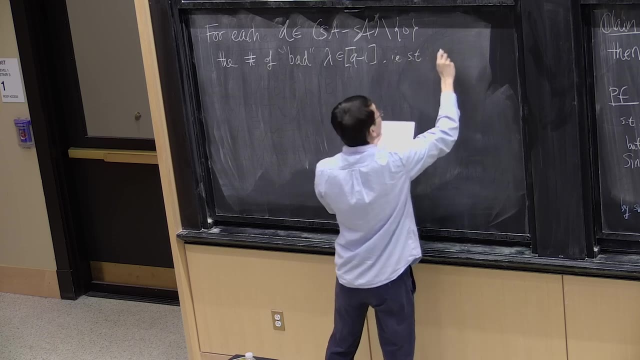 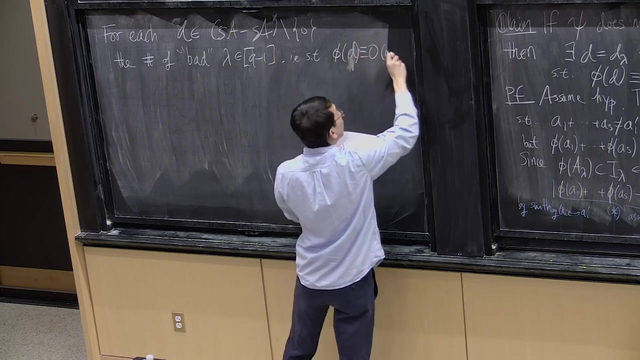 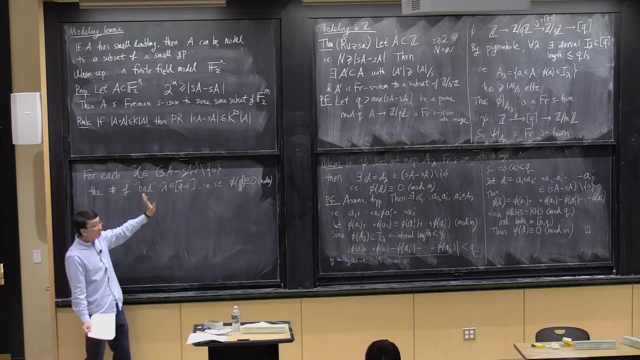 So for each d that potentially witnessed some bad lambda, the number of bad lambda so ie such that phi of q, phi of d, is congruent to 0 mod m. So here we're no longer even thinking about all the group. 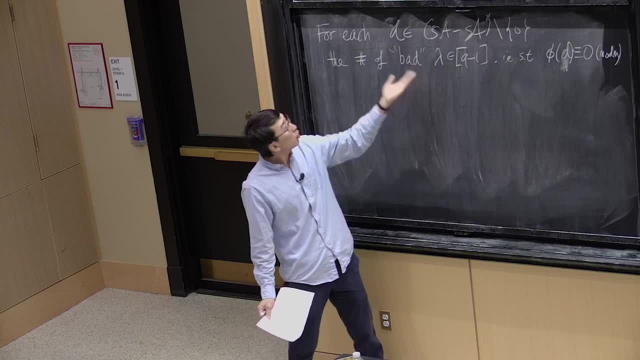 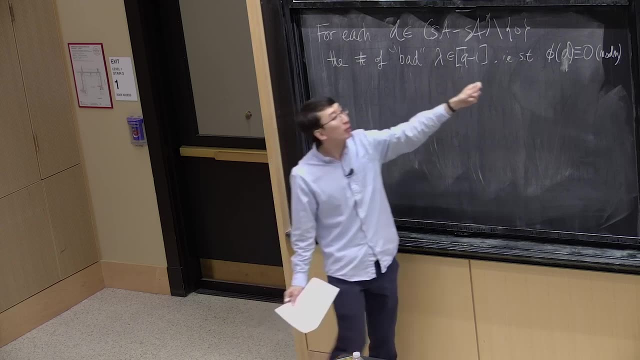 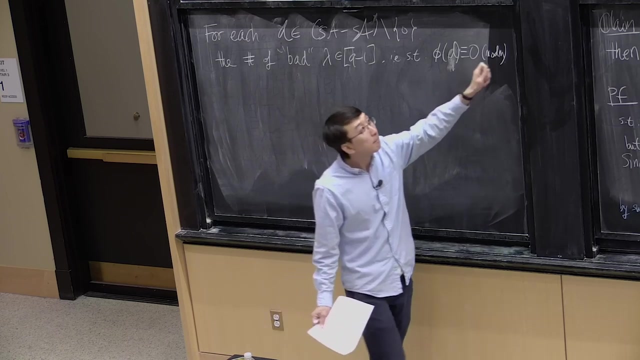 homomorphisms anymore, all the Freiman homomorphisms. Just the question: if I give you a non-zero integer, how many lambdas are there so that phi of d is divisible by m? OK, So remember that we pick q large enough so that initially, 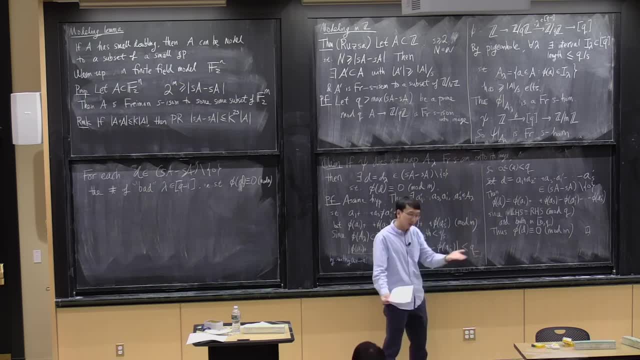 you are sitting very much inside this. everything's really between 0 and q, So this dot lambda up there acts uniformly. So the number of such bad lambdas is exactly the number of elements. OK, OK, OK, OK, OK, OK. 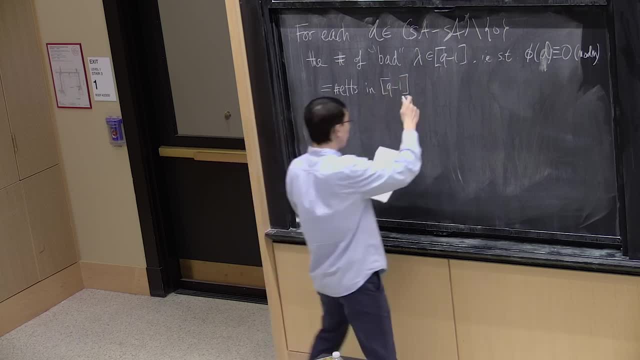 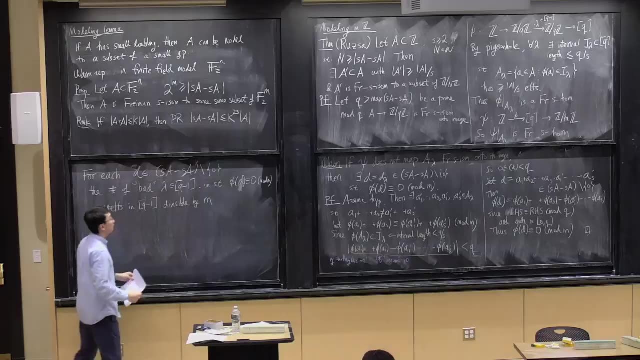 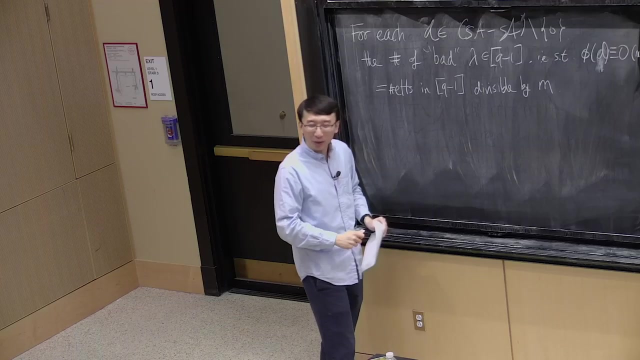 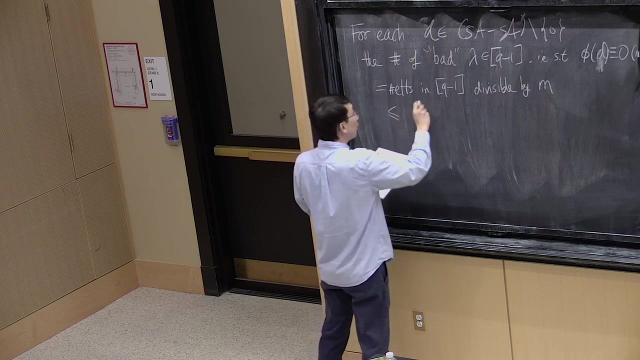 OK, So we have this interval that are divisible by m, So everything is more or less a bijection, if you restricted the right places, And the number of such elements is at most q minus 1 over m, So therefore The total number of bad lambdas is at most. 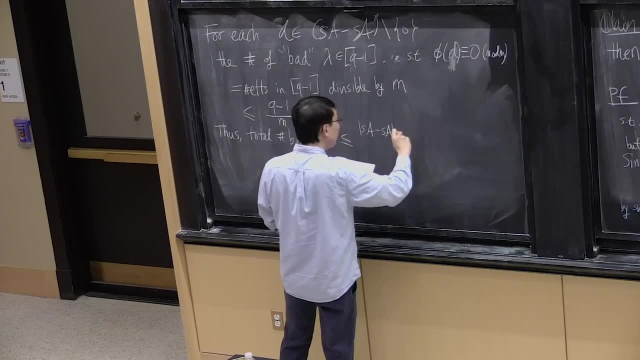 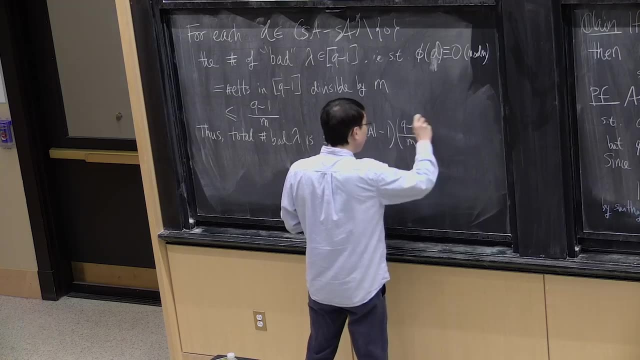 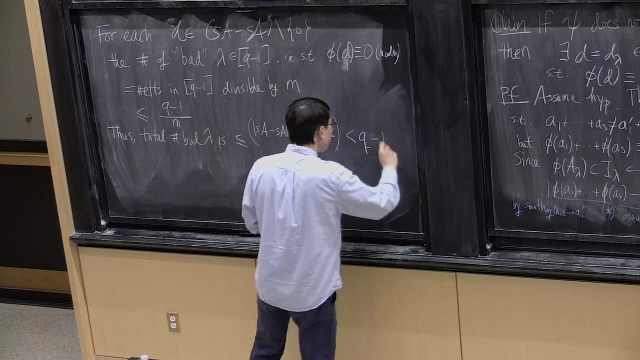 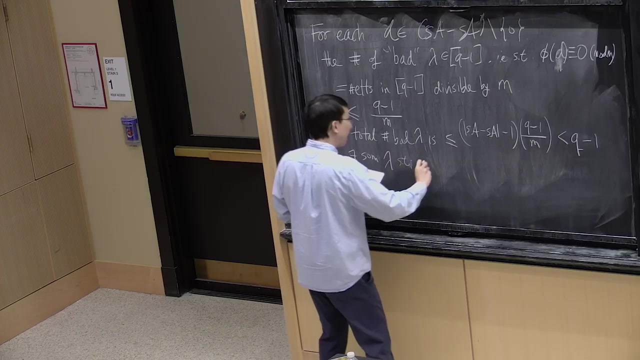 for each element d of sa minus sa, a non-zero element, we have at most q minus 1 over m bad lambdas. So the total number of bad lambdas is strictly less than q minus 1.. So there exists some lambda, such that psi. 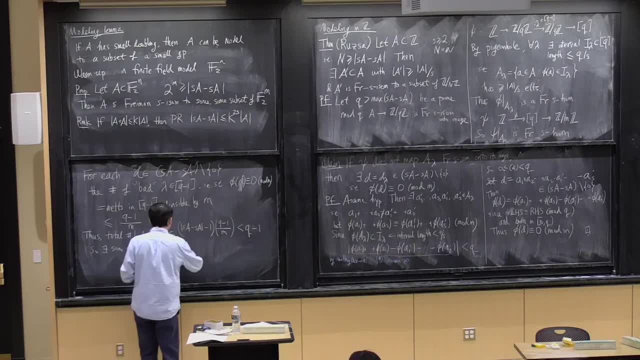 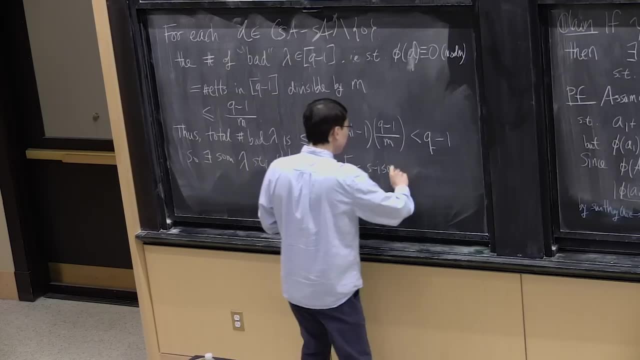 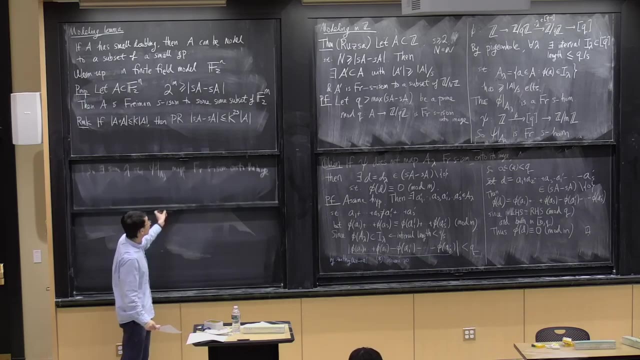 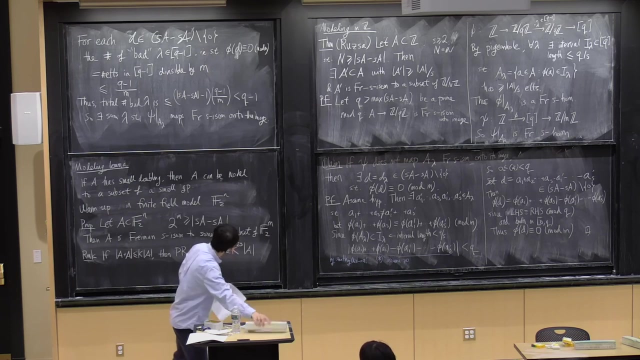 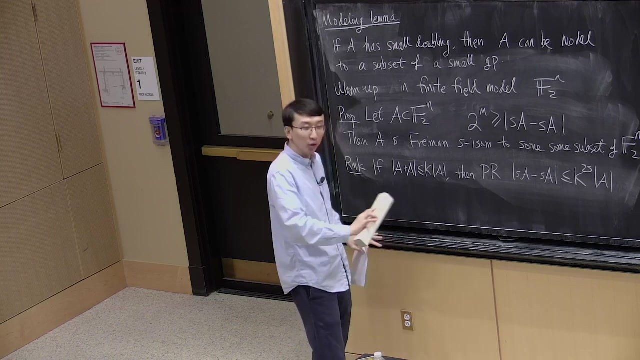 when restricted to a sub lambda, maps Freiman S isomorphically onto the image. Now, somehow I think it's really the same kind of proof as the one in the finite field case, except you have this extra wrinkle about restricting to short diameter intervals. 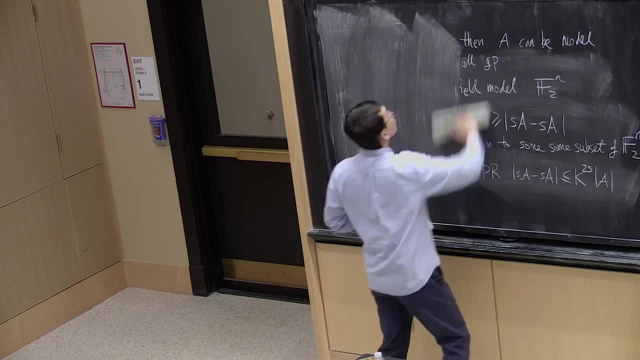 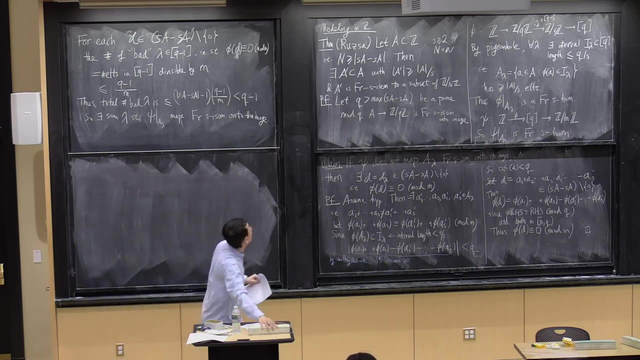 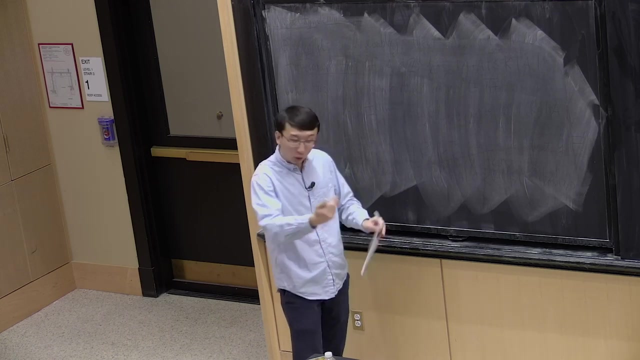 to short intervals, But the idea is very similar. So that's the Freiman model lemma in the integers, And let me summarize what we know so far so that I give you a sense of where we're going in the proof of Freiman's. 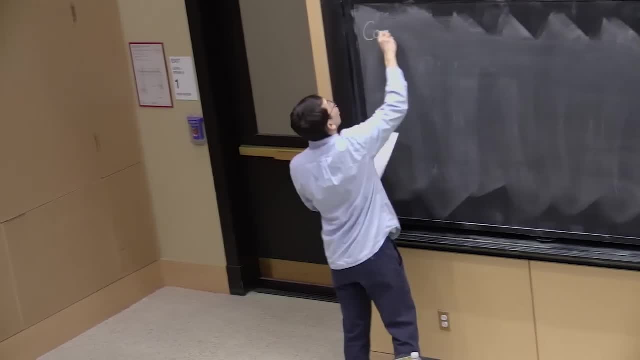 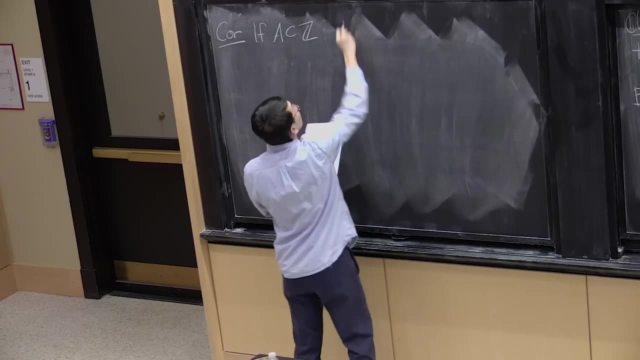 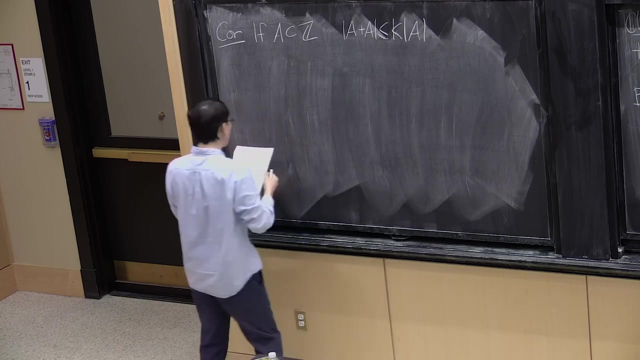 Thank you. Thank you, That's the Freiman's theorem. So what we know so far is that if you have a subset of integers, a finite subset, such that a plus a is size a times k, at most doubling constant at most k, then there 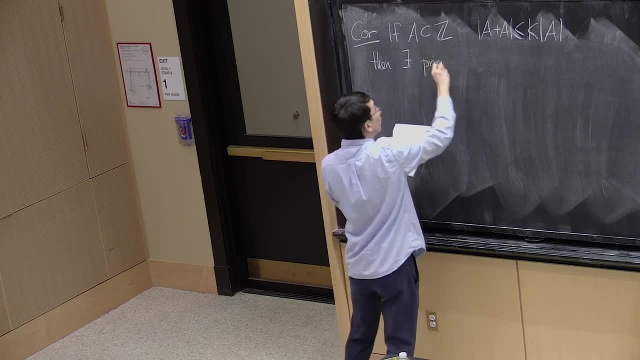 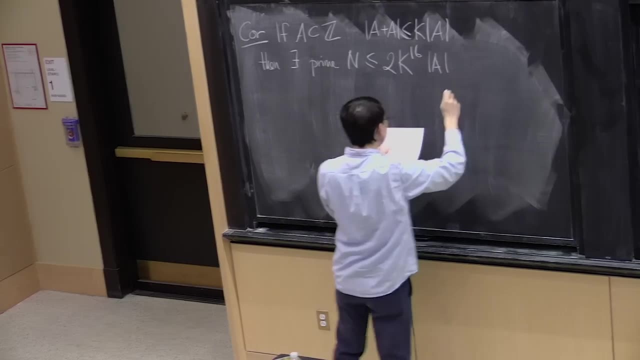 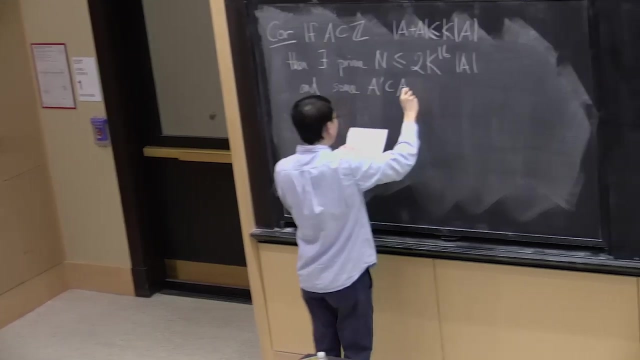 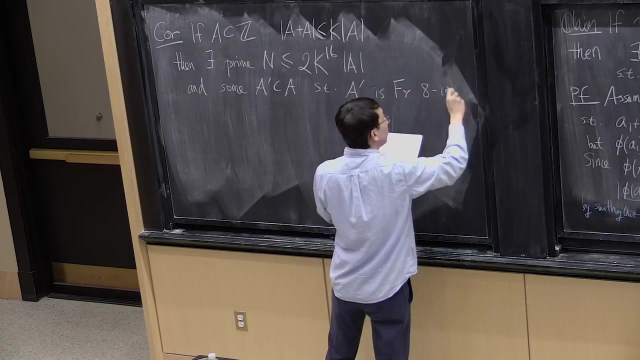 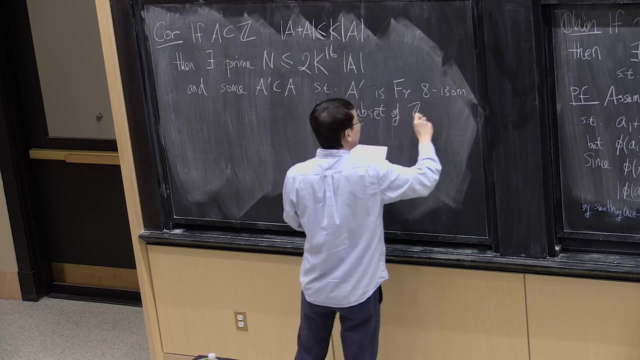 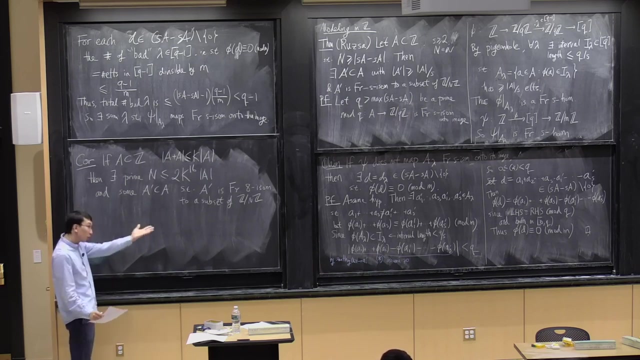 exists some prime n, at most 2k to the 16th times times the size of A, and some subset A prime of A such that A prime is Freiman A, isomorphic to a subset of Z mod nz. So it follows from two things we've 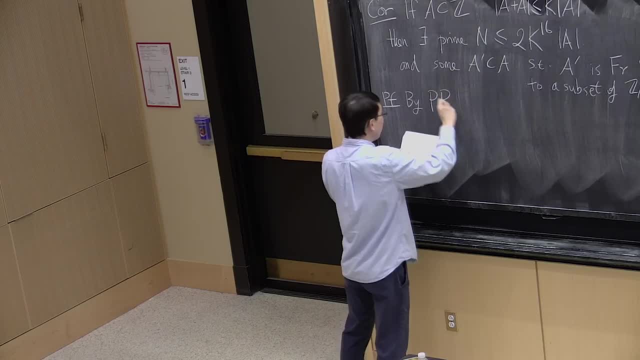 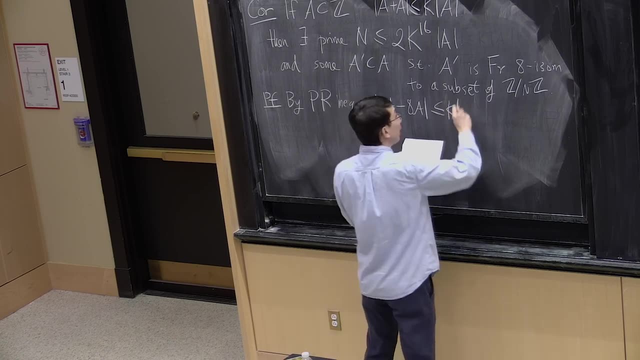 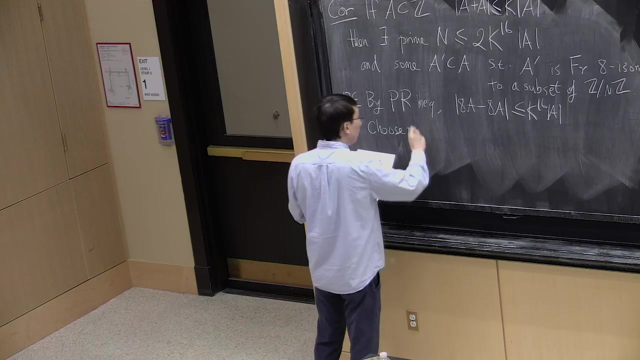 seen so far, because by the Plunnecker-Ruzsa inequality 8A minus 8A is at most k to the 16 times A, And now we can choose a prime n between k to the 16 and 8.. 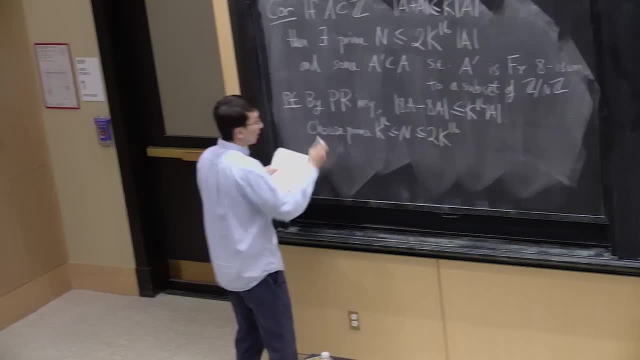 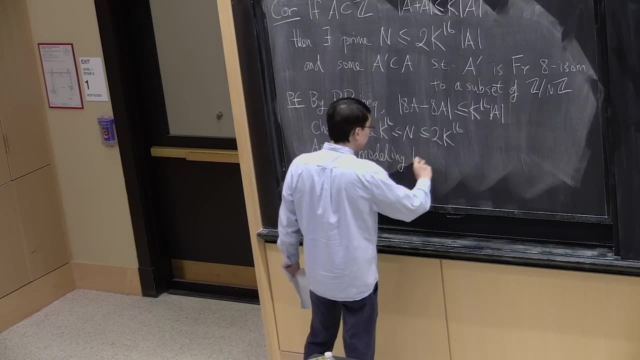 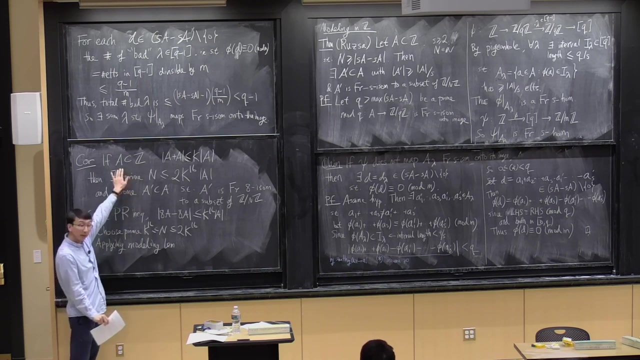 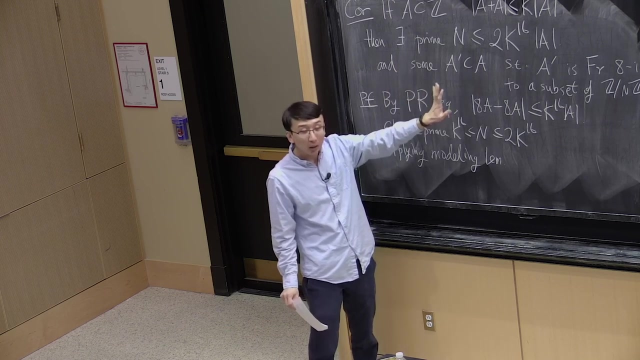 2 times k to the 16, and apply the modeling lemma. So that's where we are at. So you start with a set of integers with small doubling. Then we can conclude that by keeping a large fraction of A, keeping no. 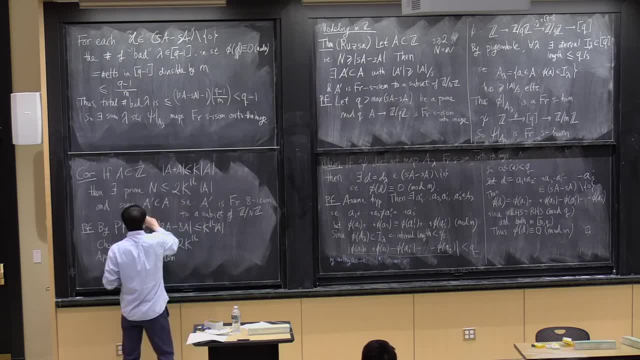 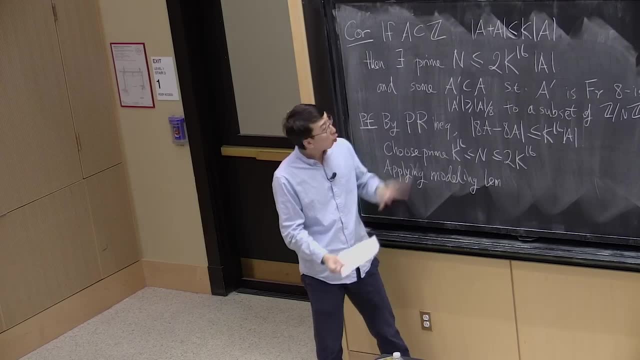 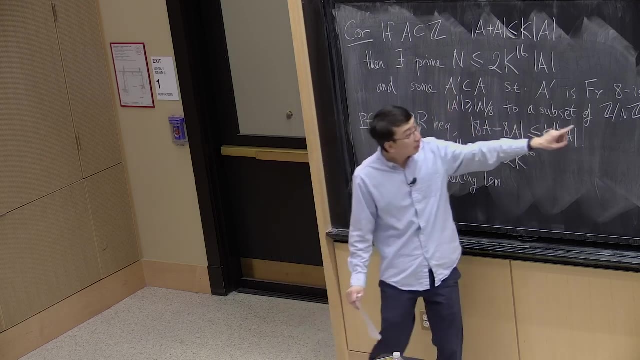 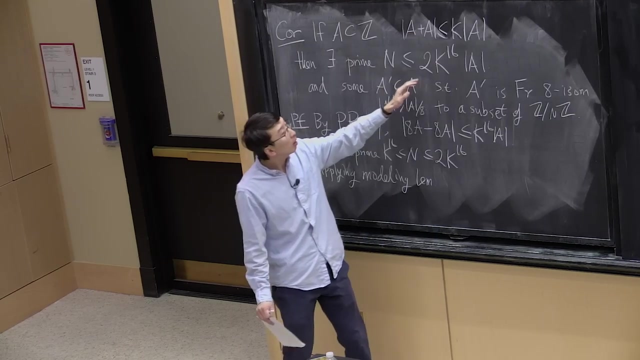 First We've got to OK, so very important. So there exists some A which is a large fraction, So keeping a large fraction of A. I can model this large subset of A by some subset of a cyclic group where the size of the cyclic group is only a constant times. 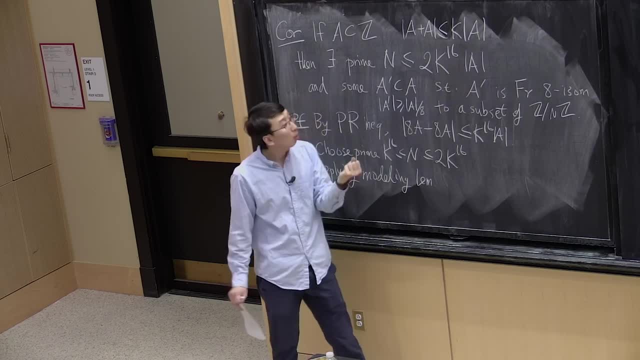 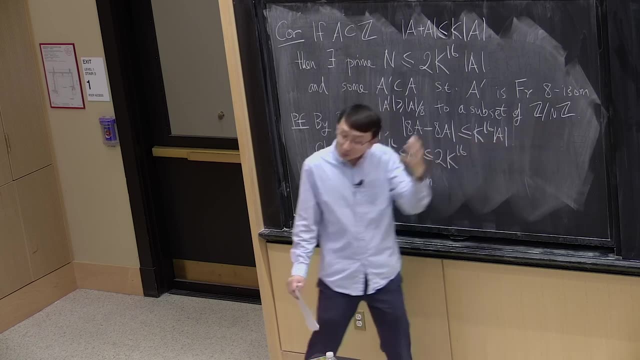 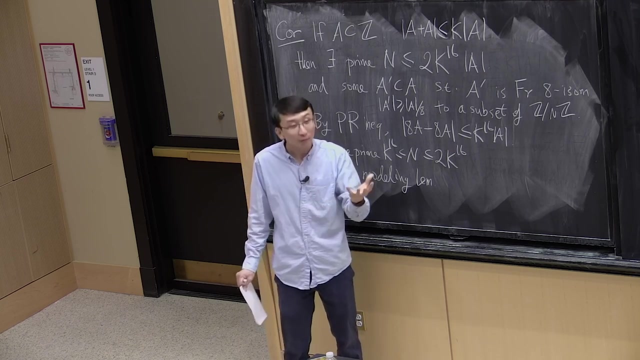 more than the size of A. So now, OK, So we are going to work inside a cyclic group And working with a set inside a cyclic group. that's a constant size, a constant fraction of the cyclic group. Why 8?? 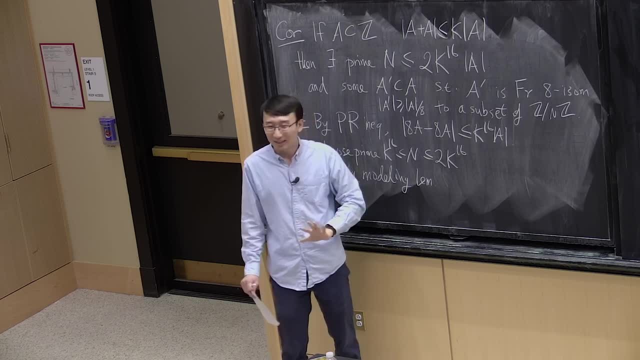 YUFEI ZHAO- Question is: why 8?? So that will come up later. So, basically, you need to choose some numbers so that you want to preserve the structure of GAPs. So that will come up later. And now we're inside a cyclic group.